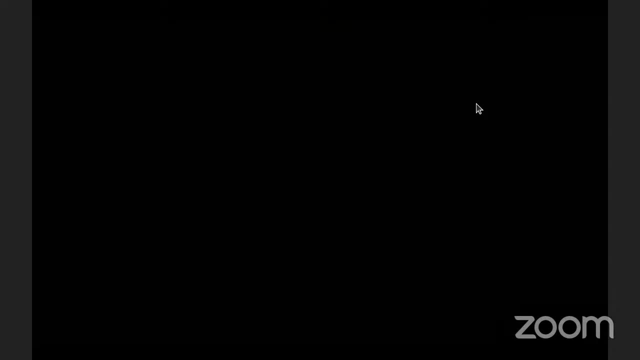 And subsequently, I think, you became an associate professor at Oxford. So you've been at Oxford for a long time now. David has worked on many things in cosmology from CMB and still works on many things in cosmology from CMB to galaxy clustering, to weak glancing, to 21 centimeter surveys as well. So he's like really impressive the amount of different topics and the amount of work that he does. 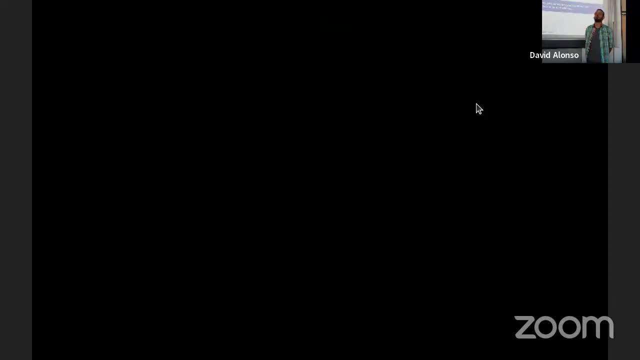 Everybody I talked to that has collaborated with David always can Great opinions, And we're always impressed by the amount of work you do and the kindness you have. So it's really I can confirm this, And so today David will tell us about cosmology from projected large scale structure. And so please take it away. 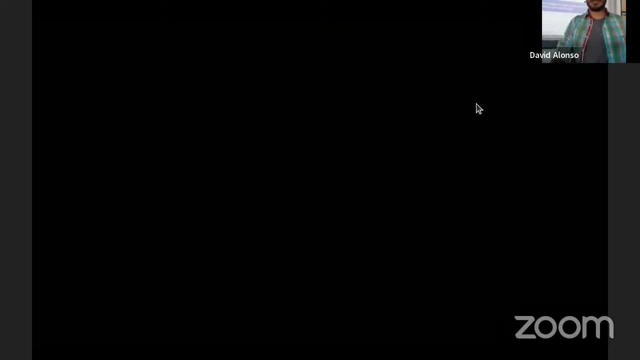 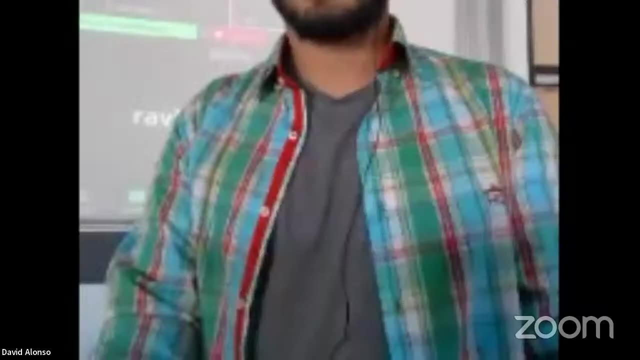 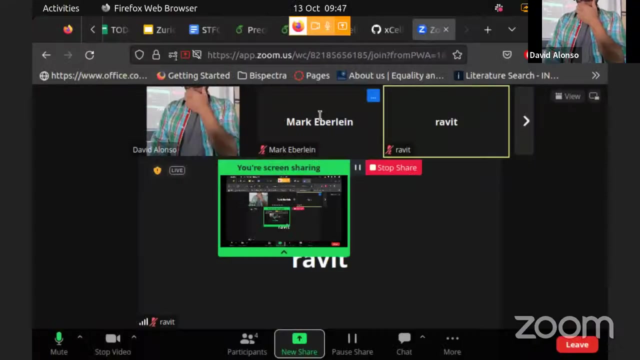 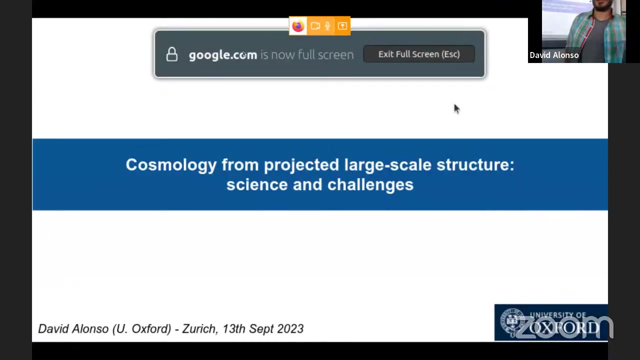 Okay, thanks a lot, Andrei. What do you want me to do? Stop sharing, Okay, Let's see. Stop sharing And then share again. Okay, How's that? Yep, Yep, Okay, cool. Well, thanks a lot, Andrei and everyone for the invitation. I'm really sorry I couldn't make it last time. I got the flu and then there was a strike at the airport, So it would have been a nightmare. 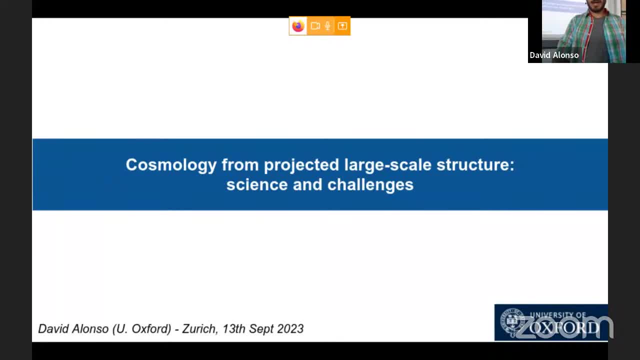 But yeah, I'm really happy to be here. It's the first time I'm actually in Zurich for academic reasons. This is quite exciting. Yes, I'm going to be talking about projected large scale structure, And by projected what I mean is that all of the probes that I'm going to be talking about are just things that are defined on the sphere rather than in three dimensions. 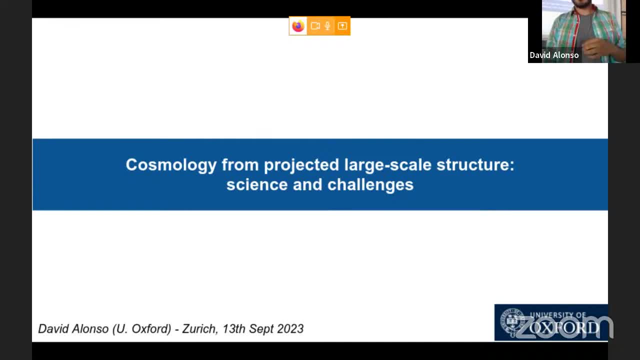 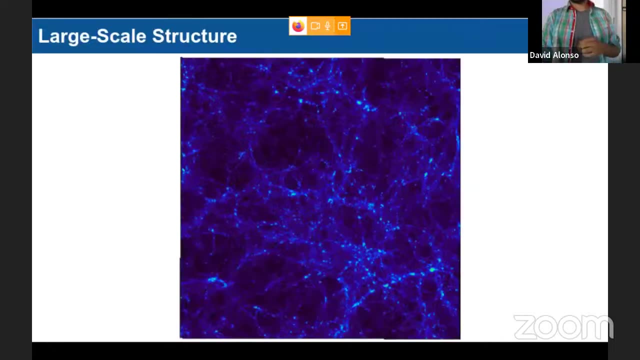 That's all. It's just to dispel any expectation that I'm going to talk about spectroscopic surveys, because I'm probably not. So let's look at some of the tracers, the probes that we have of the large scale structure, And we're talking about projected tracers. 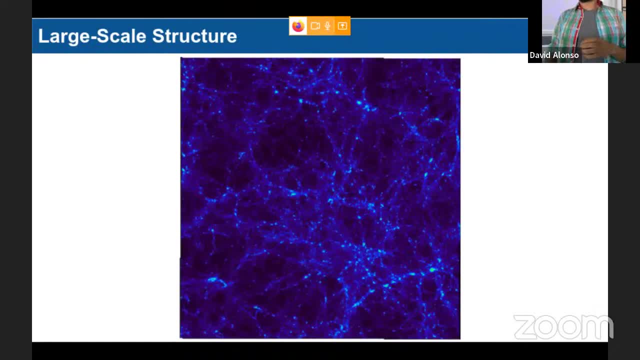 One of the main ones that come to mind is the photometric ratchet survey. Ultimately, what we care about is trying to extract constraints on fundamental parameters from the distribution of matter fluctuations in the universe. But we are not able to observe these directly, So we need to observe these through proxies of these matter fluctuations. 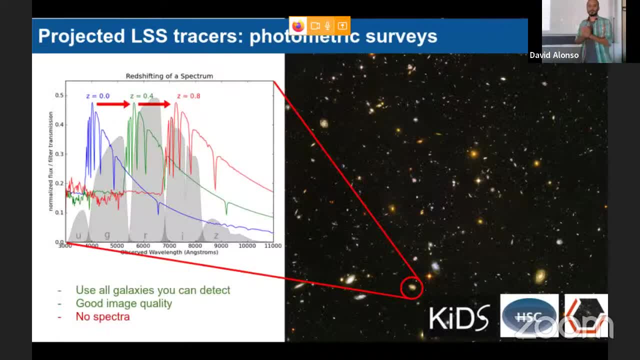 And in photometric surveys. we have several of these. For those who don't know what a photometric survey is, just a very quick introduction. in a photometric survey, it's a survey where, basically, you image as much of the sky as you can, as deep as possible, and you try to observe as many galaxies as possible. 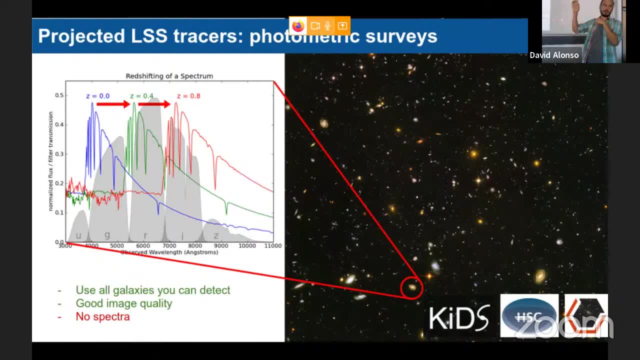 And for those galaxies. instead of trying to extract the spectrum of each galaxy, because that would take a long time, you just get the overall flux in a small number of bands. From that you try to extract what the ratchet of the galaxy is, to see where to put it. 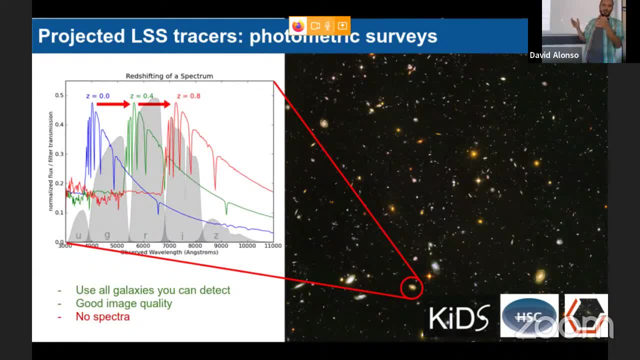 Put it in the radial direction, But you're always going to have a very crappy estimate of the ratchet. So in practice you don't really know very well where galaxies are. in the radial direction. You need to mostly rely on the angular distribution, angular properties of these galaxies. 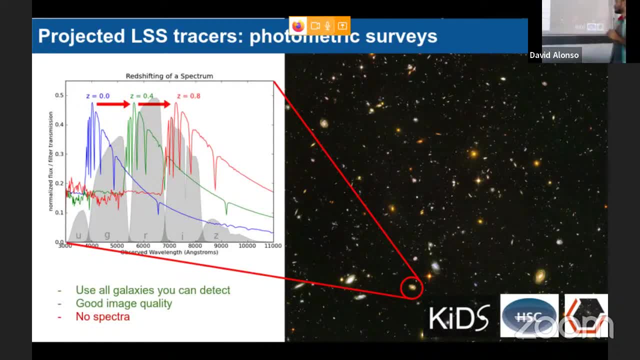 Photometric, but the advantage is that you have lots of them. So photometric surveys have become very important for cosmology in the last, I would say, 20 years, particularly the last five to 10 years, with experiments like KITS, HSC and the Dark Energy Survey, particularly in the context of weak lensing, which I'll talk about later. 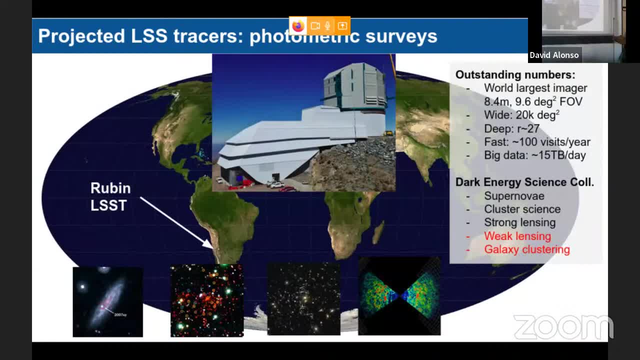 The next generation of these surveys is going to be the Vera Rubin Observatory, the LSST, which is one of the experiments I'm involved in. So I just wanted to show one of the pictures of that. So that's going to be. you know, it's going to go beyond any of these surveys in both area- depth and number of objects. that it will do. 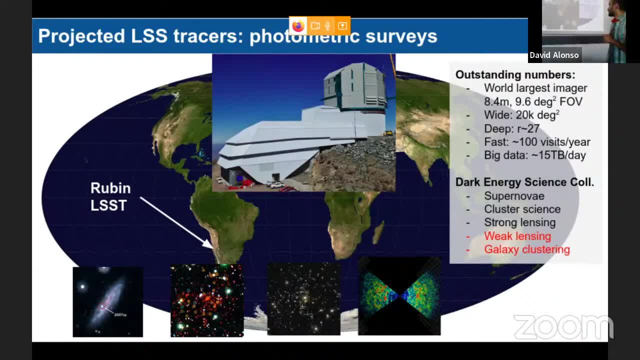 that it will observe, It will do cosmology using five different probes, which are listed here, And of those I'm going to be focusing on the two projected traces of the last structure: weak lensing and galaxy clustering. So let's dive into those. 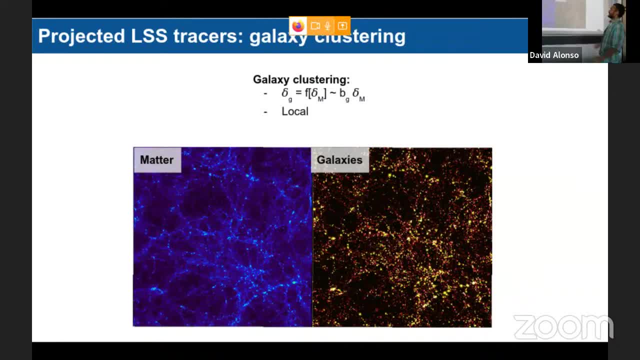 So first, galaxy clustering. So the idea in galaxy clustering is the proxy that we use to trace the matter: fluctuations, if you have, the distribution of galaxies, the idea being that where there's more matter there should be more galaxies, The actual detailed relationship between the matter. 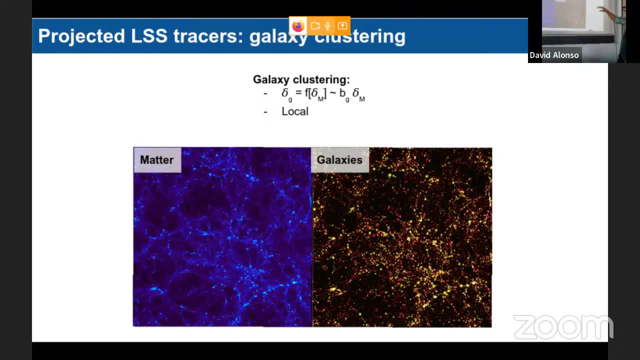 fluctuations and the galaxy density fluctuations is very complicated. We know that it's probably nonlinear, non-local and stochastic, But on sufficiently large scales there's good reasons to expect that the relation between the two of them should be linear, with an unknown linear proportionality constant which 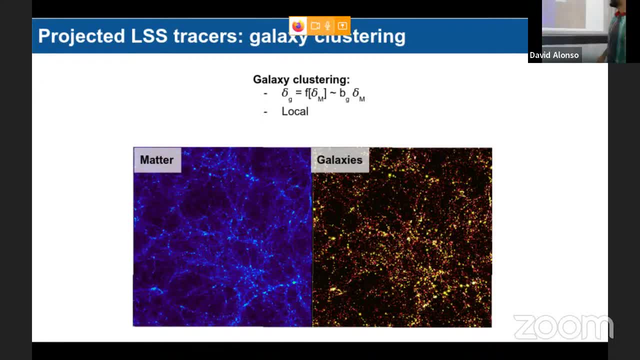 is what we call the galaxy bias, that BG over there. And the other important aspect of galaxy clustering that one must know Very mind is that it's a local tracer of the matter- fluctuations- which means that if you're observing galaxies at the given redshift, 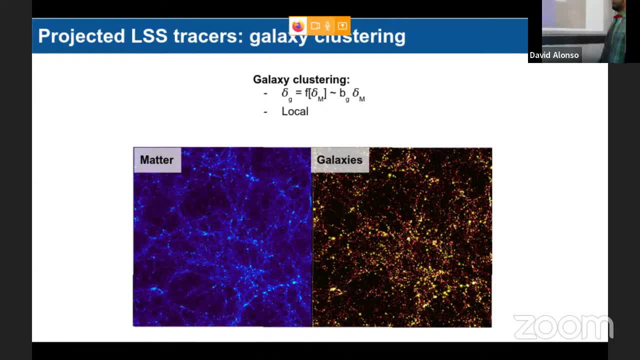 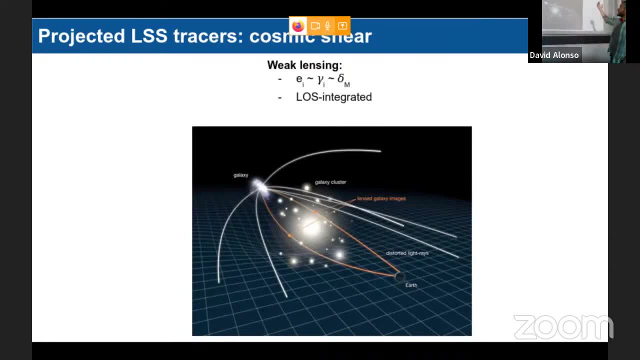 those galaxies are probing the matter. fluctuations at that redshift, That will become important later. The other probe I mentioned is weak lensing. So weak lensing is just the distortion in the paths of photons as they travel from some background source to us. 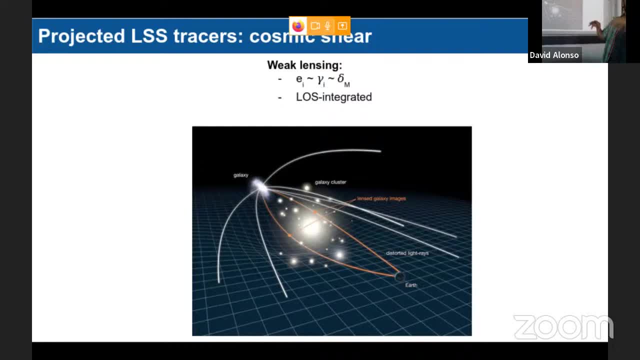 This distortion is caused by the gravitational field of the intervening logical structure. But we're talking. We're talking about weak lensing of background sources, background galaxies. We usually call that cosmic shear. So shearing is basically the deformation in the shapes of galaxies caused by weak lensing. 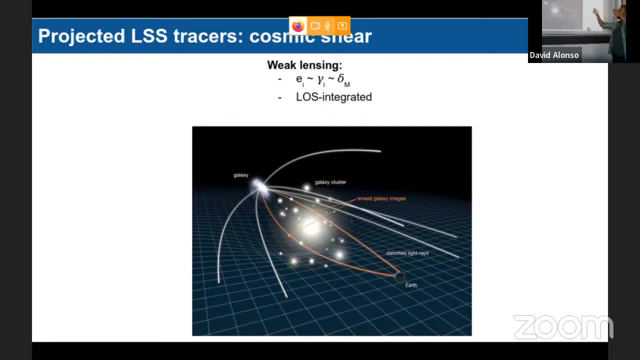 The idea is, we look at shapes of galaxies, We look at the correlations between these shapes of galaxies and that correlation, which would have been induced by the intervening logical structure, allows us to reconstruct that logical structure and then probe the matter. fluctuations, Because all matter causes gravity, weak lensing. 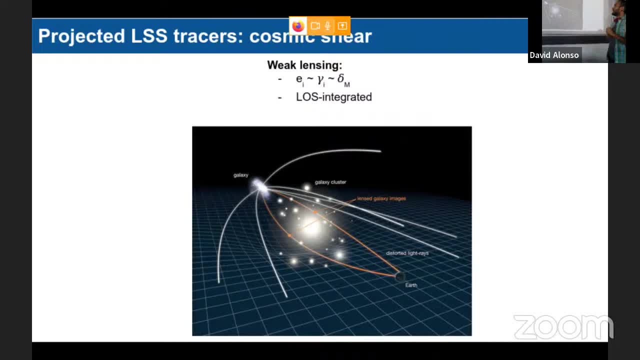 is an unbiased tracer of the matter fluctuations But it is a line of sight integrated tracer of the matter fluctuations, meaning that if you're looking at the cosmic shear effect of galaxies at the given redshift, the matter fluctuations you're sensitive to are all the matter fluctuations. 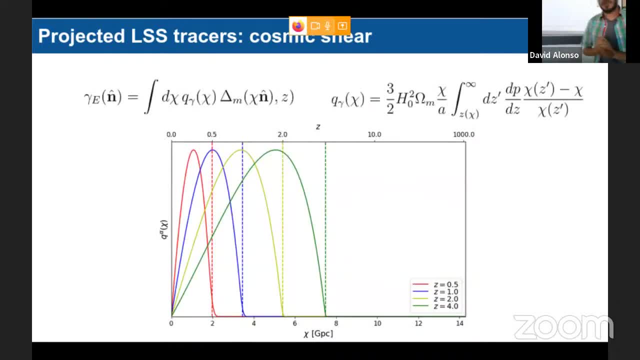 from that redshift to redshift zero And that's captured in this function here, Q, that I'm going to call the lensing efficiency, which essentially tells you how sensitive the cosmic shear map that you can make from galaxies at the given redshift. 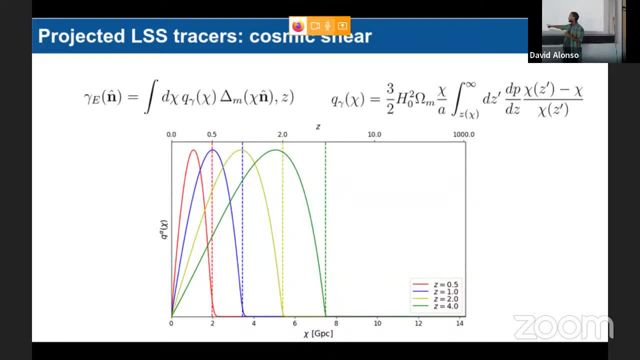 how sensitive that is to structure at different redshifts. So you have here the shape of that function. If you had source galaxies, let's say at redshift 0.5 or redshift 2, what you can see is that most of the information you're getting. 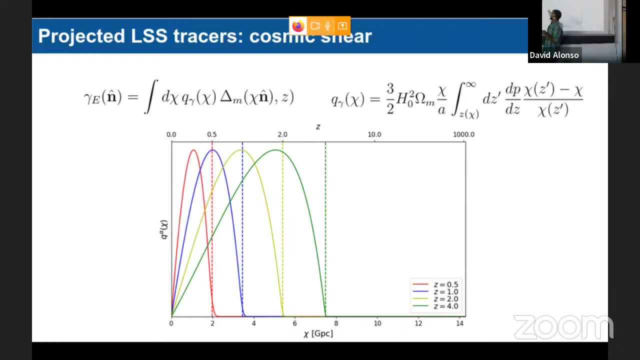 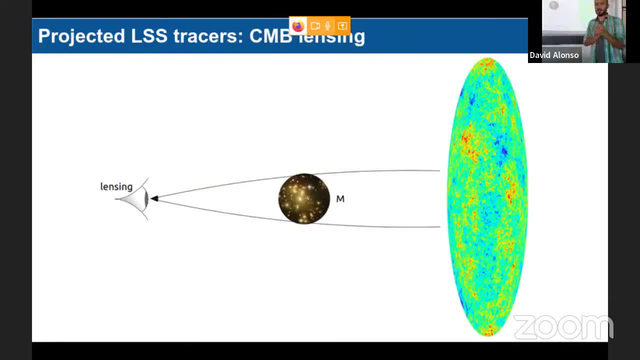 So that's again going to be important in a bit. And the last probe of the large-scale structure I wanted to mention is CMB lensing, which is essentially the same idea. It's just gravitational lensing, but now the photons that. 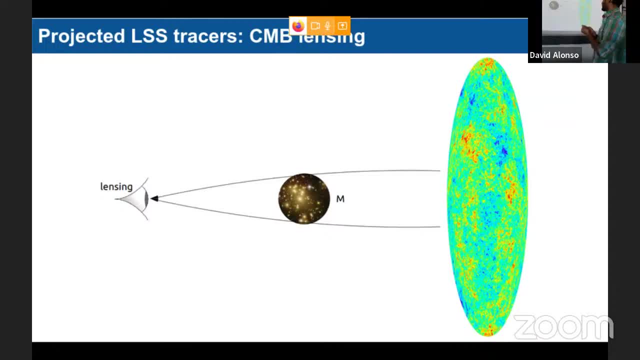 are being lensed are the photons emitted by the cosmic background. So the gravitational lensing effect effectively modifies the distribution of anisotropies in the CMB temperature map and causes additional correlations between those anisotropies. And by looking at those correlations, 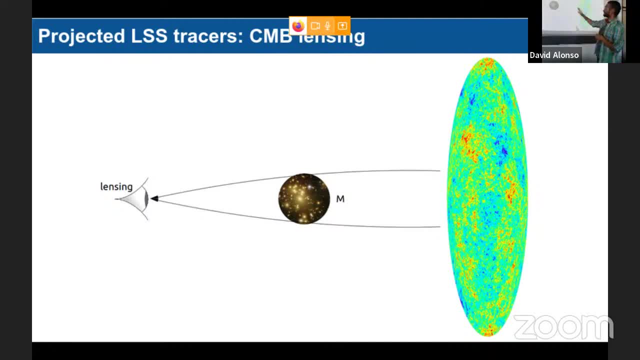 you can again reconstruct the projected large-scale structure that gave rise to that lensing. The best way to think about it for the purposes of this talk is just to think of having another set of sources that now lie at a really high redshift. 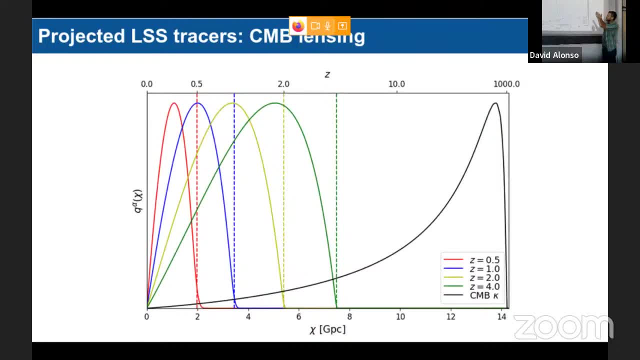 at the redshift of 100,000.. So, essentially because of CMB lensing, just think of it as something that is sitting at a redshift of 1,000 and allows you to look at the whole cumulative matter distribution from there to redshift 0. 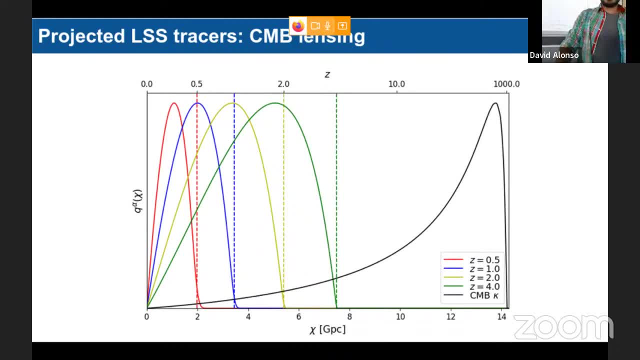 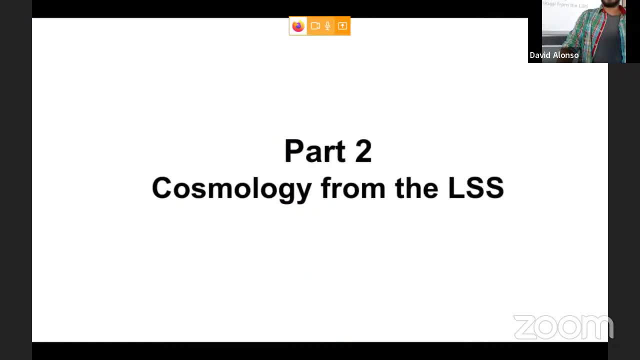 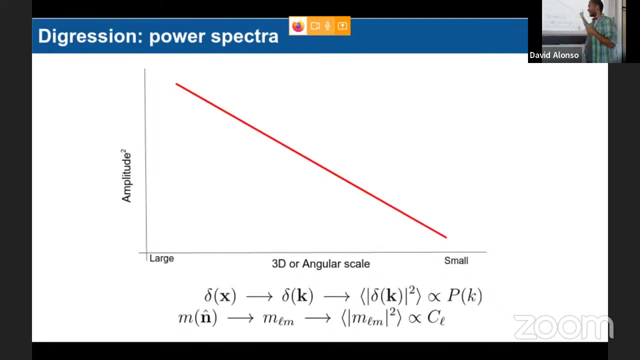 OK Now. so those are the tracers of the large-scale structure. Now, how do we extract information from these tracers about cosmology? So I'm going to go through this slide, because I promised myself that I was going to do this for a few years. 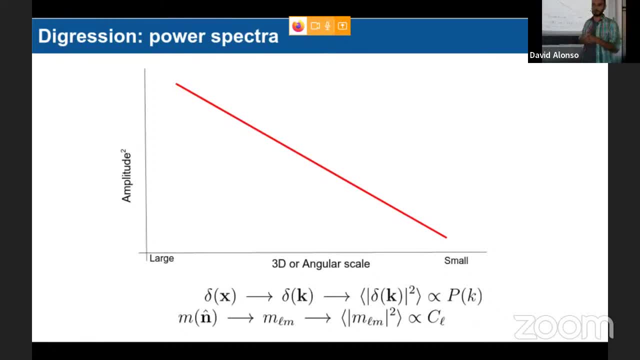 And this was after a conversation I had with a galaxy evolution person at Oxford where I was not complaining but I was saying: we go to cosmologists, go to galaxy evolution seminars. You guys put up a plot of property A, property B. 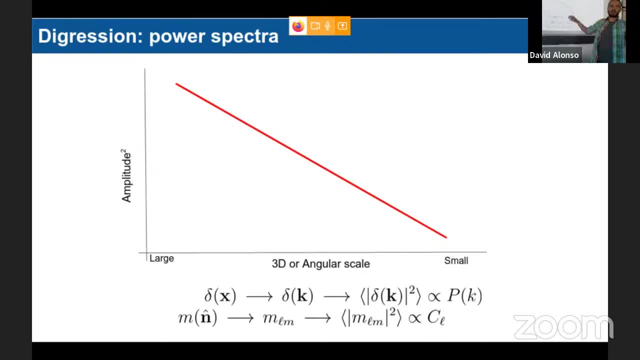 and it's a scatterplot. and then there's a line that goes through it And everyone's very excited and cosmologists are completely confused. We have no idea why we should be excited about that. And she complained back and told me: 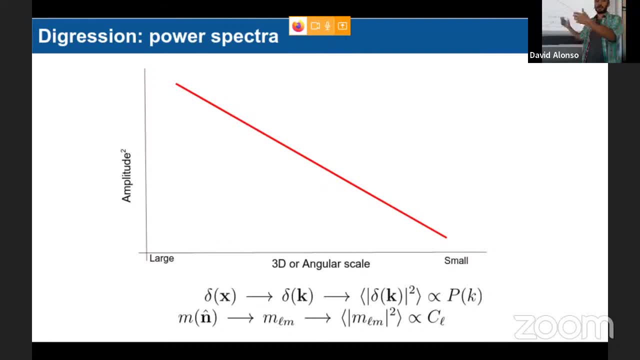 yes, when you go to a cosmology seminar, you guys show a power spectrum. We have no idea why a power spectrum is something to be excited about. So this is just explaining what a power spectrum is, because I'm trying to bridge the gap between the two communities. 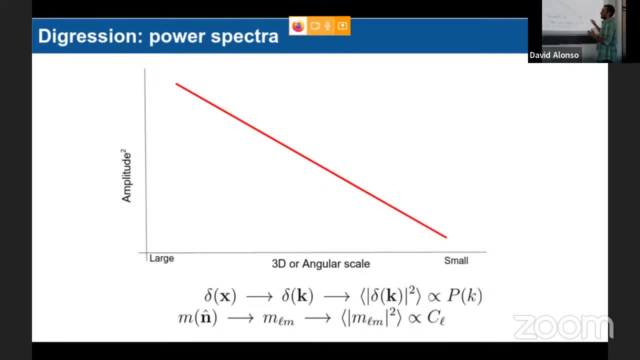 basically. So a power spectrum is extremely simple, right You have. a power spectrum is what we use in cosmology to study the properties of some field defined on the sphere or in three dimensions. OK, So let's say you've measured a field delta. 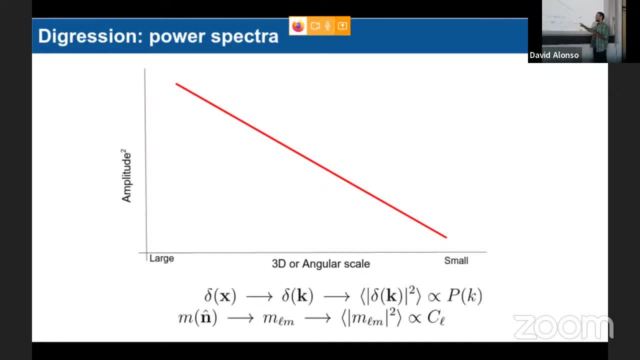 What you do is you put it in Fourier space and then just square it essentially, And that's effectively what a power spectrum is. The power spectrum is just telling you the amplitude of Fourier modes, so different oscillatory modes in that map. When we're looking at projected tracers, 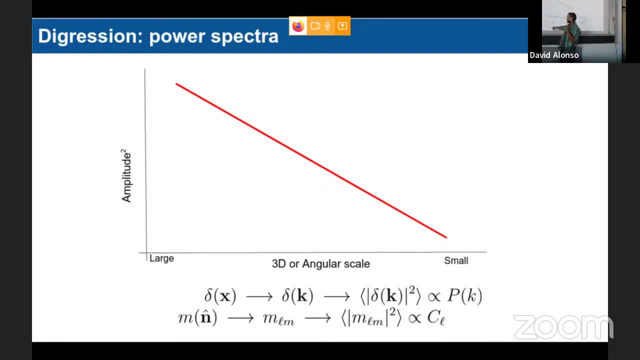 so things defined on the sphere, it's a Fourier transform. We do a spherical harmonic transform And the corresponding quantity is what we call the CL, the angular power spectrum. The interpretation is exactly the same And you can actually think of L as the amplitude. 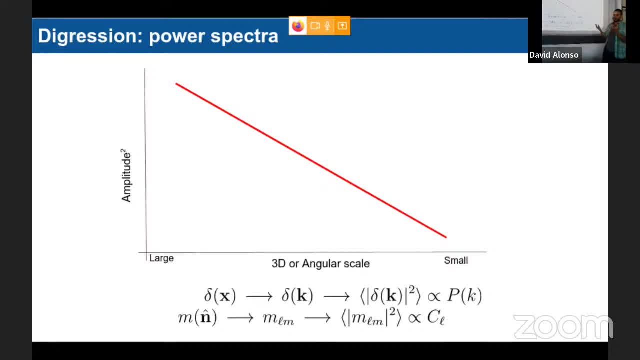 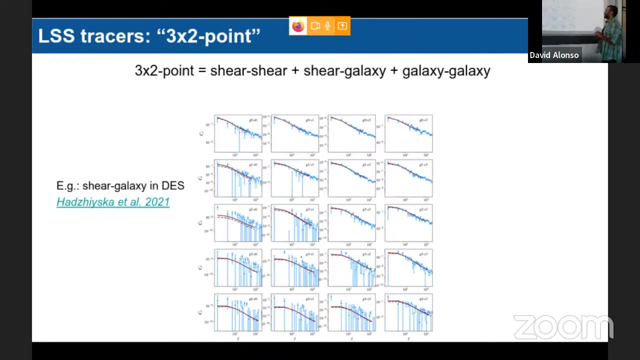 of the Fourier mode, now defined on the celestial sphere instead of in three dimensions. OK, That's all that. a power spectrum is Now. how do we extract information from tracers of the large-scale structure? The main way we do that. We do that in the context of photometric services. 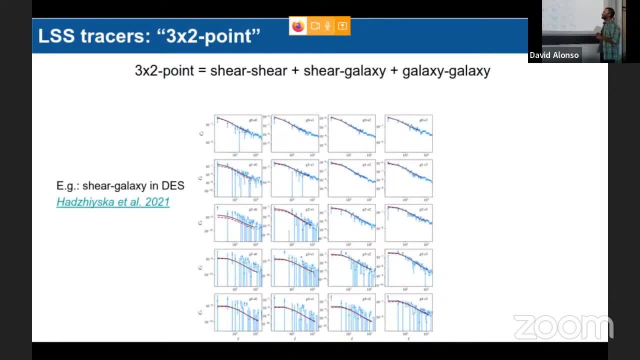 through something that you've probably heard quite a few times, something called the three times two-point analysis, So I wanted to spend some time just describing what that effectively is, even though maybe actually you've heard about this too many times already. So the three times two-point analysis effectively. 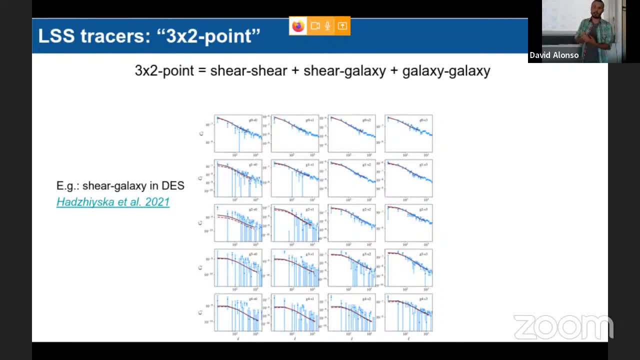 is the analysis of all possible two-point correlations between the two tracers of the large-scale structure we have. We have shear and galaxies, So we can look at the autocorrelation of the cosmic shear data, the cross-correlation with the galaxies and then the autocorrelation of the galaxies. 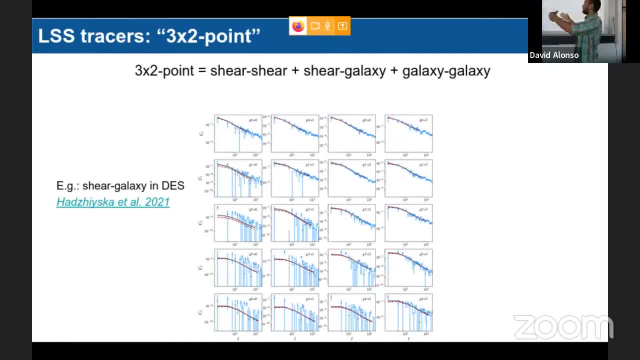 Moreover, we can always split galaxies into redshift bins So effectively. what we look at is all the possible autocorrelation between those redshift bins and the properties of these galaxies. There is an example, for example, that shows all the shear galaxy. 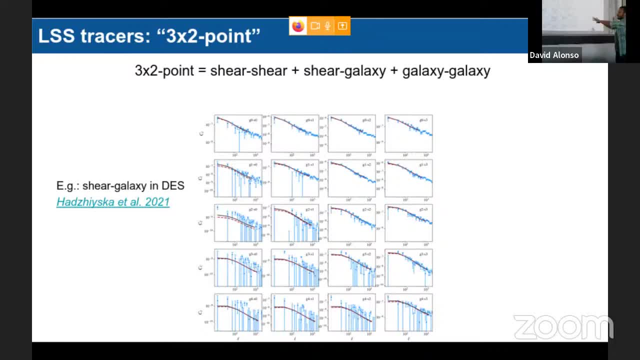 correlations in the year one, DS data. And this is all power spectrum. From now on, if I say correlation, just think of the power spectrum, All right, So let me try to give you a pictorial idea of how we extract information from these three correlation. 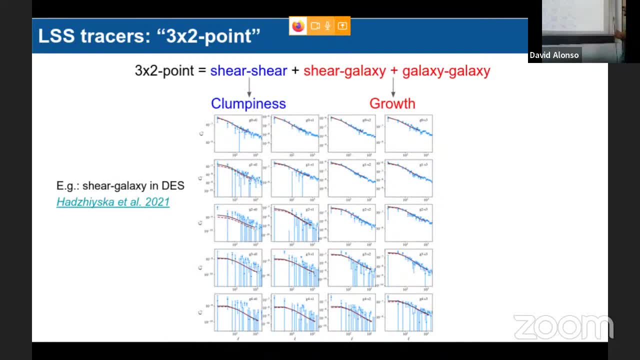 functions, And I think the best way to split the three times two-point analysis is into the shear-shear part on its own and then the combination of shear, galaxy and galaxy-galaxy, because they give you information about two different things. So shear-shear gives you information. 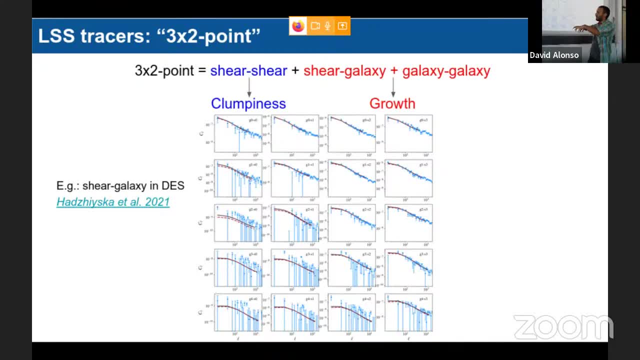 about the clumpiness. so the amount of, how large, how many observations are in the matter, fluctuations in the universe and the combination of shear galaxy and galaxy-galaxy tells you more about the evolution of those perturbations as a function of time. 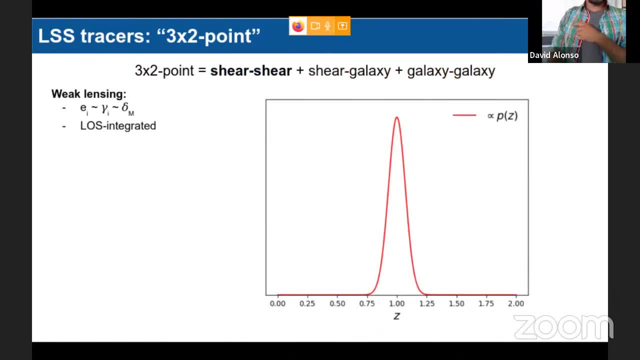 So let me explain how that works. So the reason for this is deeply tied to the main properties of these races, which I already mentioned. So the main thing that we need to bear in mind about cosmic shear, or weaklensing, is again that it's a line-of-sight. 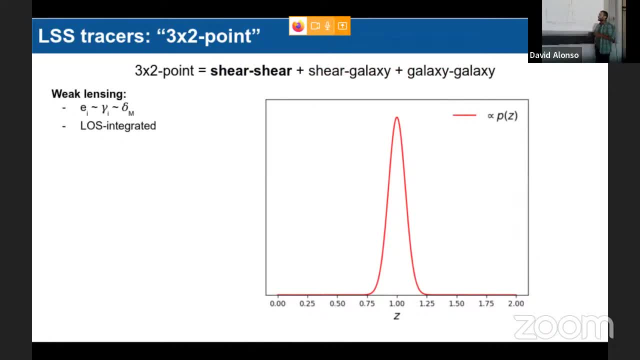 integrated quantity. So if you had galaxies distributed around redshift one, the lensing efficiency function actually looks like this. So you're actually picking up structure along the line-of-sight all the way to redshift zero And you're going to get a lot of contributions. 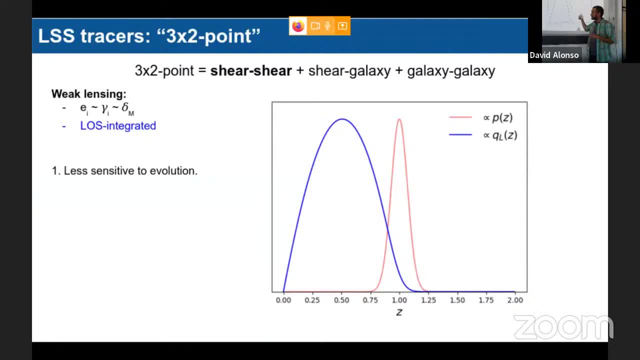 from very low redshifts. So this means several things. This means that, first of all, cosmic shear is going to be less sensitive to evolution effects than galaxy clustering, because you can't really resolve things very well in redshift. You have this huge kernel that you're integrating over. 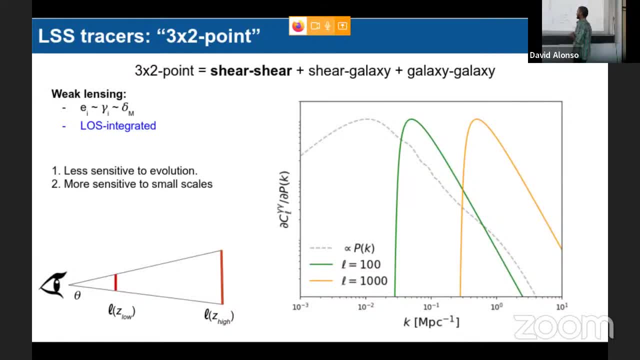 Also, the fact that you're always going to get contributions from low redshifts means that you're going to be sensitive to small scale. So things at low redshifts or even angular scale correspond to smaller physical scales. So let me try to explain this plot here. 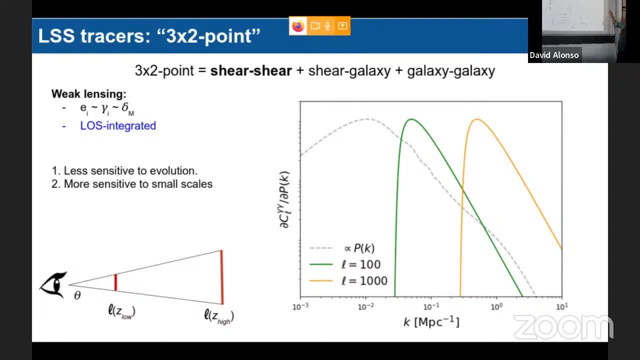 I think it's an important one. The quantity that we really want to reconstruct is the matter power spectrum, so the 3D underlying power spectrum of the matter fluctuation. What this plot is showing you, This is how much a given 3D Fourier mode. 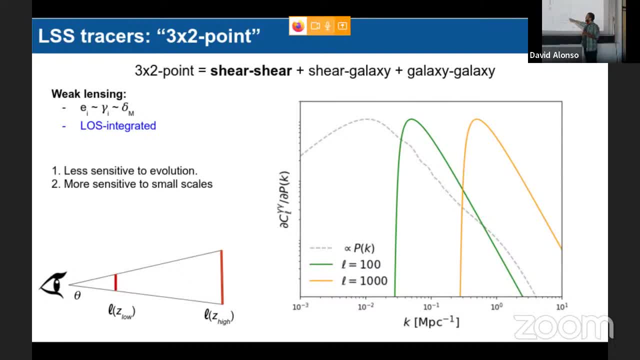 contributes to the total angular power spectrum at the given angular scale. So L of 100, corresponding to about 1 degree, L of 1,000, L of 10 to the degree right. So you can see that for L of 100,. 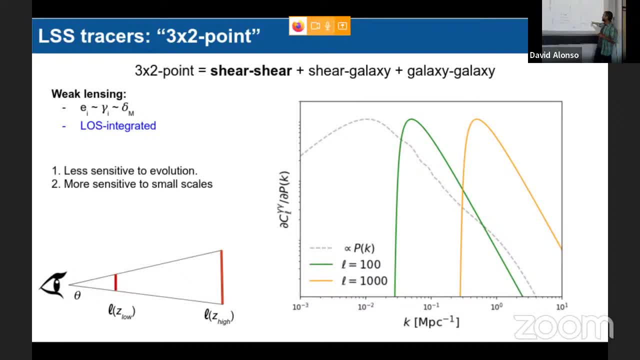 you're actually getting contributions from a wide range of scales to the total OK. So you're actually kind of averaging over all of these parts of the matter- power spectrum- just to get the angular power spectrum for cosmic shear at the given time. Invariably, you're always going to pick up. 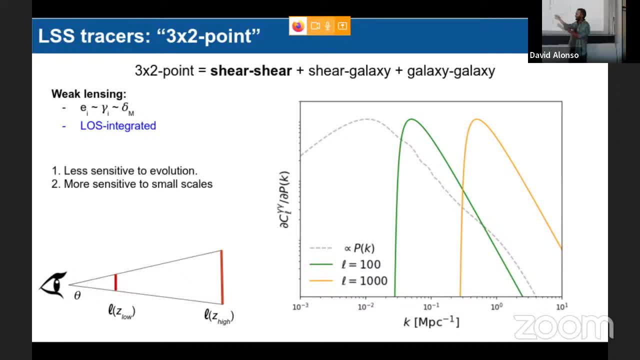 a lot of information from small scales because you're going to pick up fluctuations and low redshifts always, regardless of what redshifts you're looking at. So cosmic shear is always going to be more sensitive to small scale than other tracers. What is the relationship of the source? 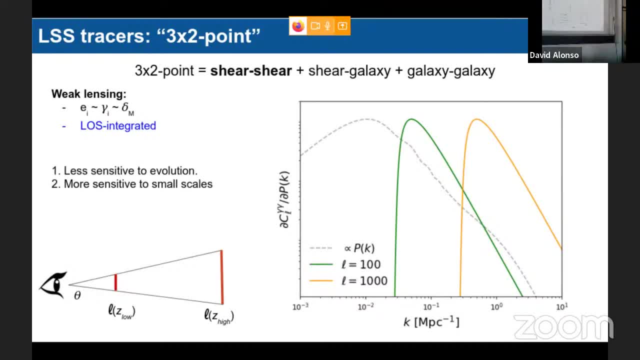 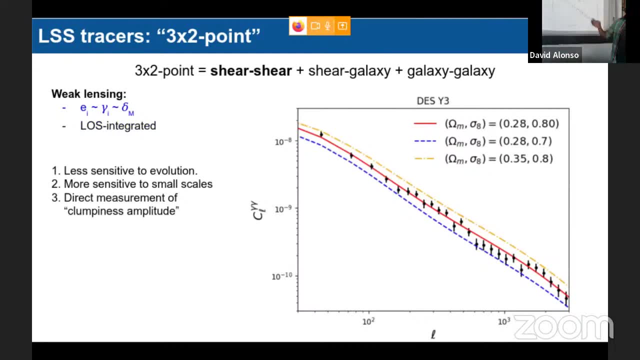 In this case it's redshift 1, actually, So it's quite far away. Also, please interrupt me whenever you want, because it's better to get feedback in the meantime as well, So I'm happy to answer questions whenever. 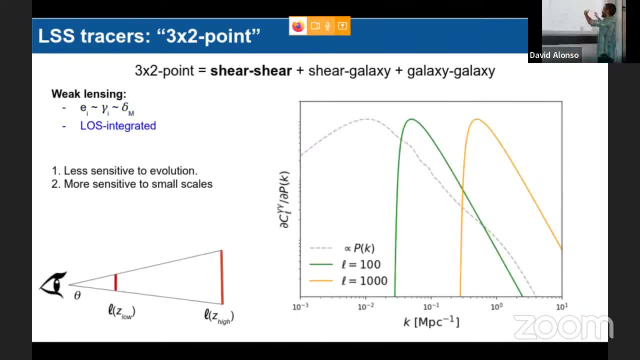 Also, the fact that you're averaging over all these huge range of scales whenever you're looking at a single angular scale means that a lot of the structure in the matter- power spectrum- is washed off, So you can't really reconstruct, for example, the variance of the oscillations. 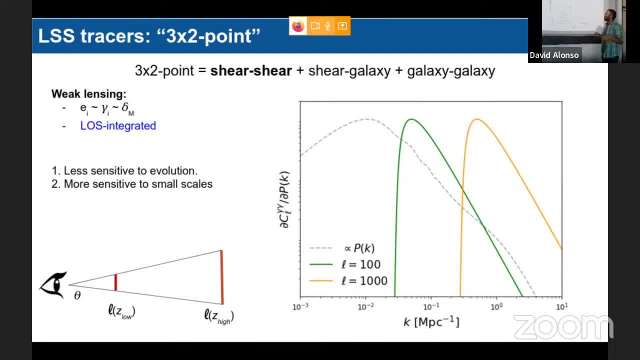 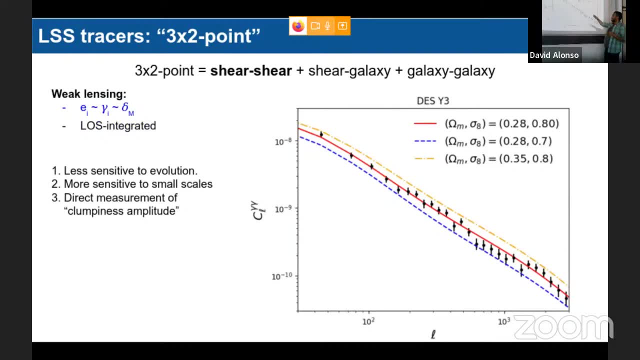 Right. Most of the scale dependence of the power spectrum is kind of lost in this operation, So the cosmic shear power spectrum usually looks rather boring. So this is, for example, the power spectrum for the third year. DES data Looks like a power lock-ish. 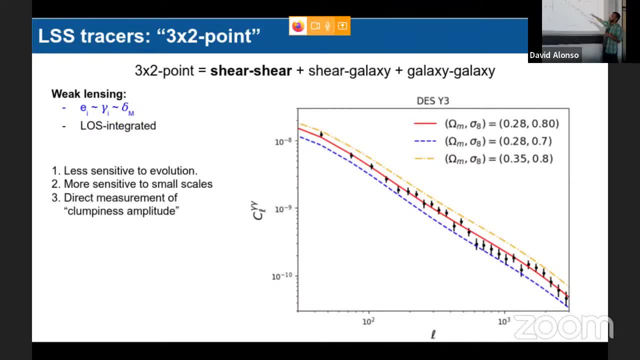 And so the main thing you're going to be able to say about this is roughly what the amplitude is. So you can find lots of combinations between two parameters, omega and sigma 8. Which I'll describe in a second That give you essentially the same thing. 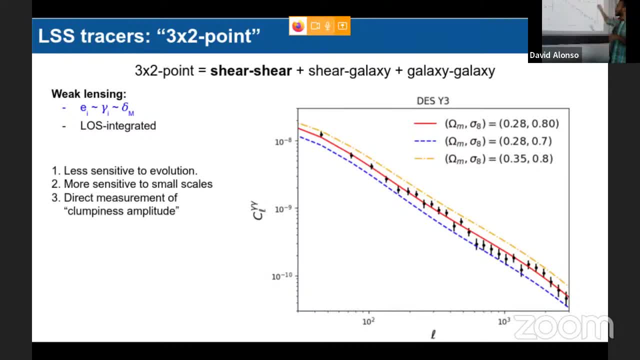 just scale up and down by an amplitude. So that's why I was saying the shear-shear part of three tends to point. mostly tells you about the global amplitude of fluctuations. OK, Then we turn to the other combination, so shear galaxy plus galaxy-galaxy. 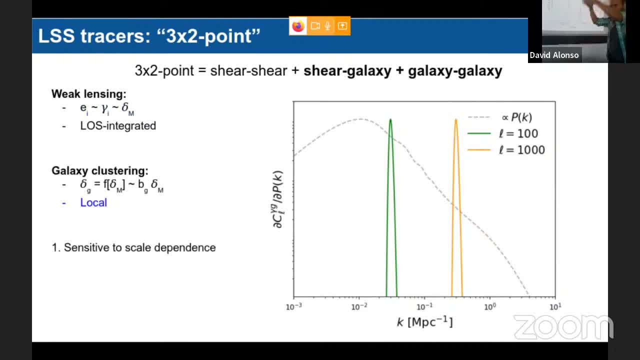 So in this case you're always looking at a cross-correlation that involves galaxies at the given well-defined set of ratios which are tracing the fluctuations in the matter distribution at that ratio. So that means that if you look at a given angular scale, 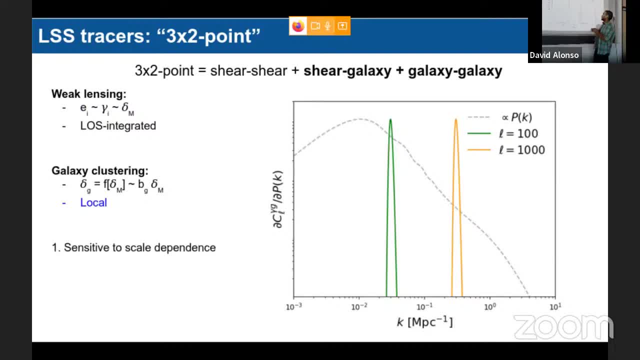 you're going to be looking at a very specific range of physical scales because the ratios of these galaxies are well-defined. So that means that these two correlations are going to be a bit more sensitive to scale dependence of the matter-power spectrum than the shear-shear. 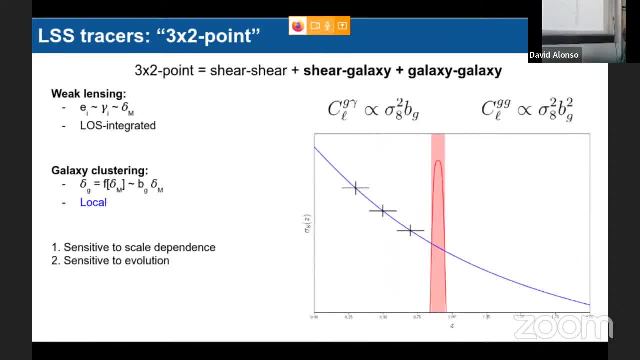 correlation And you're also going to be more sensitive to evolution effect. So you're going to be able to reconstruct the evolution of growth as a function of that And you're also going to be able to reconstruct the evolution of growth as a function of time. 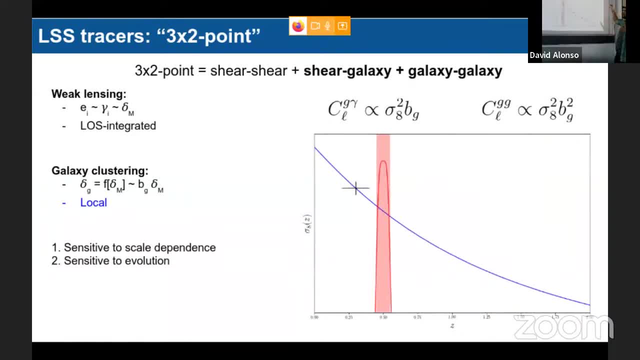 or the evolution in the amplitude of fluctuations of the function of time. So the way to try to understand that is, if you look at the, for example, the cross-correlation between galaxies and cosmic shear, that's going to be proportional to sigma-8 squared. 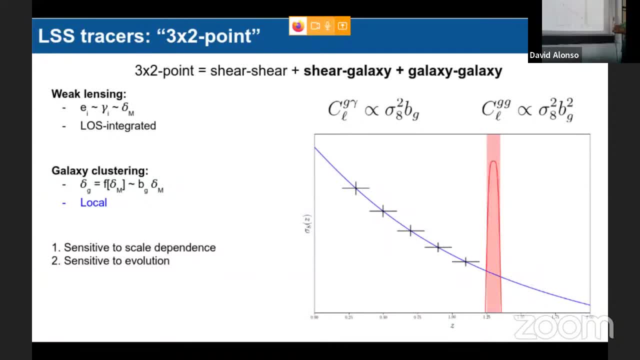 So sigma-8, I should have described it before- is a measure of the amplitude of matter fluctuations. So any power spectrum will always be sensitive or proportional roughly to sigma-8 squared times one power of the galaxy bias, whereas the outer correlation will be 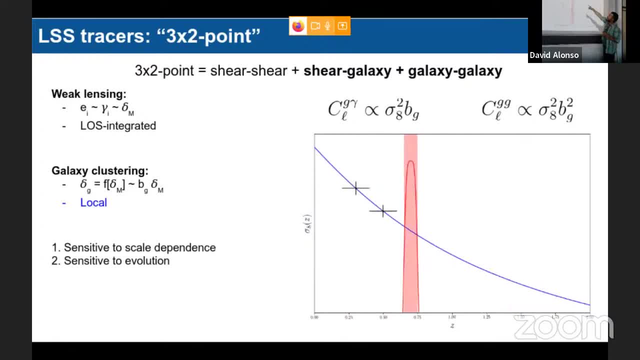 sigma-8 squared times the galaxy bias squared. So if you combine two of these at the given redshift, you're able to break the degeneracy between galaxy bias and sigma-8, and effectively measure sigma-8 as a function of. 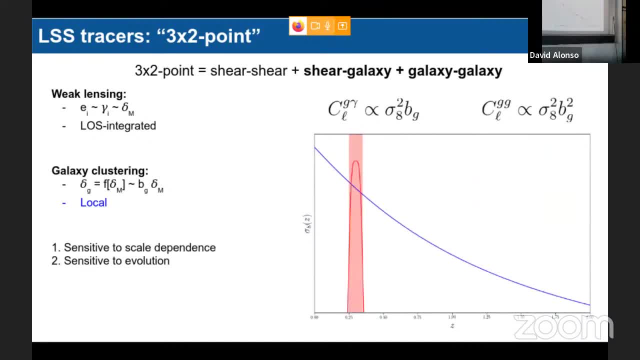 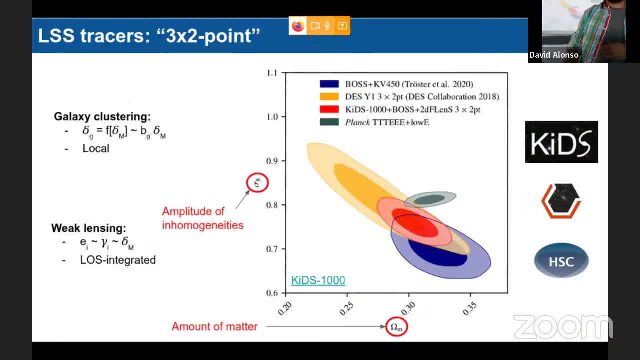 That's kind of the historical idea for why this combination allows you to reconstruct the evolution in the growth of structure. Yeah, so combining cosmic shear and galaxy clustering, you can, You can put. The main cosmological parameters you can constrain, at least with current data, are omega-m and sigma-8.. 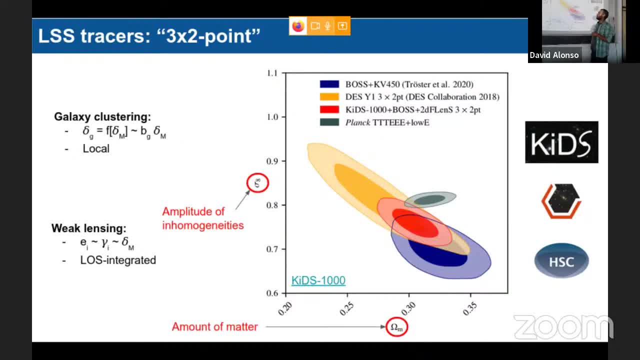 Sigma-8, I already said, is basically a measurement of the amplitude of, And omega-m is the fractional amount of non-relative in the universe. So this picture here shows the constraints from several experiments. Maybe the ones to look at here are kids, for example in red. 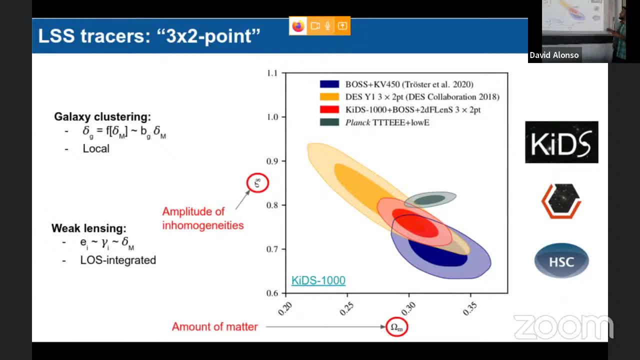 Or DES. this is from the third year of DES, where you have these constraints on these two big things, sigma-8 and omega-m. But one thing to notice from this plot is that most constraints from either shear-shear or three times two points have this kind of degeneracy. 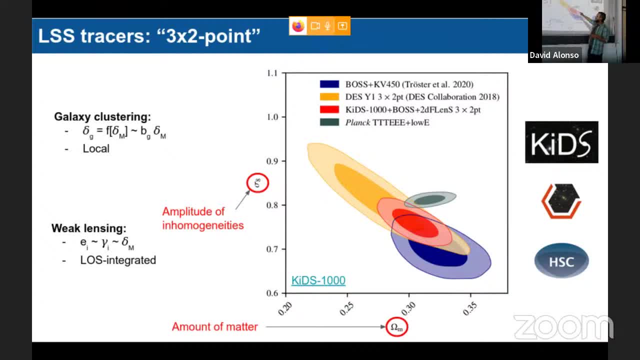 between omega-m and sigma-8.. So the actual parameter that you're able to measure very well is kind of whatever is going on in this perpendicular direction, And that's the reason why when you see talks that involve three times two point analysis. 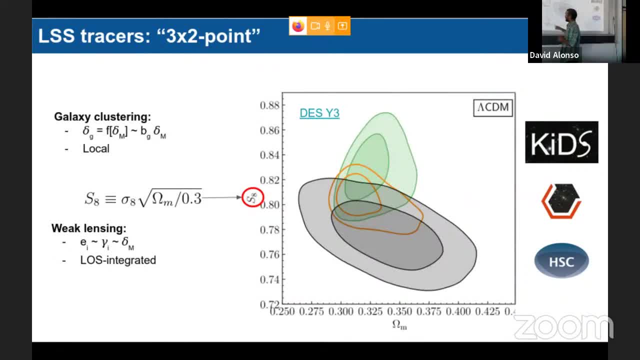 very often you hear about this parameter called S8, which is just a combination of sigma-8 and omega-m. that is the combination that is roughly the best measured parameter for this type of analysis. So sometimes you'll see plots like that, And in fact I'm going to keep on referring to S8 from now on. 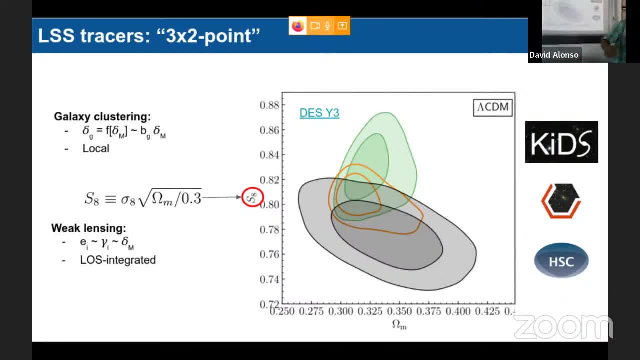 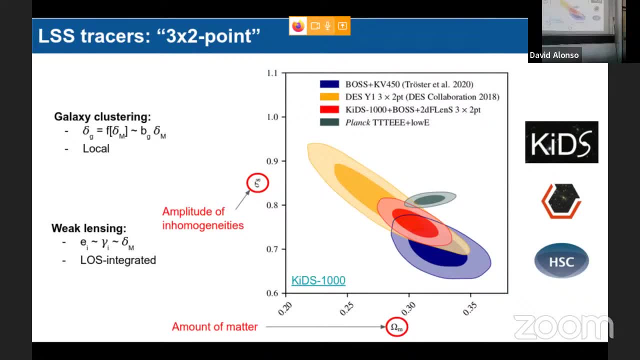 The main. yeah, Yes, yes, Exactly yes. So for each of these contour plots- and I'll be showing more of them- this will obviously be 68% for one sigma and 95%. So there's There's a tension between the Planck and Bose. 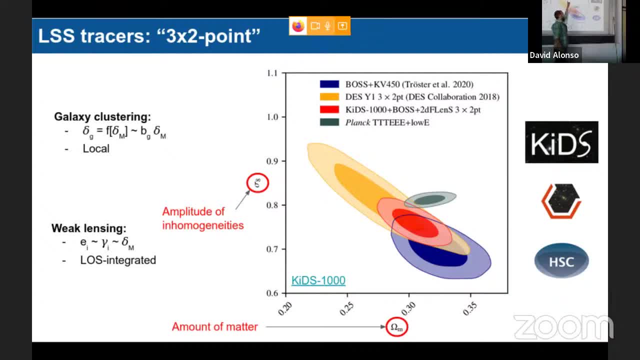 There's a three sigma tension. If you quantify it, you'll probably know the big number: The three sigma between the Gibbs result and Planck. So yeah, So this is what I wanted to mention. So the other contour there is the inferred value. 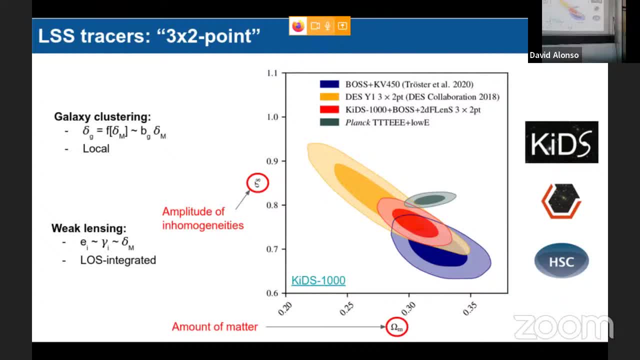 for this parameter from the pure CMB's primordial fluctuations. OK, So what's going on there is, the CMB is a very it's mostly sensitive to the early universe right, So it can measure the fluctuations in the matter distribution at really early times very well. 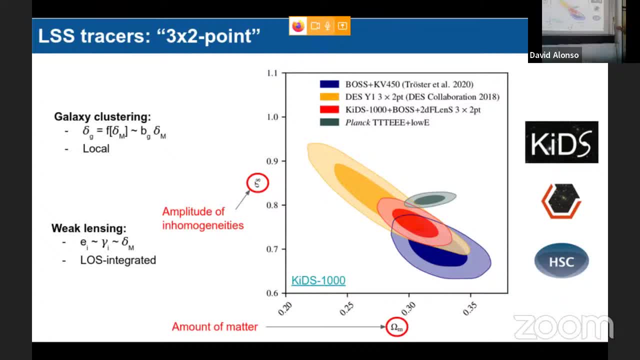 And from that it's actually able to measure, to constrain the parameters of the CMB. And having constrained those parameters, what they can do is they can predict what the amplitude of fluctuation should be at late times. So that's what's going on, right. 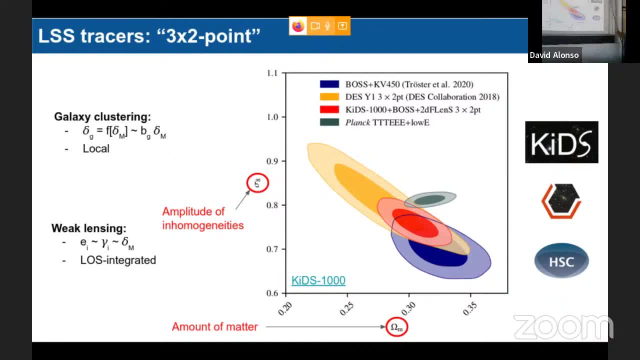 So within the CMB model, Planck predicts that the amplitude of fluctuation should be this: You can think of weak lensing measurements as being a direct measurement of that amplitude. that seems to be in slight tension, And I'll get back to the tension actually. 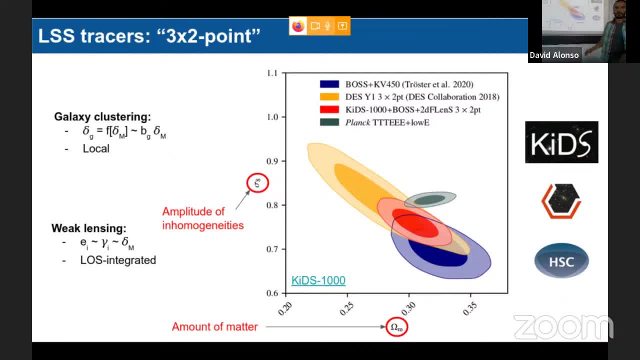 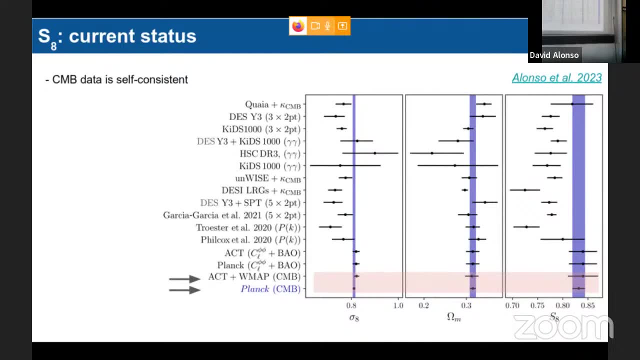 OK, Cool. So actually, let's look at that tension, Right? So what I'm showing here is a sigmite, omega m and mostly SA. So let's focus on SA for now. Ignore that. I think that will become important later on. 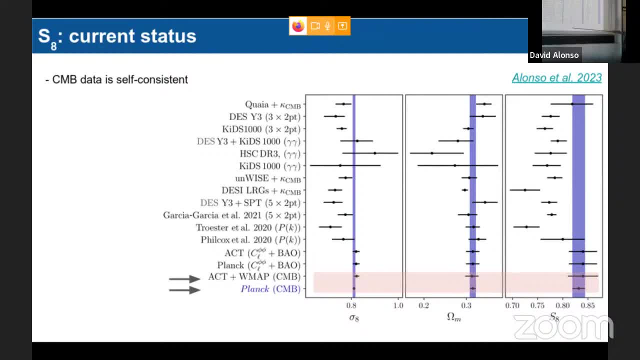 And then the measurements of SA by different experiments: Right. So the two at the bottom are Planck and the combination of act and WMAP, Right. So the first conclusion we can draw is that the measurements of sigmite are consistent across the CMB experiments. 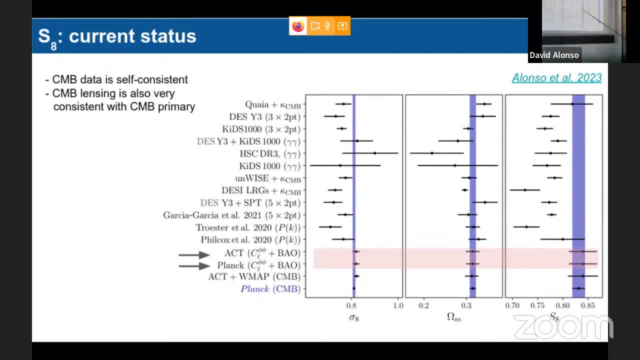 Moreover, if we look at just the CMB lensing effect from those CMB experiments- so we do not take into account the primary fluctuations, just the CMB lensing- they also seem to recover the same amount of clustering as CMB. 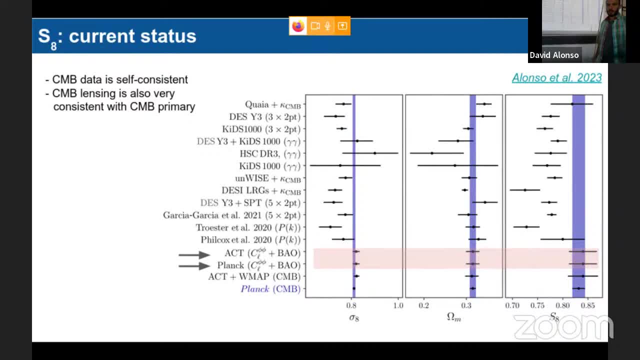 So it agrees with primary CMB data. If we then move on to just the sheer, sheer part of the three times two points, right, most of these measurements consistently get you a value of SA that is lower than Planck- Not by a lot. 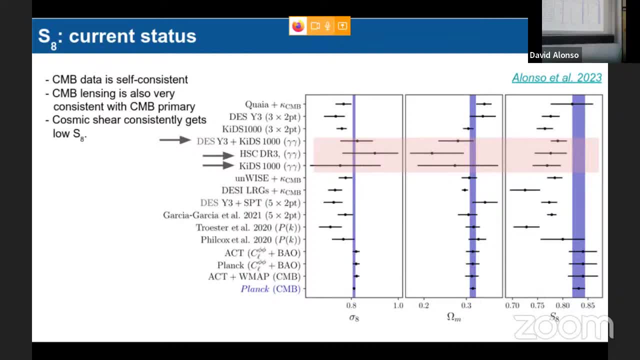 So, individually, they're always fluctuating between two and three sigma, But the fact that they're consistently low is what gives rise to this kind of SA idea of an SA tension. When you combine with galaxy clustering, very often you do see the same kind of tension. 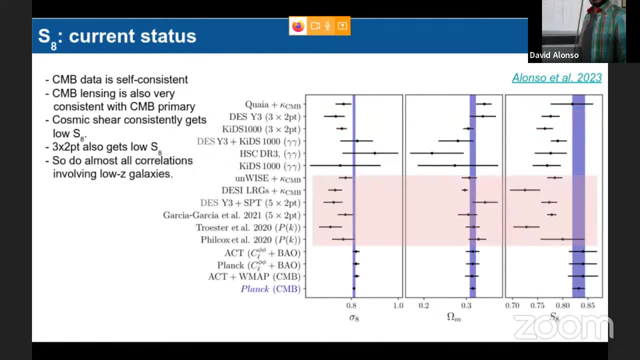 And almost all other, or many of the other studies that look at low redshift data in different combinations. So this is looking at galaxy clustering and CMB lensing, So no cosmic shear, for example. And then, if you see, five times two points. 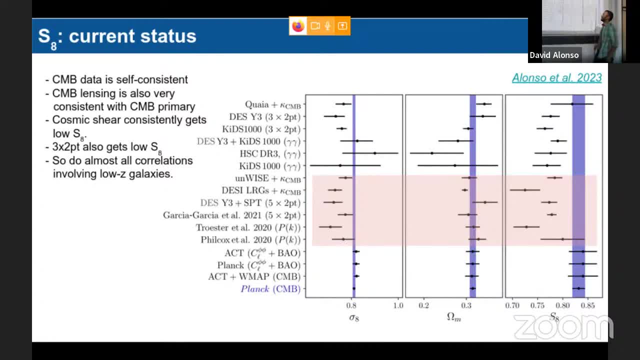 this is just three times two points, but you also have CMB lensing, for example. The point is, all of these low redshift measurements under the key that is, low redshift, give you a consistently low value of SA. OK, OK. 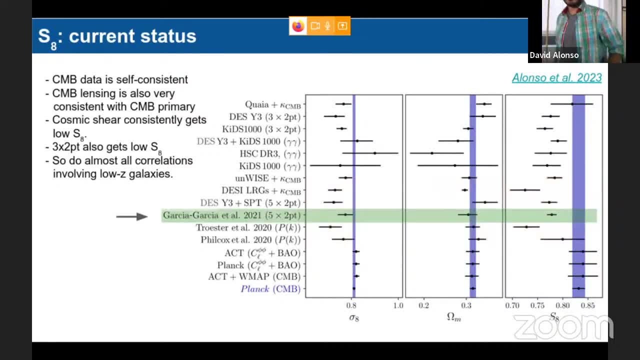 So that's kind of the state of affairs. So we could try to figure out or try to think about these results and think what are the possibilities, What could be causing this SA tension? So let me see how much time I have, Good. 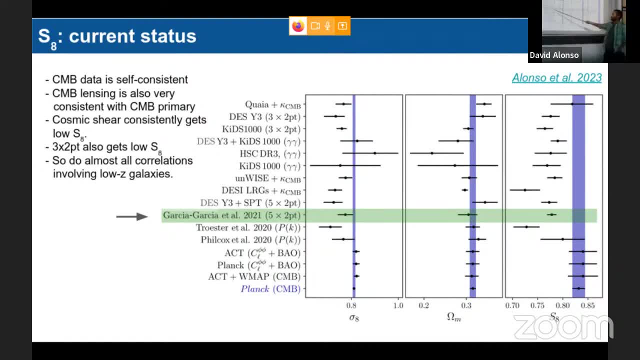 All right. So there was a paper that we wrote back in 2021 with data that was whatever the latest data was there at that point That tried to address this thing right, Trying to understand where the tension is coming from. So there's new data that has come out since then. 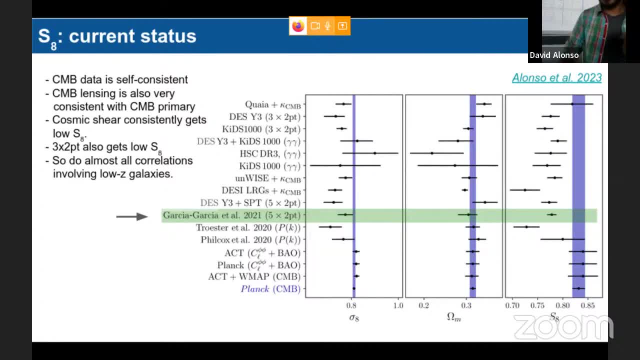 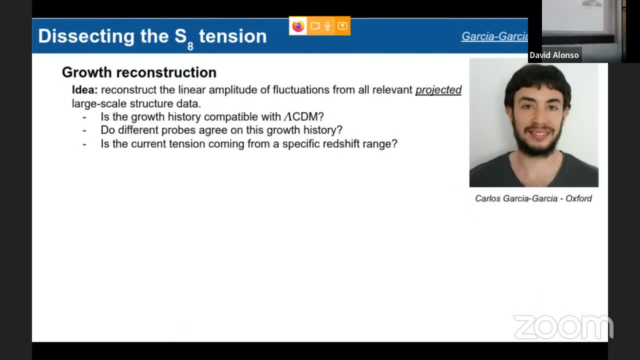 but I think it's a useful paper to look at. I'm not going to describe it in detail, but I thought I would point it out. So this was a paper that was led by one of our fellows at Oxford, Samuel Garcia, And his idea there was trying to use all of the data. 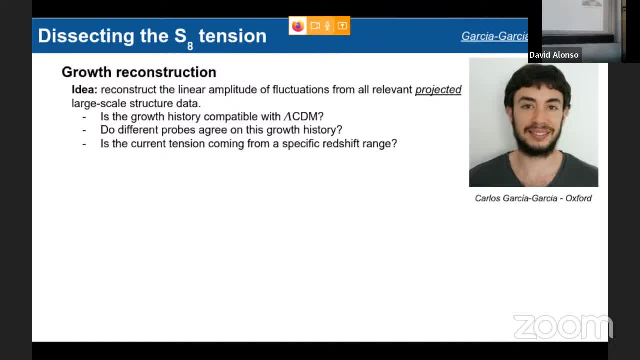 that we currently had at that point from cosmic shear, galaxy clustering and CMB lensing. to try to reconstruct the value of SA as a function of redshift, as given by the data directly, To try to understand whether is it just the value of SA. 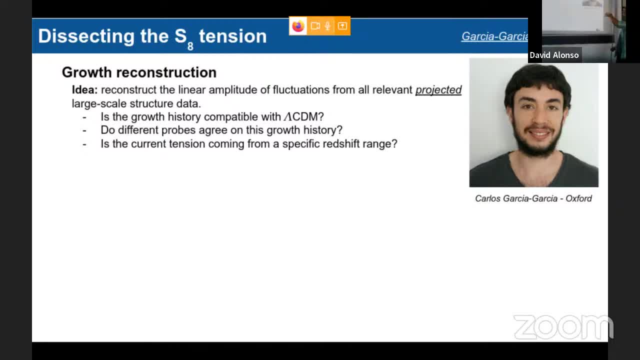 that is intentional, or is it the whole growth history that is intentional? with lambda-CVM Do we see a growth history that is incompatible with what lambda-CVM would predict? Do different probes agree with this growth history? And if that's not the case, then that might point. 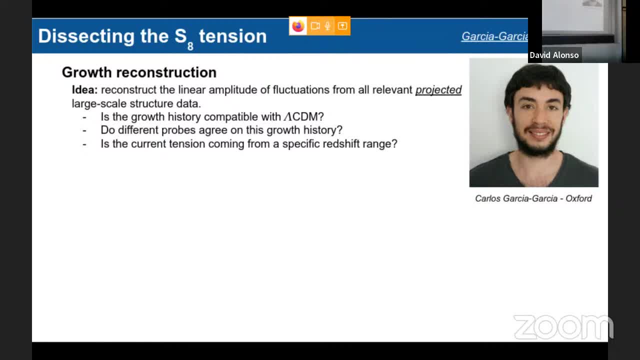 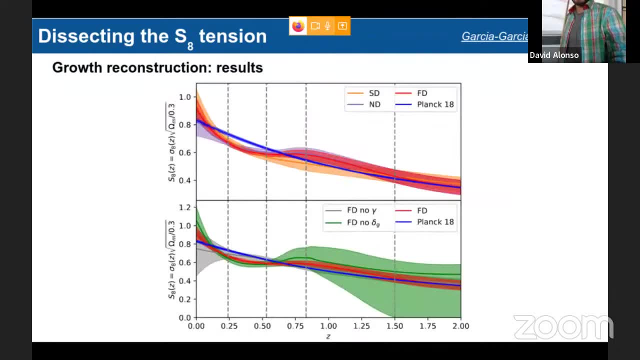 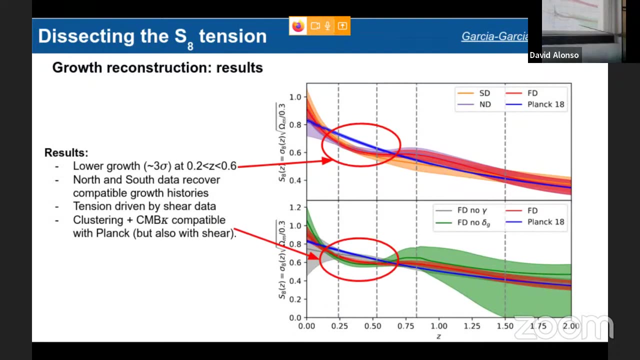 to systematics in one of the probes And whether this tension is coming back from a specific range of redshifts. So I'll just show you the main result, without going into details, which is this: So this is x-axis, is redshift and y-axis 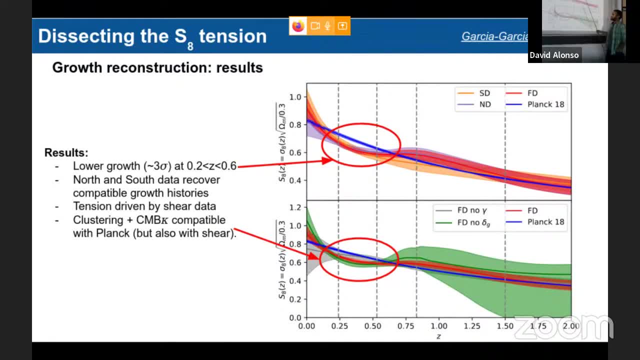 is the reconstructed value of SA as a function of redshift. So just think of how the amplitude of perturbations is growing as a function of that. So the Planck result- assuming lambda-CVM- is in blue, and then you have the predictions from. 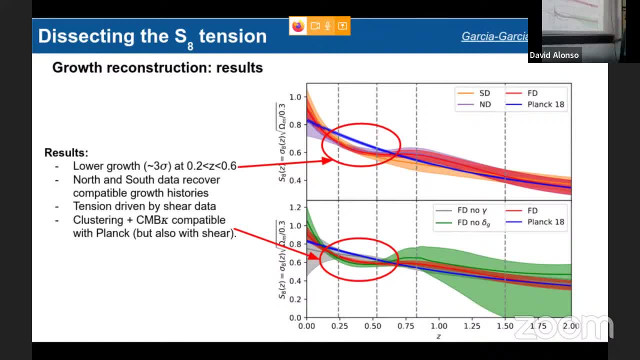 or the inference from different combinations of data. So SD and ND are just two different sets of data which are based on cosmic shear from DES or cosmic shear from KITS. So it allows you to see whether the two surveys are in tension with one another or not. 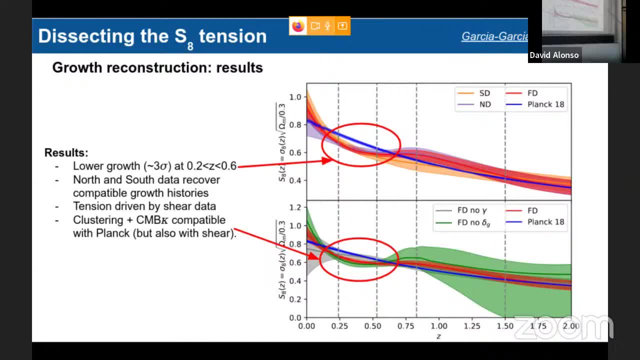 And the answer is they're not. And then he looked also at splits between using cosmic shear or not, using galactic clustering or not and things like that, And the main conclusions were that where you see a lot of the tension coming from is there's range of redshifts where 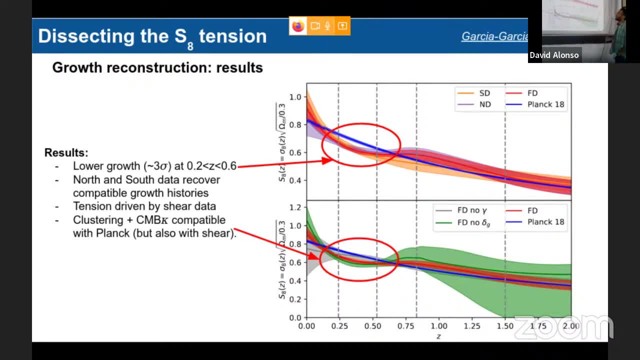 you have the best training power. so where your errors are smaller, which is no surprise, So it's very low redshift right. So it's coming from redshift 0.2 to 0.50-something- The level of tension there seems to be. 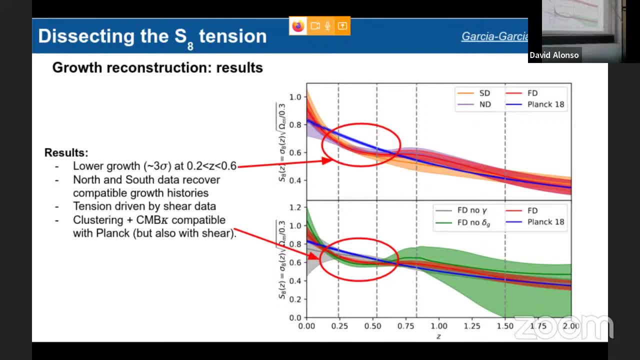 at the level of 3 sigma And this is the range of redshifts. that is where cosmic shear data are most sensitive to At least the cosmic shear data we looked at back then And in fact, when you remove galactic clustering. 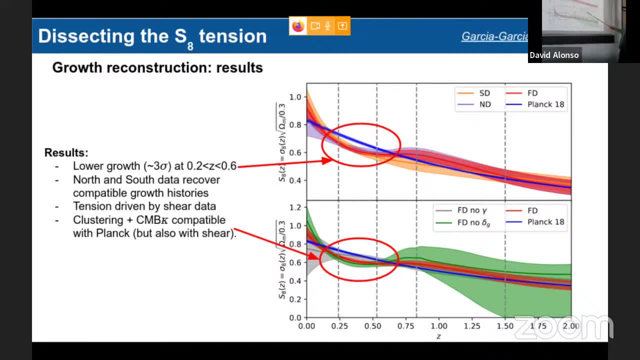 a lot of the tension went away, But it stayed if you had no galactic clustering and only relied on cosmic shear. It doesn't mean that galactic clustering and cosmic shear are in tension. It's because when you separate them, the error bars go up. 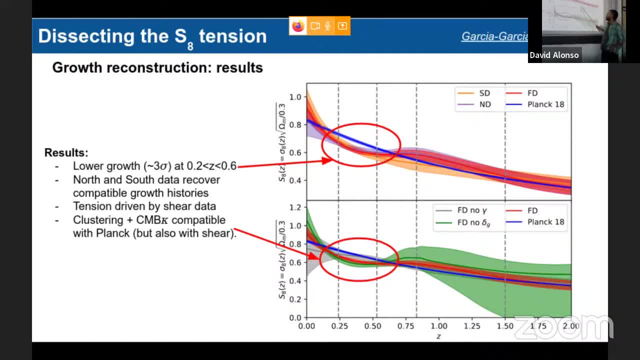 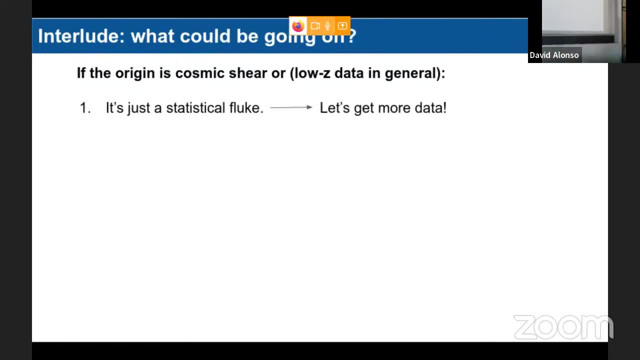 And it's not like they're really in tension, But the tension seems to only show up when you have cosmic shear, at least for the data set that we Right OK. so with that in mind, let's try to think about what could be the different causes. 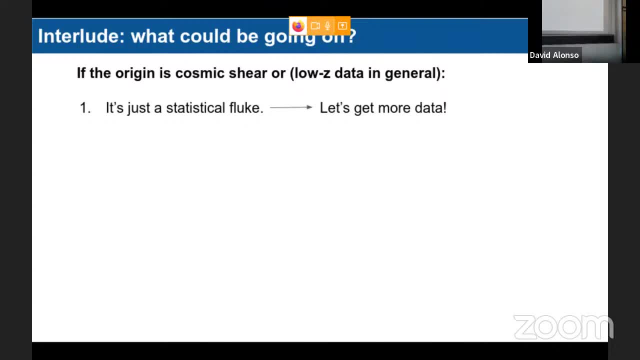 for the tension. So if we assume that the conclusion is that the origin of this is either cosmic shear or, in general, just the fact that we're sensitive to the matter- fluctuations at very low redshifts- there could be different definitions. So the first one is OK, it's just a typical fluke. 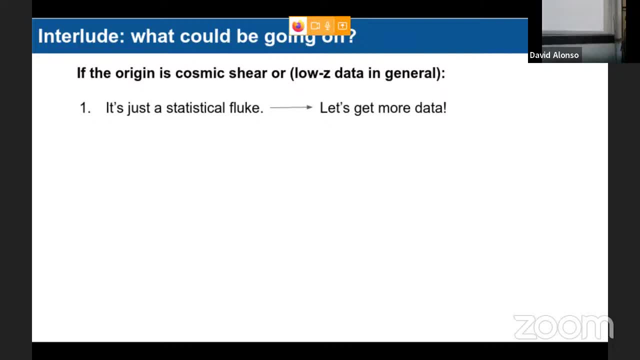 We just get more data, wait for LSS to come online, then we'll know if this is true or not. But that's kind of boring. The more exciting situation would be if there's actually slower growth at low redshifts and this is an indication of new physics- dark energy. 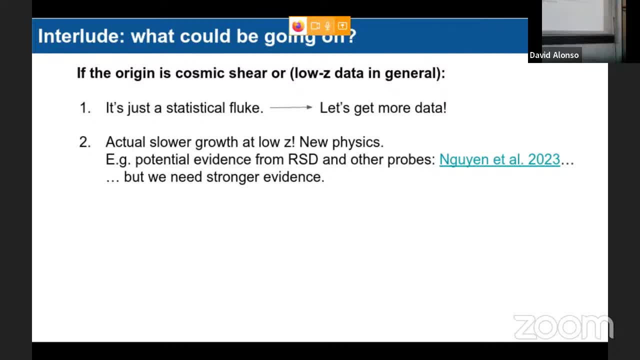 or something like that, And there might be some evidence from other distorsions. There was a nice paper by Mingyuan earlier this year, But I would say 3 sigma to 4 sigma evidence is not enough to actually train the physics. 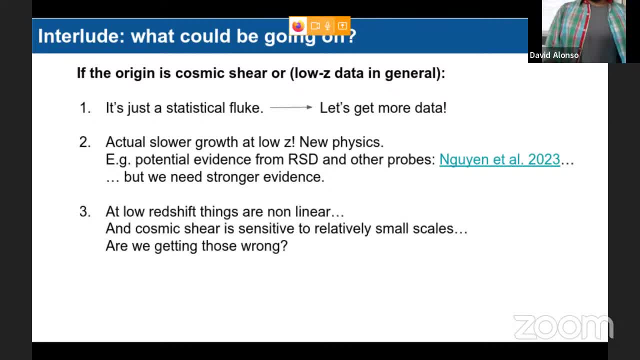 so we need to keep thinking a little bit more as well. The thing, if we think about it, is we assume that there could be something wrong with how we're analyzing this data. The thing that is characteristic of low redshifts is that the matter fluctuations are nonlinear. 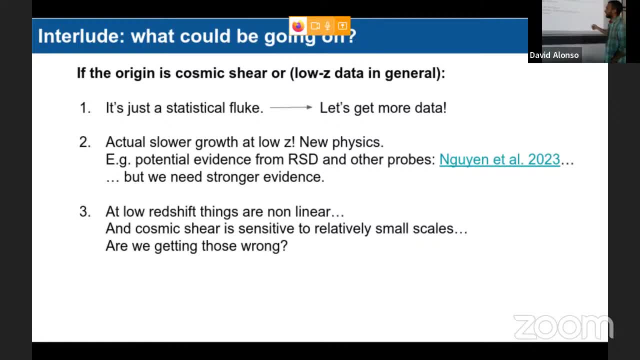 and you're mostly sensitive to small scales, which are even more nonlinear, particularly when we're talking about cosmic shear. So could it be that there's something wrong with our way of modeling the nonlinear structure formation? So there's two different ways to try to address that? 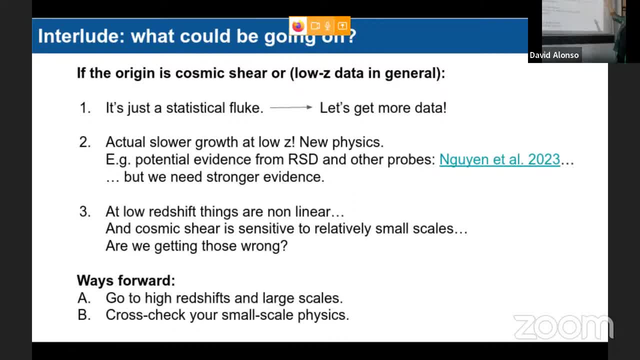 One way is to go to higher levels and try to measure high redshifts. try to measure cosmological parameters at very high redshifts and particularly targeting large scales, because that allows you to see the complement of these and see if those actually agree with Landa-CVM or not. 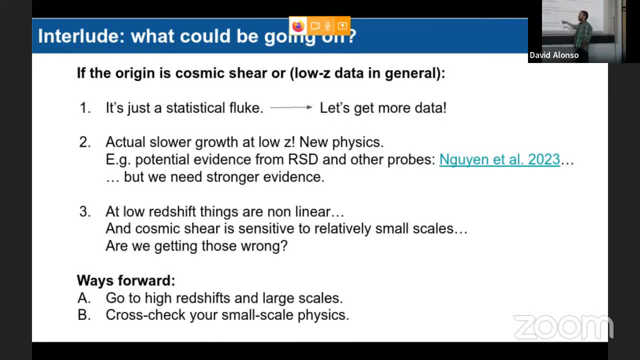 And the other option is to just cross-check, see if we have other probes that allow us to figure out whether the way we're treating the matter- fluctuations at small scales- is correct or not. So I'm going to talk about these two options. So going to high redshifts. 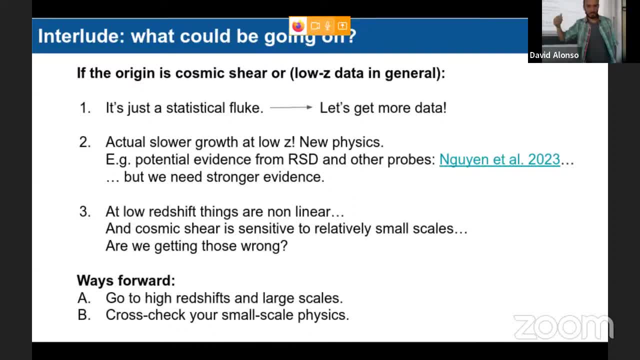 first of all is I'm going to explain why. but the reason is, if you go to high redshifts, it's only at high redshifts that you have access to the larger scales that are not that wouldn't be sensitive to this nonlinear. 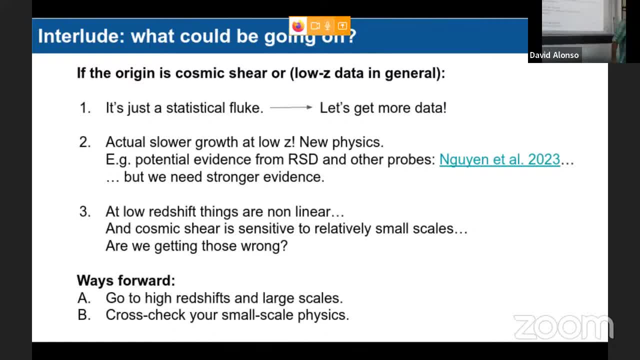 or less sensitive to this nonlinear Well, we can confirm whether this is actually so. if we get the same level of tension from high redshifts, then we know that it's actually not due to the nonlinear scales. You don't know anything. 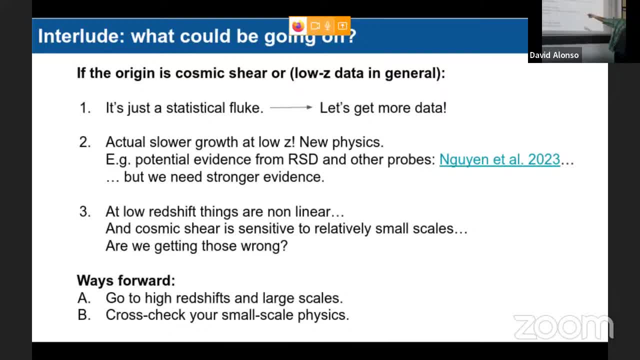 but you at least are sure that the problem is in nonlinear scales at low redshifts, right? So you've checked linear scales at high redshifts and those are fine. It could still be neophysis. yes, It could still be neophysis. 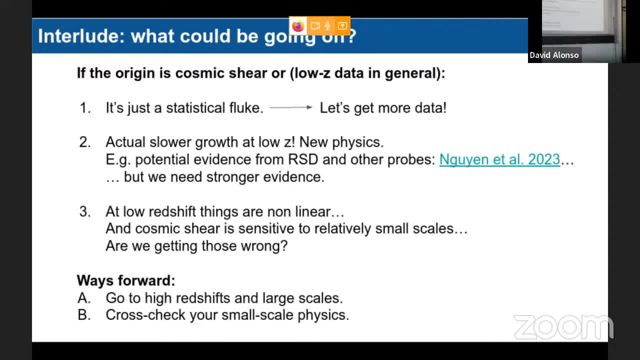 but it would be neophysis that doesn't show up at high redshifts or at very large scales. So it's trying to narrow down exactly where it's coming from right And there are very few actual measurements of the amphitheater of fluctuations. 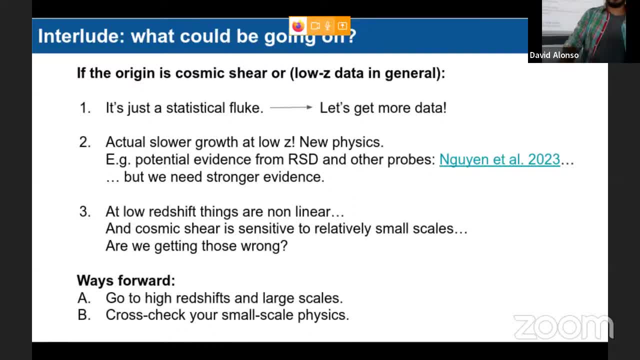 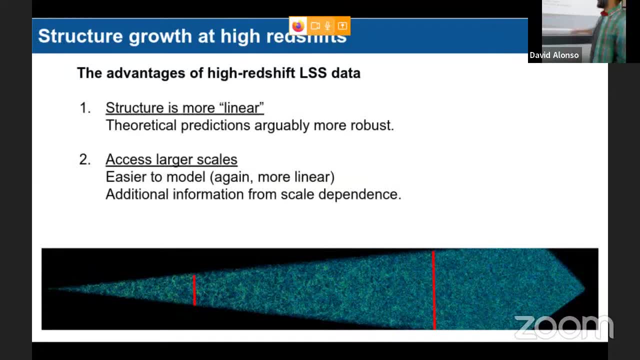 at the redshifts that I'm going to be talking about. so it's an untrivial thing to ask, Right, okay, so how can we go to high redshifts? As I said, the main reason why it's interesting. 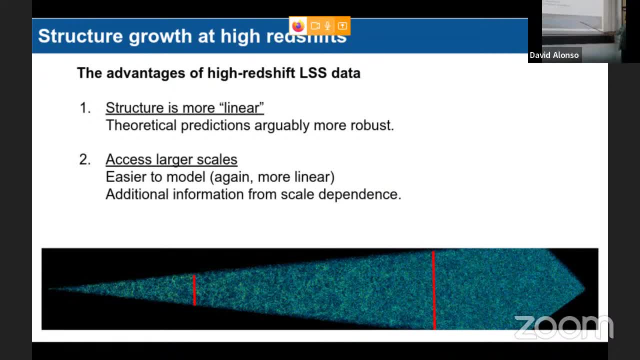 to go to high redshifts is, first of all, the structure is more linear there, so theoretical predictions are going to be more robust, and also it gives you access to larger scales. So how can we do that The way we did it in this paper? 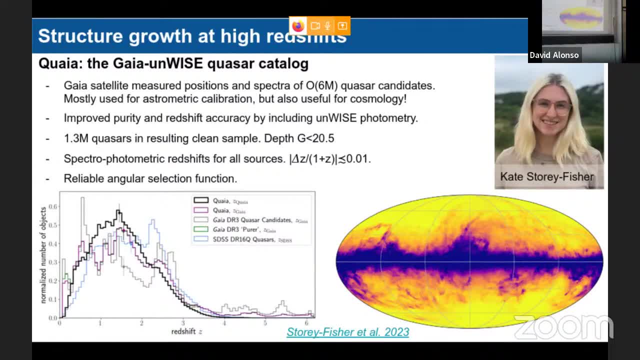 is looking at quasars at high redshifts. In particular, we used a catalogue of quasars derived from the Gaia data release, So Gaia actually measures the positions of a lot of quasars or candidates for quasars. 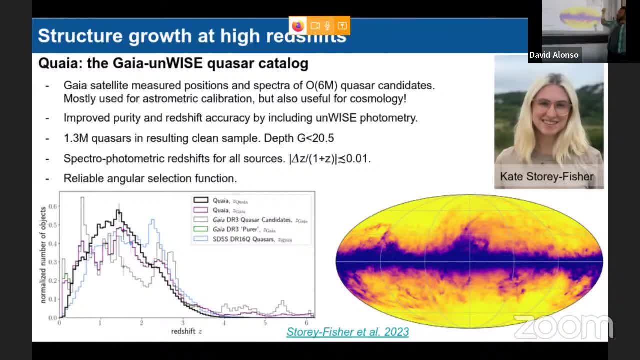 about 6 million of them. Not only that, but it actually measures the redshifts of those quasars. But usually they don't care about them because they're mostly used. they care about them for astromatic calibration, but not necessarily for cosmology. 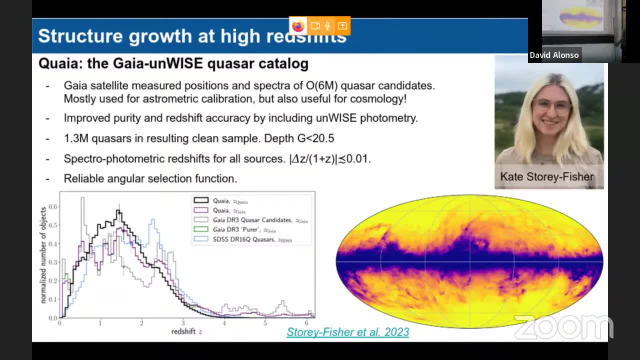 So what Kate Story Fisher did was trying to extract a clean cosmological sample from those quasars, and what she did for that is basically combining the Gaia data with photometers from the unwise infrared catalogue, which allows you to solve two things. 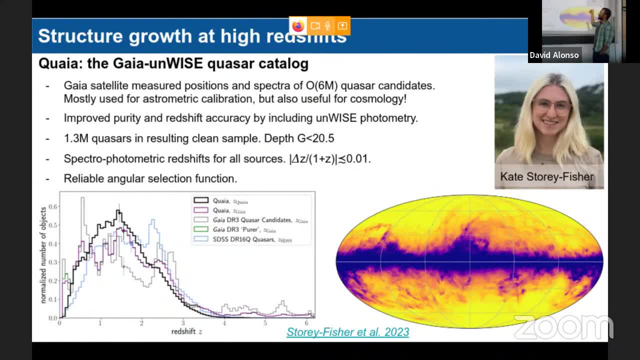 First remove quasar candidates that are suspicious and also improve the redshift accuracy of these quasars. So in Gaia you do have spectroscopic redshifts for some of these quasars, but there's lots of interlopers and wrong redshifts there. 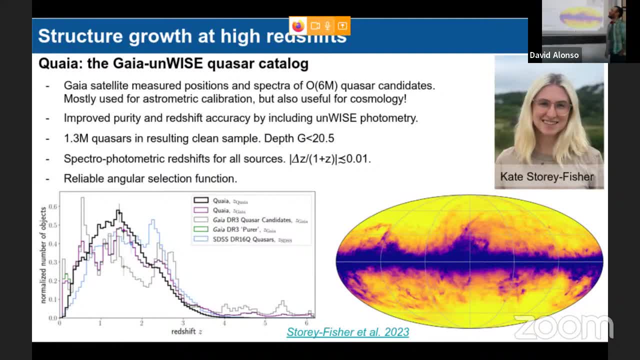 So you can clean them up by looking at the photometer. The result is this catalogue called Quelia, which has about 1.3 million quasars And it's an extremely clean sample. It's a sample where you understand the transfer function really well. 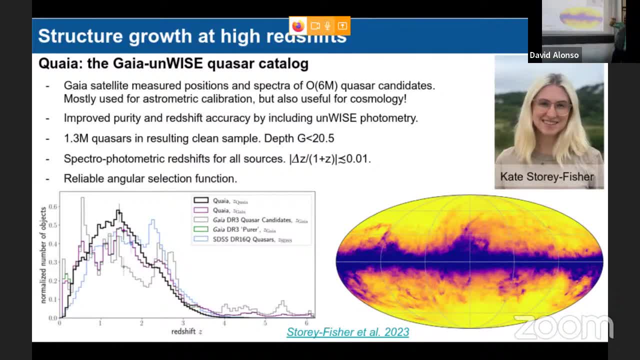 So basically you understand very well any systematic variation in the angular distribution of these quasars by virtue of Gaia being a space satellite and the techniques that we use here to characterize that transfer function, And also you have very decent photometric redshifts. 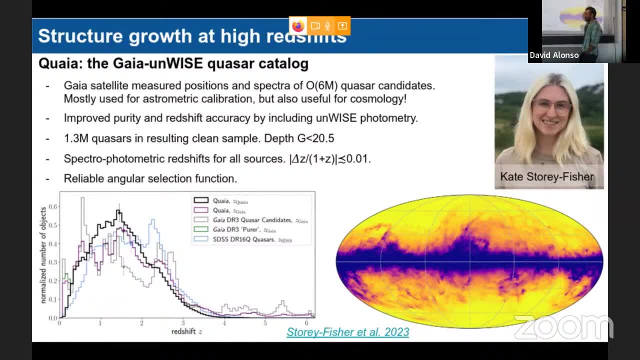 for all of these quasars, because you have the spectra from Gaia as well And, most importantly, the catalogue goes all the way to redshifts of about four, So we can try to get a measurement of the amplitude of metaflaturation. 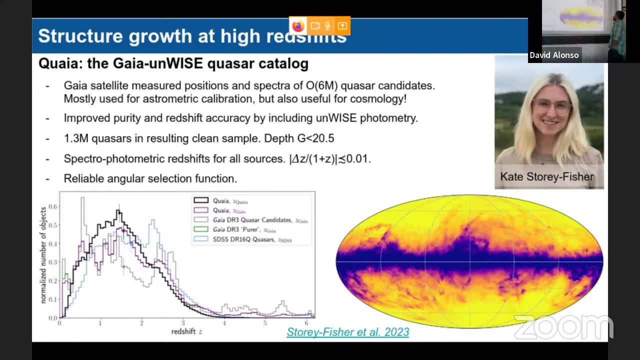 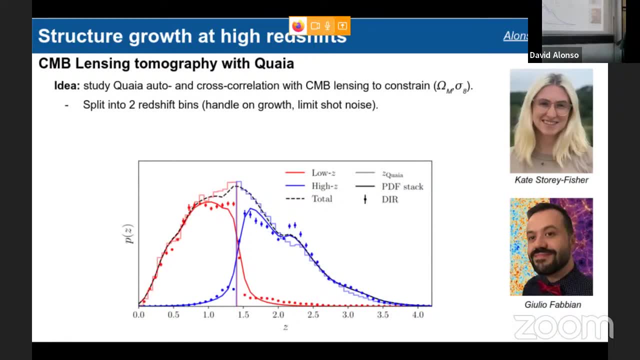 at very high redshifts and see what that does, Right. So what we did is we looked at the kind of the two times two point thing where the part of that came from rather than from here. So what we did is we took Quelia. 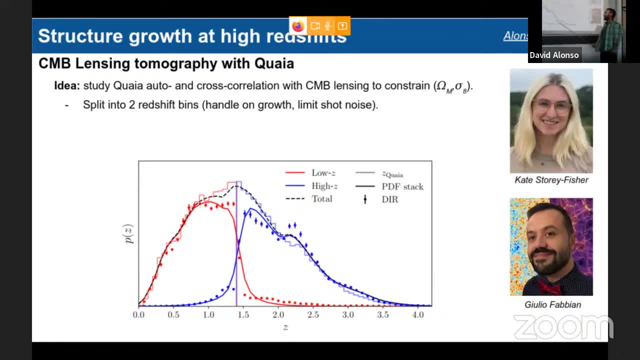 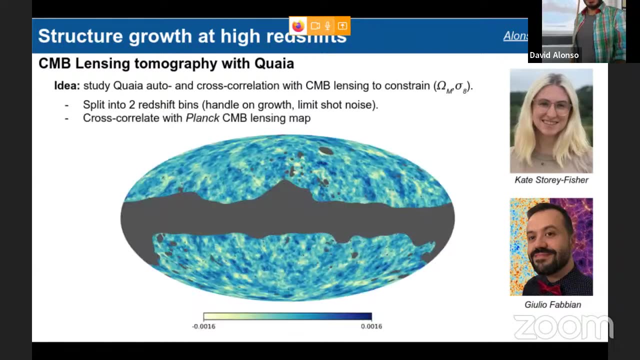 together with Julio Fabiani- Some of you know him- We split that into two redshift bins To get some sense of the growth of structure of the redshift. And then we looked at all the out and thrust correlations between that and CMB lensing. 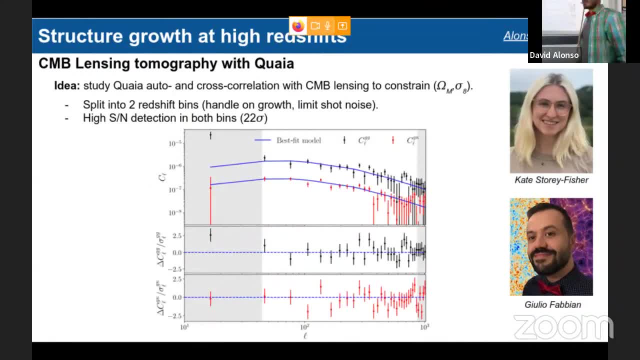 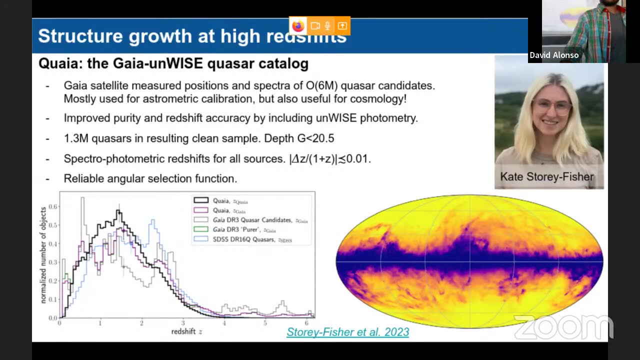 So that's the CMB lensing map And these spectroscopic measurements- are they from Gaia? Yeah, So you have a spectroscopic redshift for all of these quasars from Gaia, But it is often wrong. So in the end, what you have is: 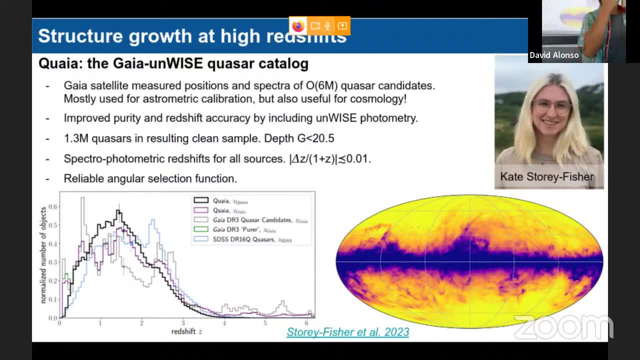 a spectrophotometric redshift for all of these sources that combines whatever photometry exists in Gaia, whatever photometry exists in UNWISE, whatever spectrum information exists in Gaia and a training sample from quasars in SDSS to figure out the redshift. 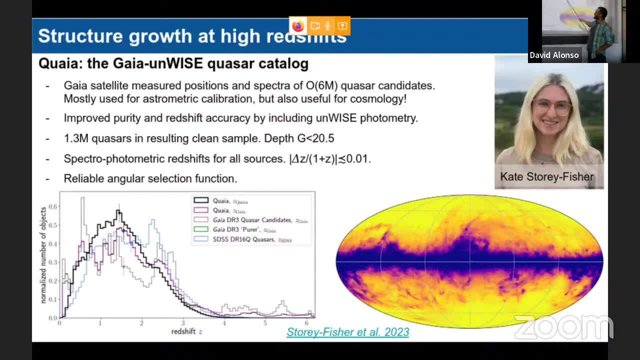 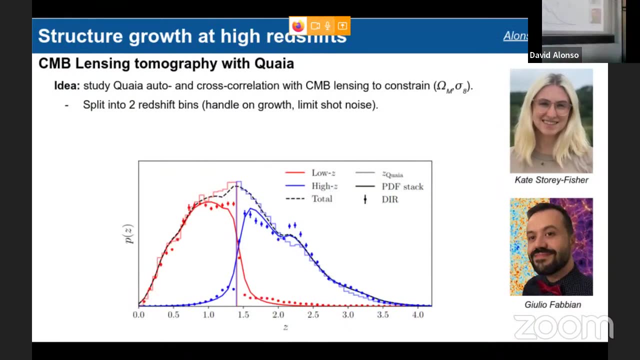 So very often they're not very precise, But substantially more precise than almost any photometric sample that is redshifted, certainly for such a wide catalog. So we have a good understanding of the redshift distribution, for example for these places Cool. So these are, for example: 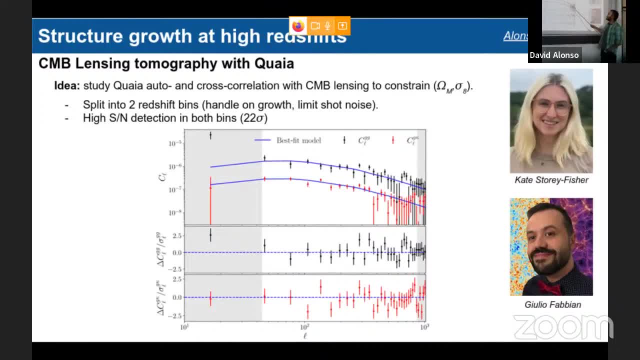 the autocorrelation, the quasar autocorrelation and the cross correlation with CMB lensing. And the cross correlation with CMB lensing is actually detected at very high significance, but at higher significance than the autocorrelation of the quasars. 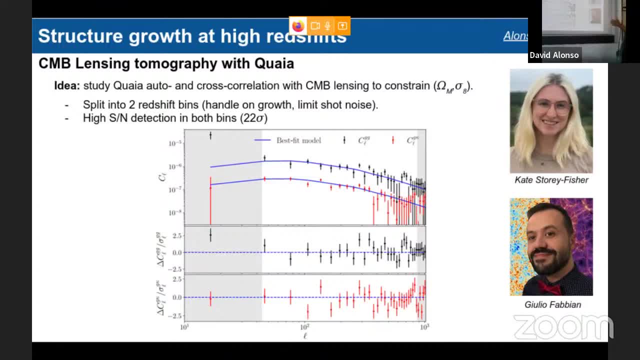 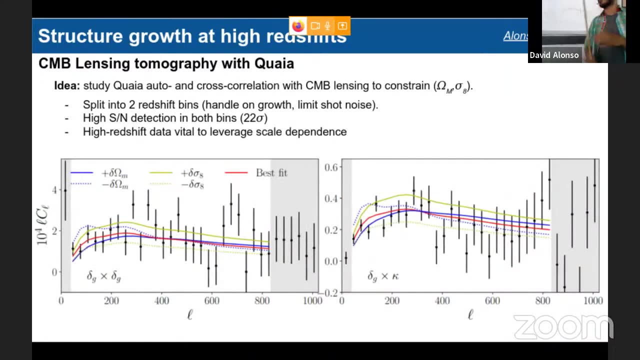 Of the quasars themselves. So the fact that you're sensitive to fluctuations at very high redshifts makes CMB lensing extremely useful here, Right? so with this I can actually illustrate why going to high redshifts is nice. So what I'm showing here 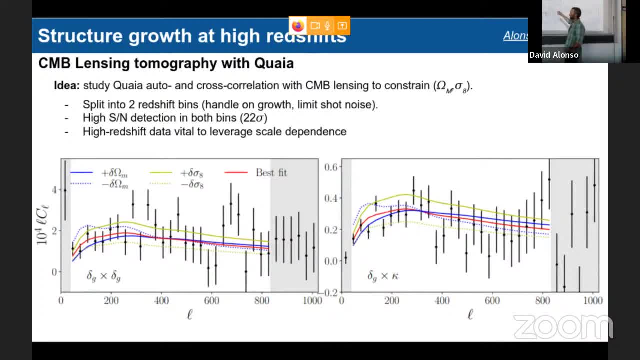 is for the higher of the two redshift pins- the galaxy autocorrelation on the left hand side and the cross correlation with CMB lensing, And for each of them you have a red line which is the best fit. prediction from Landa-Sedien. 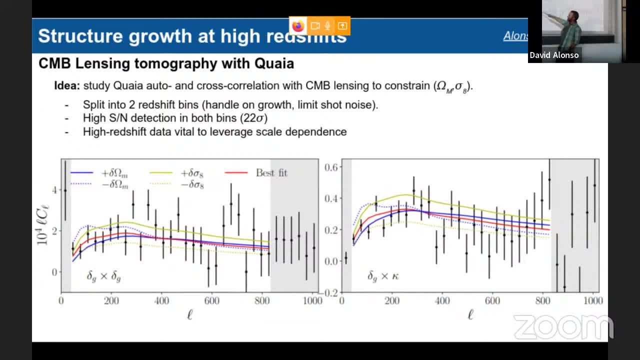 And then in blue, what I've done is I've shifted a little bit omega-m or sigma-8.. If you only had access to the smaller scales- which is what you do when you're looking at much lower redshifts, because all of these filter out of your data. 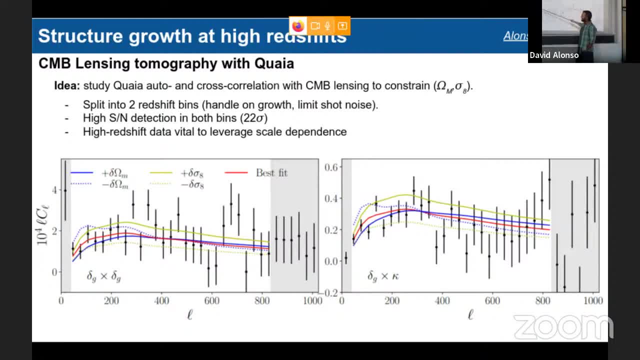 the impact of varying omega-m or sigma-8 is basically the same, just changes roughly the amplitude at this scale And that's the main reason why you have this banana shape in many of these analogies. If you have access to the larger scales, which are also more linear. 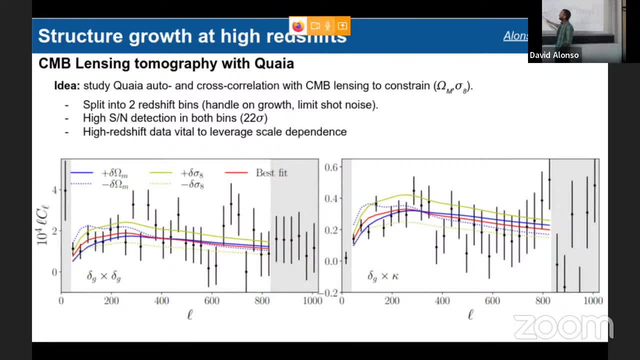 then you start picking up the scale dependent impact of omega-m, for example. So omega-m actually changes the tilt at low cases, large scales. So you can actually break the degeneracy between these two parameters by looking at high redshifts And you actually no longer measure. 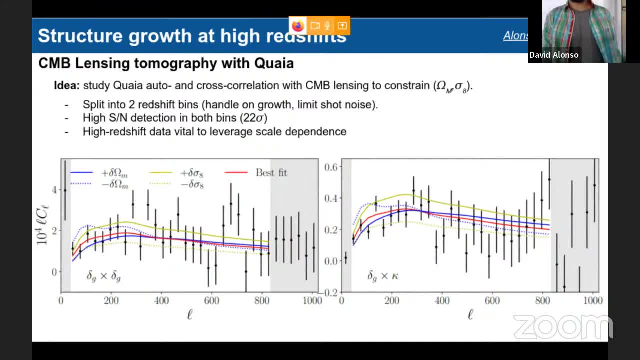 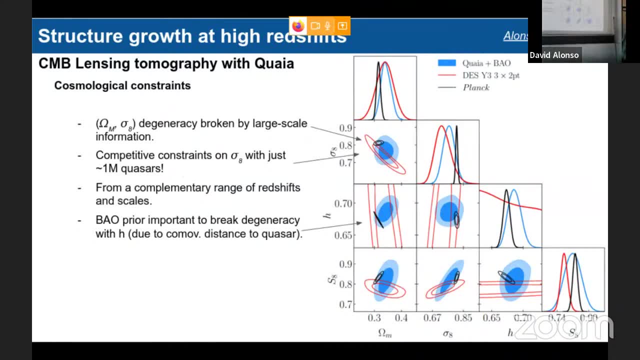 just S8. You can actually measure both of them separately. So this is the main result. Yes, So I think that's the best way of understanding basically that it shifts the position of the quality peaks, basically, and that changes the effective slope of the power spectrum. 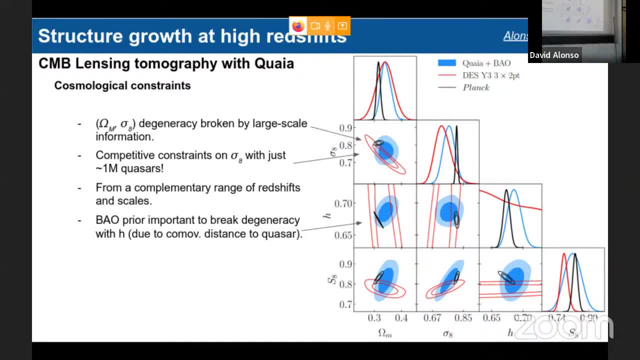 at the VAO-like scale. The one thing we're trying to do now is actually make a detection of the quality fail with this data, which I think should be possible, But it's tricky because you really need to measure the clustering on the really. 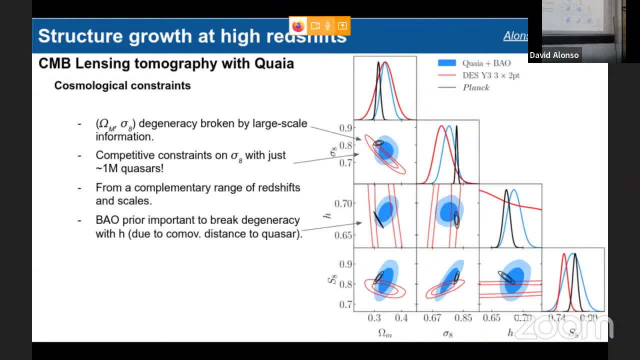 really large scales and ensure that there's no systematic there. So that's what we're working on right now, Anyway. so these are the cosmological constraints. I think the best block to look at is here. So this is sigma-8 on the y-axis. 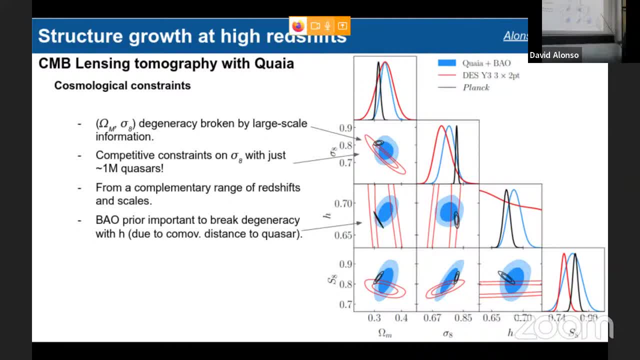 and omega-m on the x-axis And our results are in blue. The constraints from, for example, the latest and largest 3x2-point sample that we have from DES are in red And you can see that 3x2-point weak lens. 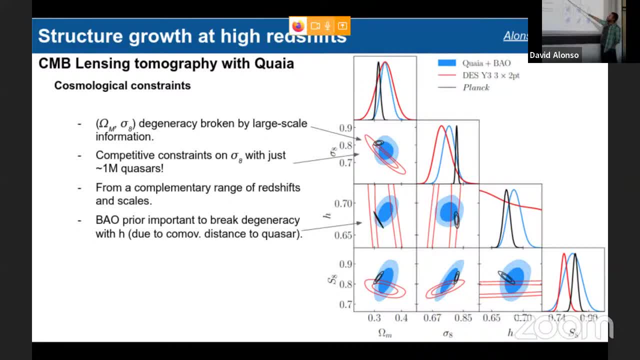 in this cosmic series is really good at measuring S8, but really bad at measuring any of these parameters independently, whereas we get basically better measurements of both of them separately with just a million quasars. So this is just to highlight the benefits of going to high-res. 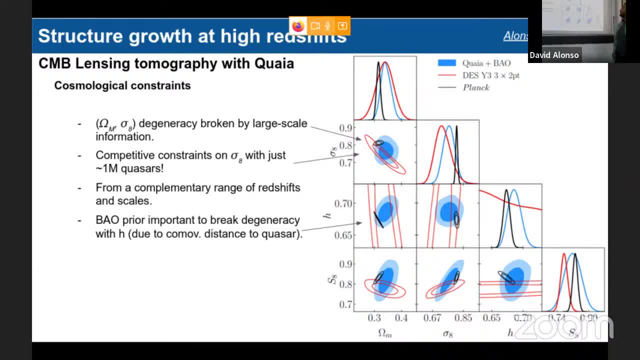 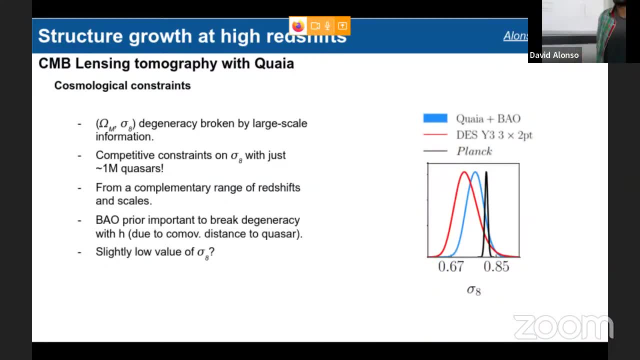 and large scales. Yes. Now, if I just look at sigma-8 for a second, and just for the sake of going with the times and keeping an eye on this S8 tension, we do measure a value of S sigma-8 that is very compatible with Planck. 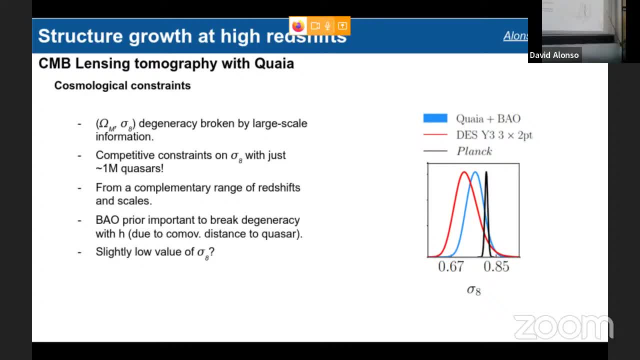 but it's on the low side of Planck right. It's still 1.5 sigma, I think, or 1.6 sigma-8 with Planck. It wouldn't be suspicious otherwise, but we're talking about these consistently. 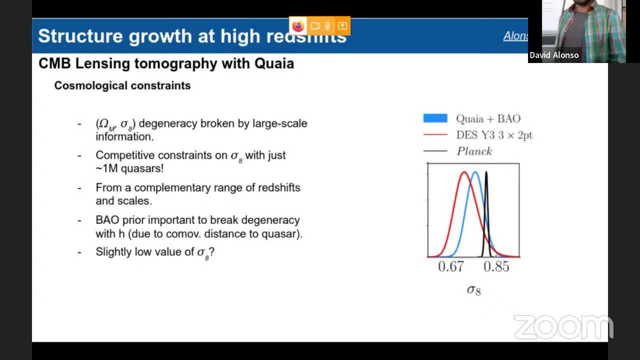 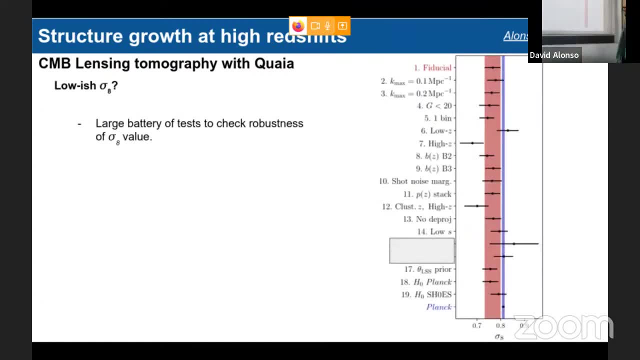 low values of sigma-8. Or S8.. Maybe it's worth looking at it a little bit more. We did lots of different checks for potential systematics And what we saw was the following. So here I'm just focusing on the sigma-8 value. 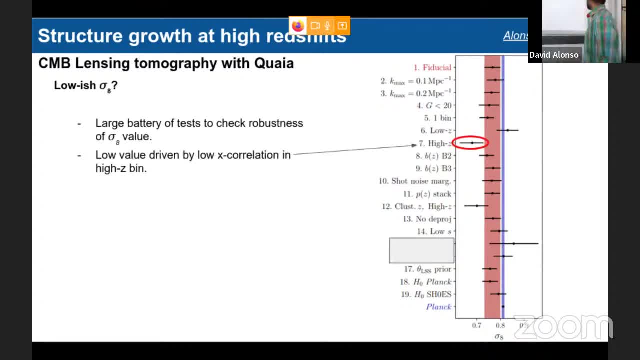 What we saw was the following. So it seems like if we split the analysis into just looking at the low-res chipping or just looking at the high-res chipping, it's actually the high-res chipping that gives you a low value of sigma-8.. 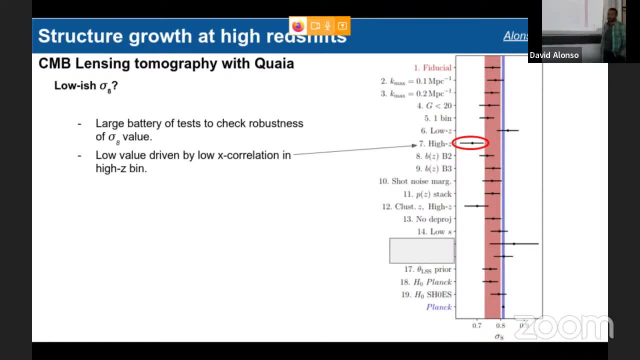 That made us very worried. So we focused a lot of our tests on Qualla and seeing whether any of those potential social systematics could move that result And none of them did, So I'm not going to go through them If you have any questions about things. 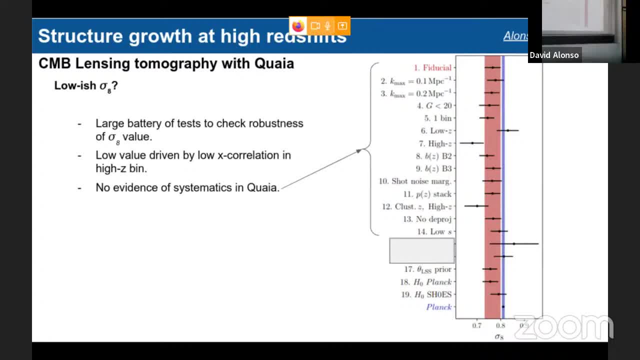 that maybe we didn't check. I can walk you over everything we did. There was nothing in Qualla that could actually explain this. So what we saw is that, actually, looking at the potential systematics in the CMB lensing map, which is the cleaner one? 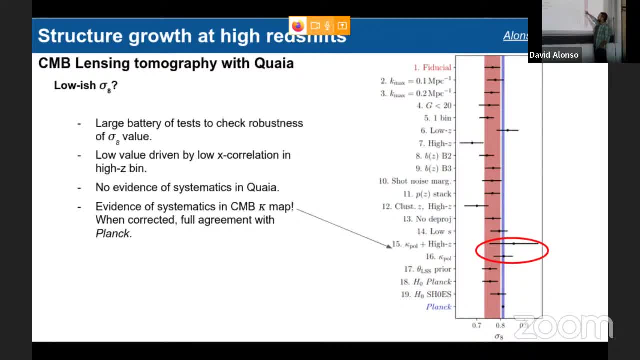 this actually reveals a potential systematic that would shift the clustering in the high-res chipping to something that is completely compatible with this one, And so our interpretation of this. and there's several reasons why this is probably correct, and I can walk you through those. 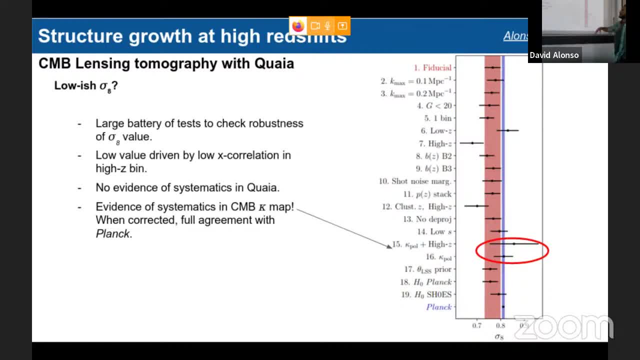 is that this is contamination from the cosmic infrared background in the CMB lensing map, which is known, if it was there, would cause a low shift in sigma-8 like this, But which you know, the assumption was that that level of contamination. 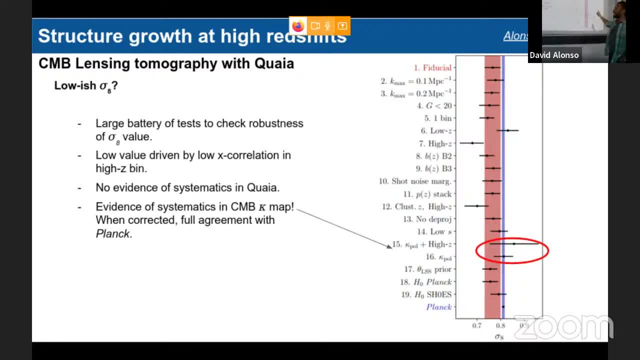 was a lot lower in the CMB lensing map, But you are not able to see this unless you're able to look at cross-relations with things that are as high-res chipped as Qualla. But the CMB came up with this unwise. 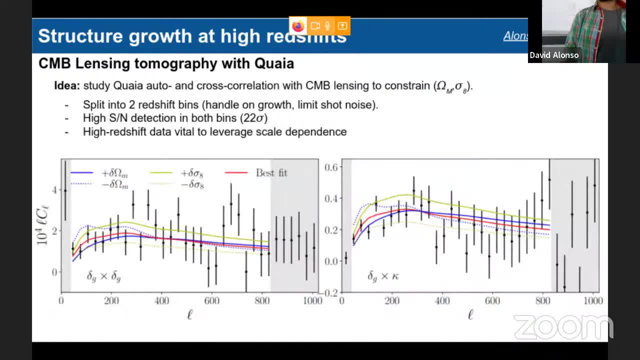 Yeah, But unwise doesn't. if you look at the redshift distribution of unwise, it goes. it doesn't go to as far as high redshifts as basically, So the mean redshift is about 1.5.. 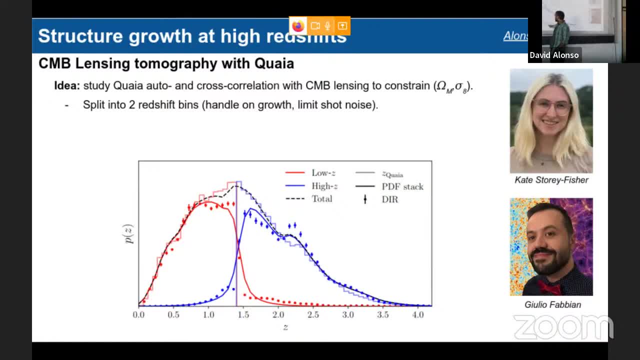 What we're seeing is that actually you pick up a system that is consistently at about between redshift 2 and 2.5, which is also where the peak of star formation happens. So, CIB, a lot of the CIB comes from those redshifts. 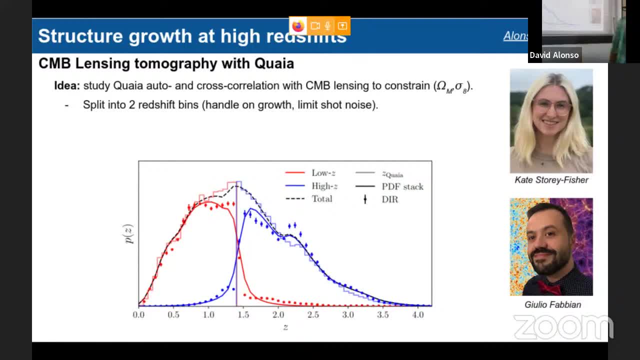 basically. So you're saying that the unwise plus CMB lensing is not affected by this? It could be. We haven't done the analysis. Also, the CMB lensing is not affected by this. So what we did, which people haven't done before, 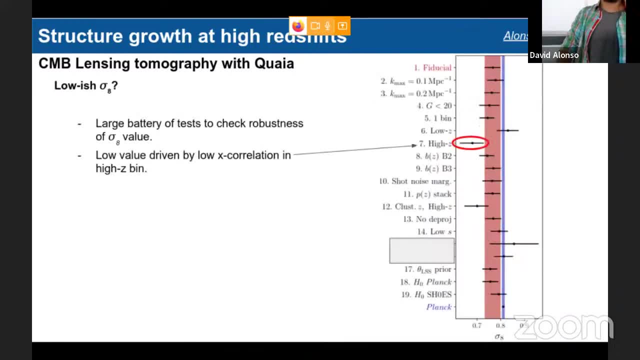 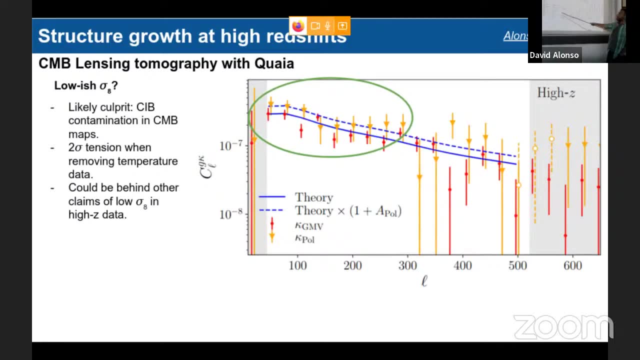 is. we looked at cross correlations. I'll show you this. then We looked at cross correlations between the high redshift sample and a CMB lensing map that is constructed using only polarization data in the CMB, So polarized. the CMB is completely unpolarized. 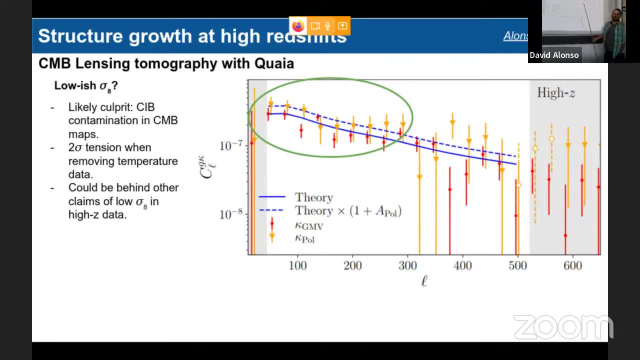 The CIB is completely unpolarized, so it wouldn't show up in this map, And what we see is a two-sigma consistent shift upwards of all this, of all these redshifts. So we can see that the CMB is completely unpolarized. 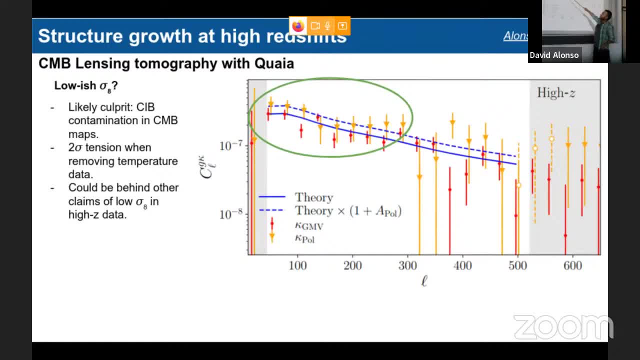 The CIB is completely unpolarized so it wouldn't show up in this map, And what we see is a two-sigma consistent shift of all these correlations: for the higher redshift, So at low redshift. you don't really see that. 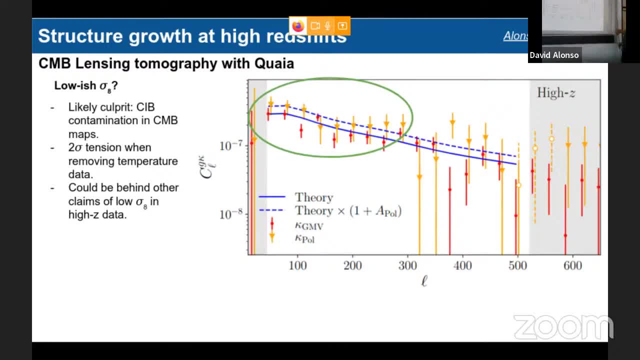 It's only if you do like a sliding cross correlation at different redshifts, you see that it pops up at redshift two And there's two-sigma evidence. You can do an even cleaner map using polarized, using polarization. 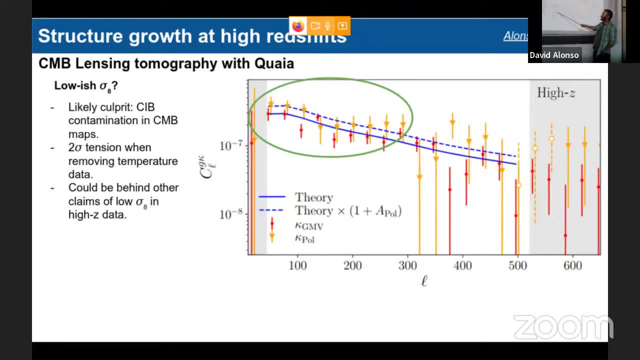 but also cross correlations between polarization and temperature, without looking at the temperature-to-temperature correlation. That would also be immune to the CIB contamination, And this is actually something that we did in the CMB. So we can see that the CMB is completely unpolarized. 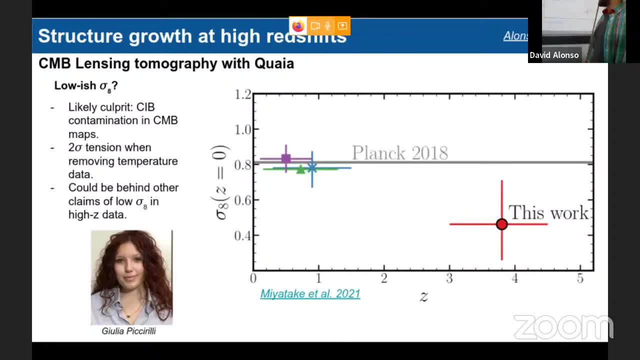 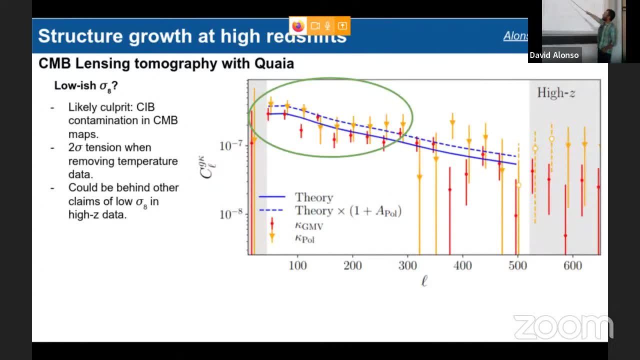 in this map. This is something that a student is looking at, Julia, particularly with us now. So this is unpublished stuff And it shows that. It shows that this evidence for a systematic that shows up at about redshift two goes from two-sigma. 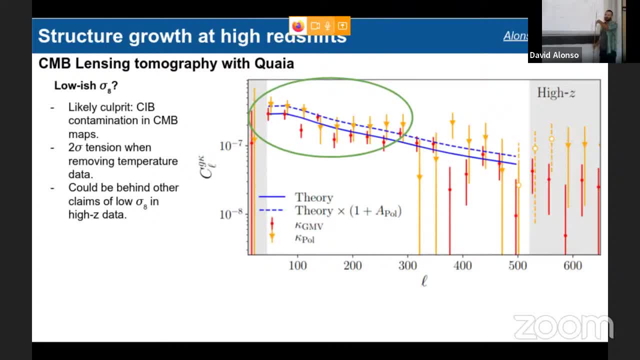 to more like three-sigma, three-by-five-sigma, So I think that would be probably correct. Yeah, But anyway. so once you use a cleaner CMB lensing map to look at the high redshift sample, the construction of this map. 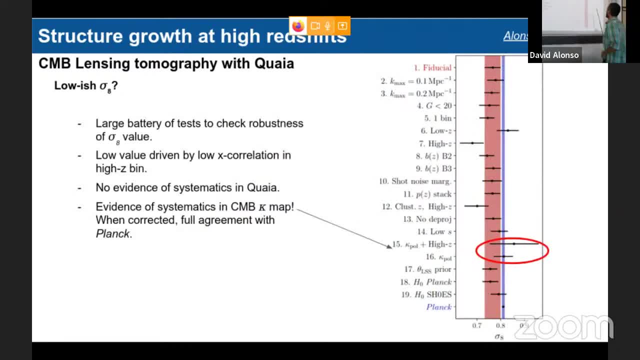 is pretty much the same, but the constraints become completely compatible with this line. so that is the final number without having lost much of the sensitivity. All right, So the main conclusion is, when you look at large scales and high redshifts, results seem to be: 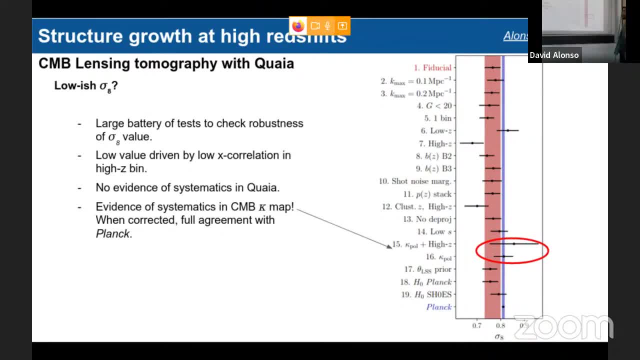 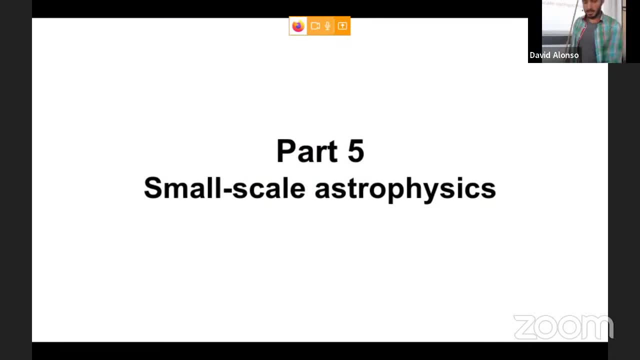 in good agreement with this line. Okay, All right. So the other option I mentioned: How much time do I have? Okay, So here high redshift means that you can see the high redshift in 1.5 to All the way. 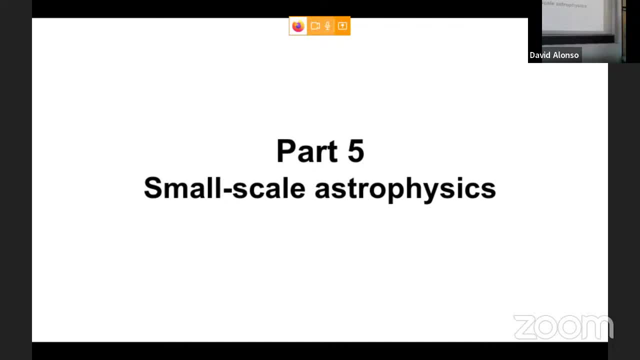 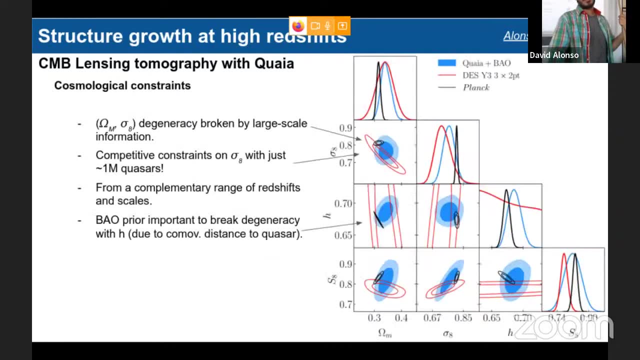 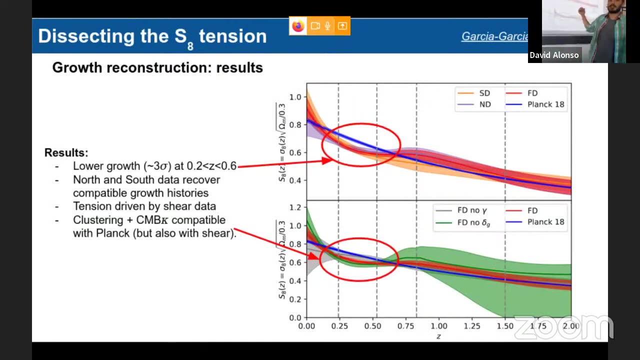 to 3, if you want, right, Yeah, Yeah, Only below 1.5.. Yeah, Yeah, Exactly. Which kind of agrees, Exactly. I think all of this data that I've been looking at are mostly sensitive to this range. 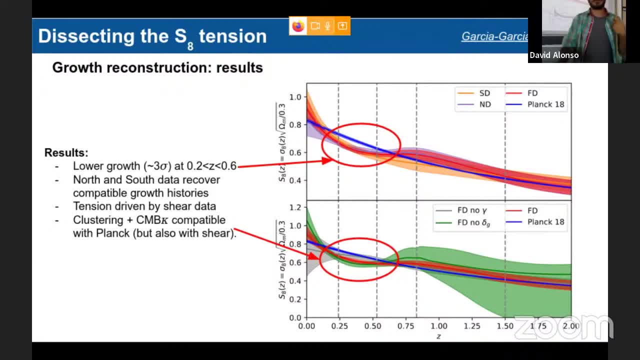 of redshift in practice, right? So it's 0.5, 0.7,, let's say, which is a little bit more than 0.5 or 100 or 100 of the same values. So this is pretty. 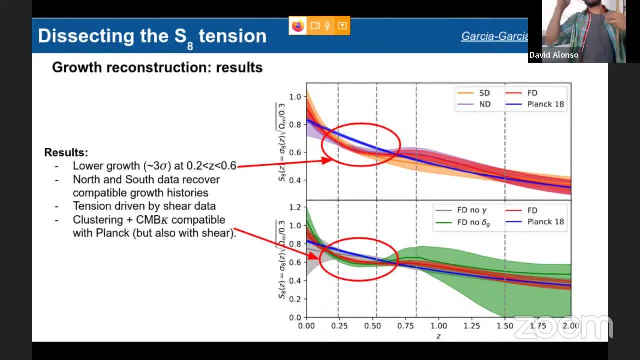 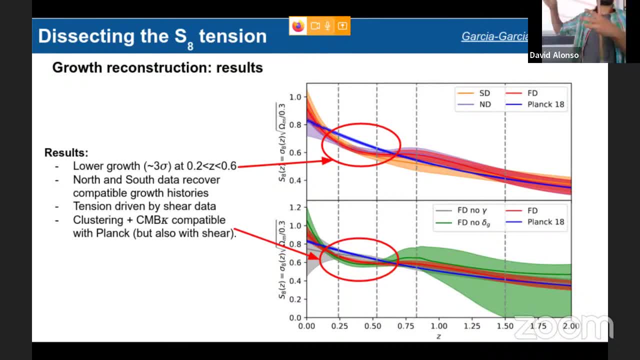 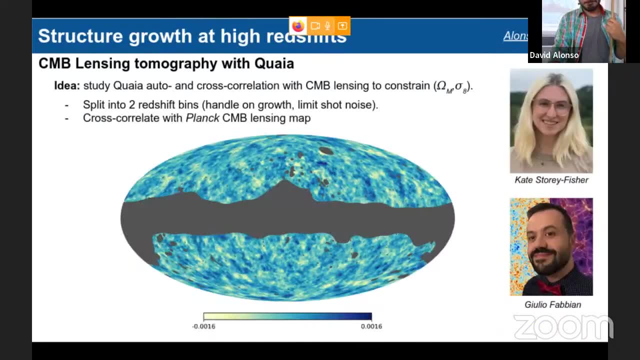 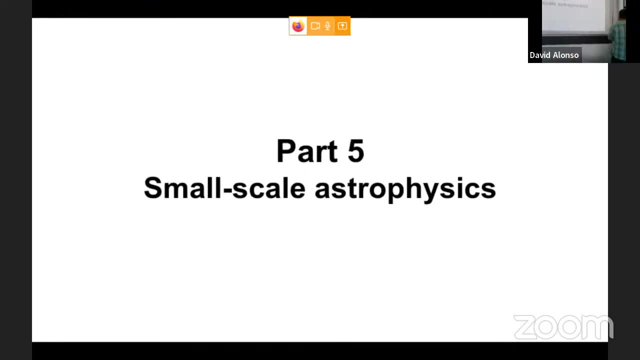 autocorrelation, and that's probably correct. you only pick it up when you, when you target the red cheese where it pops up. basically, all right, um, let me go back, um, so the the other thing, uh, the other option we said is: are there, uh, is there other data that, um, um, that can kind of help us? 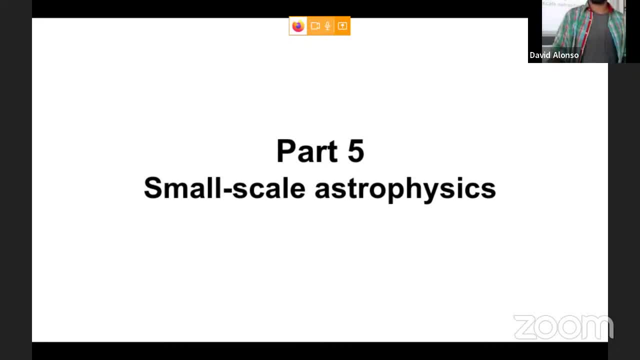 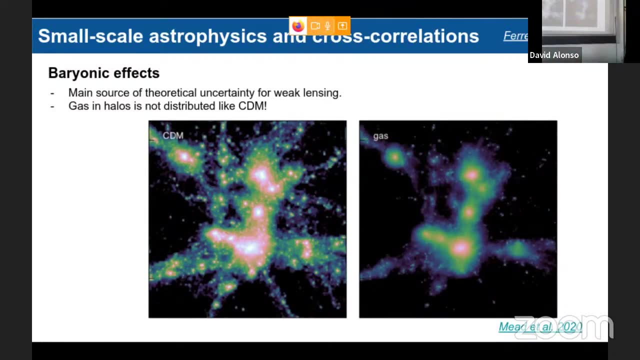 figure out whether there's something wrong with the way we're modeling the small scale structure, um and then um. the main, one of the main sources of uncertainty on small scales, i would argue, is: is the the impact of what we call baryonic effects? uh, in the glancing um and so bionic? 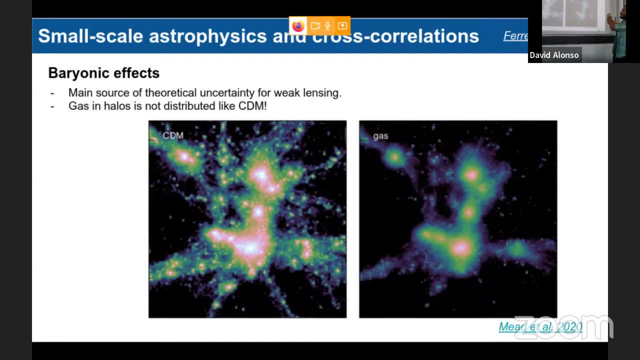 effect is basically the idea that, uh, the gas part, so the bionic part of the matter, fluctuations doesn't really fluctuate in the same way that that, um, that the cold dark matter does. uh, because gas has pressure, um, and so you can, um, you can see the distribution of of uh. 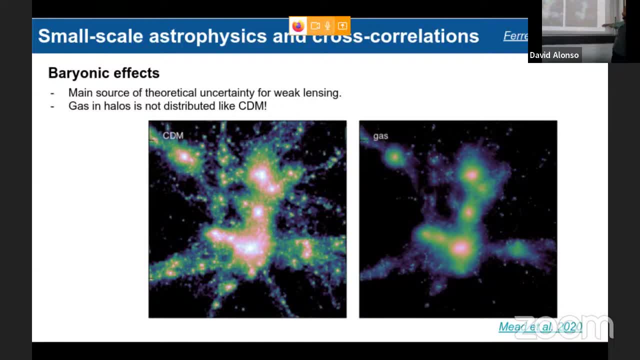 matter in the form of polar matter or gas here from the bahamas simulation. this is a paper by by alex and killman actually, um, so actually i'm sure that a lot of you guys have worked on this, so i'm i think i'm actually a junior in in this aspect, so so i i'm very happy to discuss, uh. 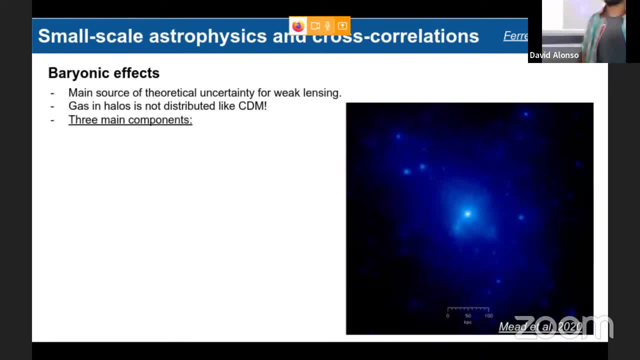 bionic effects with anyone um all right. so, so if we, but if we build the crude model for the, for the um bionic part of the of the matter, fluctuations, um we can, we can think of the three main components for, for how gas um distributes itself in in halos um, so there's the. 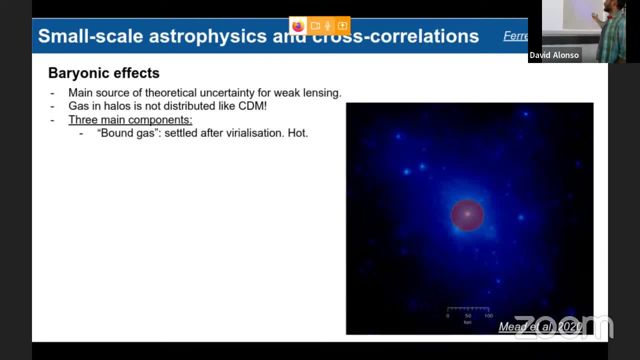 what we call the bound gas, right, so the gas that has settled down around the halo after realization, which is usually relatively hot, uh, there's the gas ejected by- by, for example, apn outflows um, which is it's farther away, less dense and usually colder, and then some some of the total amount of variance will be in the form of stars, but 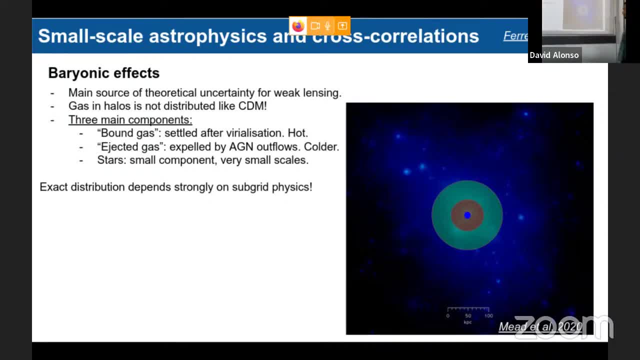 that component is usually quite small and mostly affects you on, uh, relatively small scales. so, for the much smaller scale than what i've been talking about so far. so so i you know, in principle we can ignore it, um, um. so the actual distribution of all these components, um, and therefore the impact that 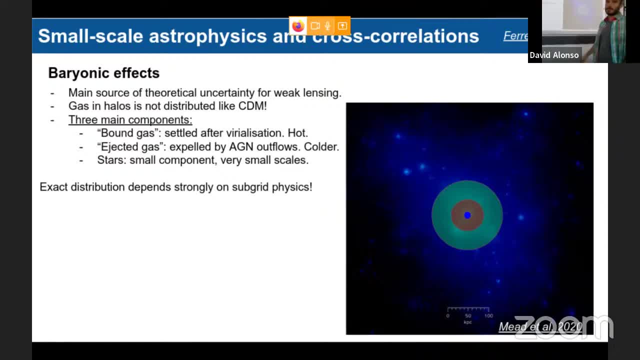 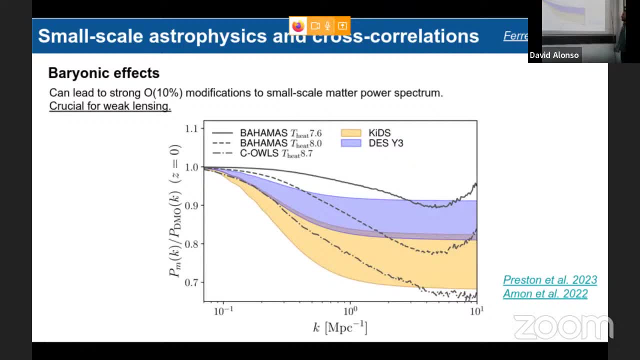 that's going to have on the statistics of the matter. fluctuation depends a lot on subject physics, um to to this kind of extent. so what what this plot is showing is the um is the level of suppression in the matter of our section caused by bionic effects in the y-axis. so one means you get the same clustering as in a in 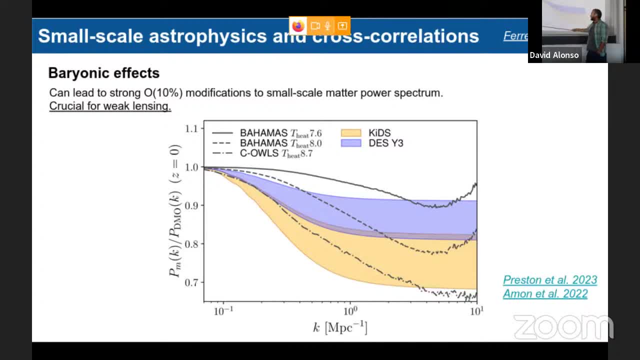 an embodied simulation that has just dark matter, um, as a margin of scales, with small scales here. right, so this is earlier stage, um, and so we have predictions from different hydro simulations, uh, just bahamas and owls models, um, and then the level of uncertainty we currently have. 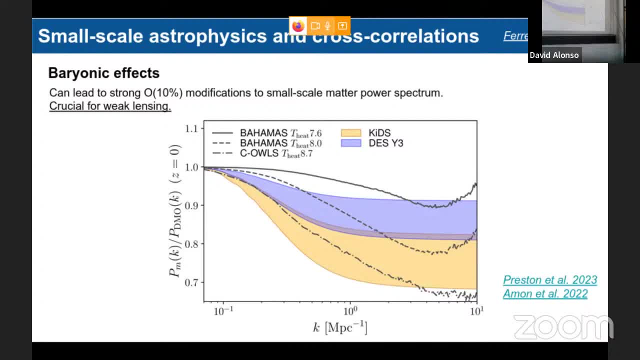 on that uh level of suppression from jessica's mixture data. so this is for those who are familiar with the work. this is the work of alex saymon and collaborators, um, but you know, it's kind of consistent between different analysis churches, um, so this is one of my main forces of uncertainty. 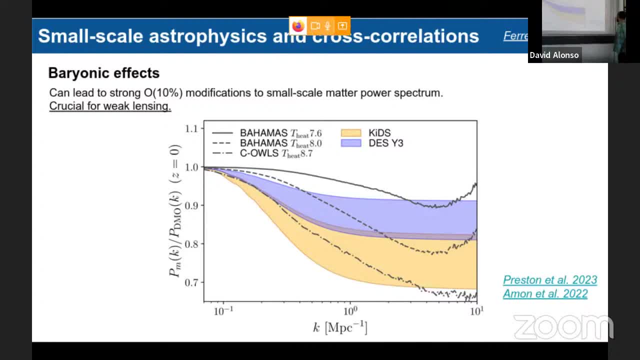 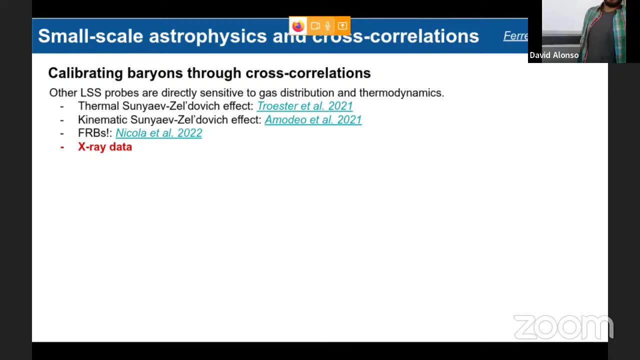 um, and it's rather crucial for for cosmology from public dancing, so, um. so the question is: um? is there other data that can give us more information about um, uh? what bionic effects should be doing um, um? so the answer is yes, there's, uh. there's large structure probes, um, beyond those that i've. 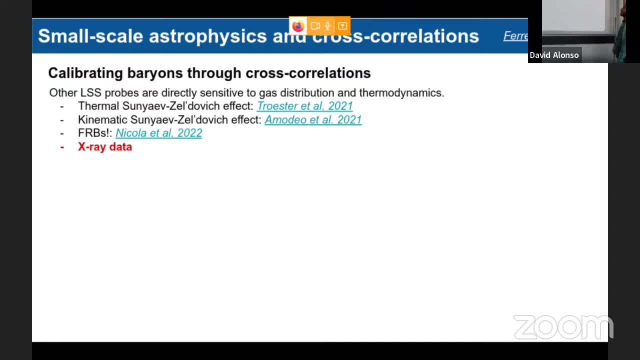 discussed so so far, that are directly sensitive to the gas distribution, so you can use those to figure out what the gas is doing, and so the obvious one are the thermals in the absolute which, uh, tillman has has, uh, um, in the past, um, uh, there's a kinematics, and yes, which, in principle, 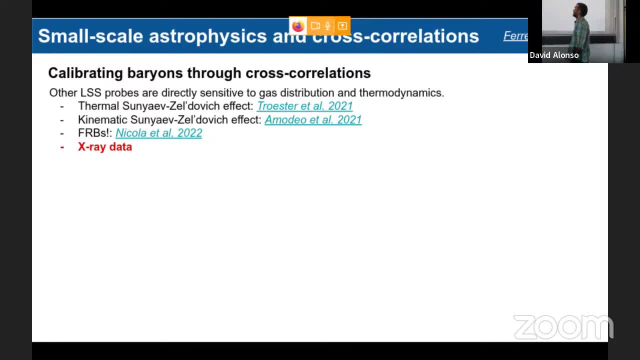 is directly sensitive to the distribution of gas, although it's a very difficult measurement to make. um, people have even suggested using frbs as a probe of the, of the, you know, the electron distribution, therefore the gas distribution in the, in the ibm, and- and what i'm going to talk about now is x-ray data. 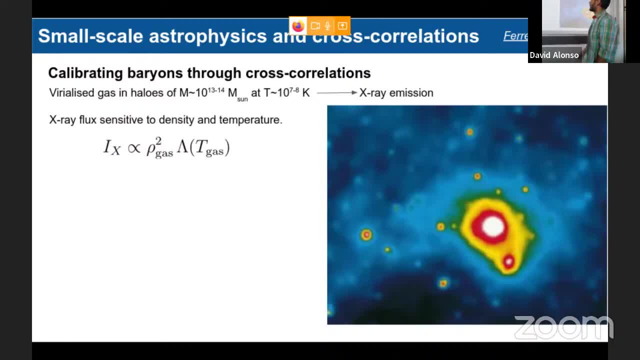 um, so the idea from a kind of back of the envelope calculation, is, if you have a halo of about 10 to the 13th to 10 to 14 solar masses, the uh virial temperature for such a halo would be at the level of 10 to the 7 to 10 to the 8th kelvin, which means that it should emit. 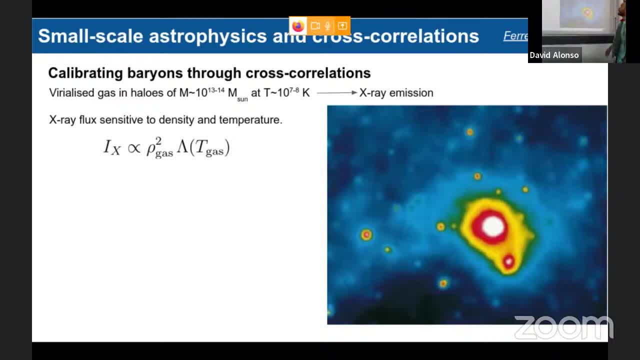 x-rays okay, roughly um. x-ray emission is mostly caused by collisional processes. so x-ray, the x-ray intensity, is going to be proportional to the density squared of the gas and then some function of the temperature of that gas, so that this is usually called the cooling function. there's many 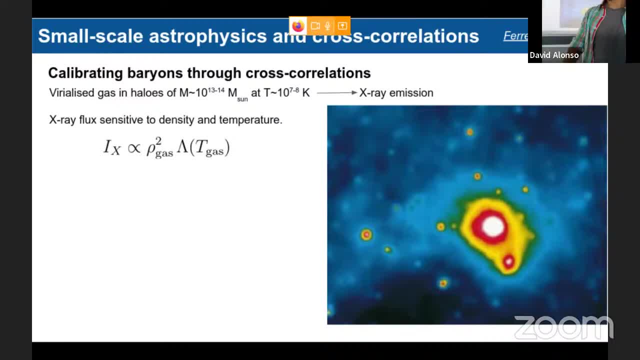 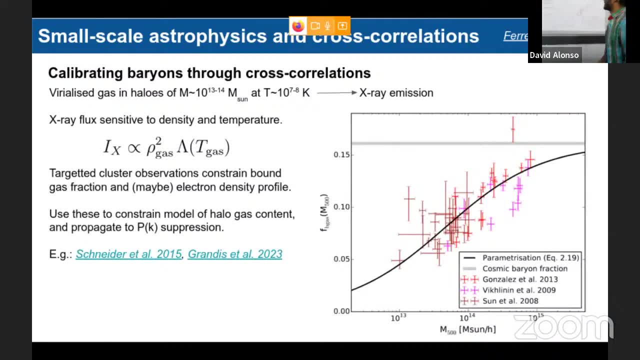 names for that, for that function, um. but the idea is that it's sensitive to these, to these two properties of the of the gas. so one way in which you can use um x-ray data to to say something about um, about the distribution of gas in halos, is by looking for. 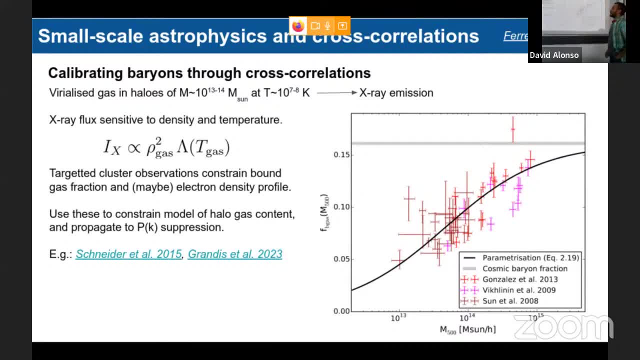 example of targeted x-rays: x-ray observations of clusters, which, for example, tells you about how much of the total um fraction of gas mass is bound versus ejected, for example. or or also measurements of the electron density profile from from- yeah, from from- x-ray observations, and i think people here have actually done a lot of work. 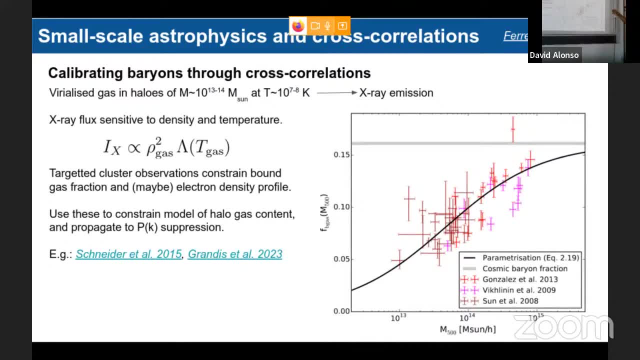 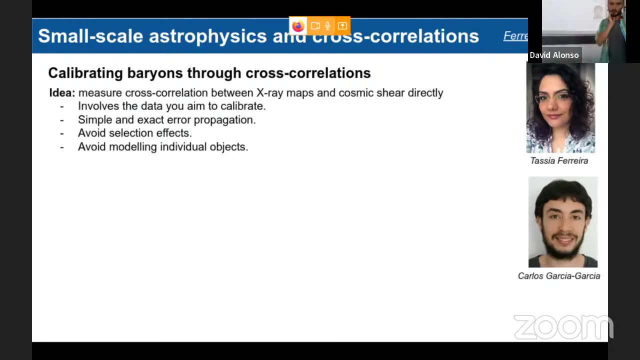 combining these with cosmic shear, um, uh data or using it to constrain the level of irony effects in cosmic here. so giovanni is one of them, um, um, so that that's what's one possibility. what we did in in this paper was, uh, taking a different approach. so, um, what we did is trying to directly. 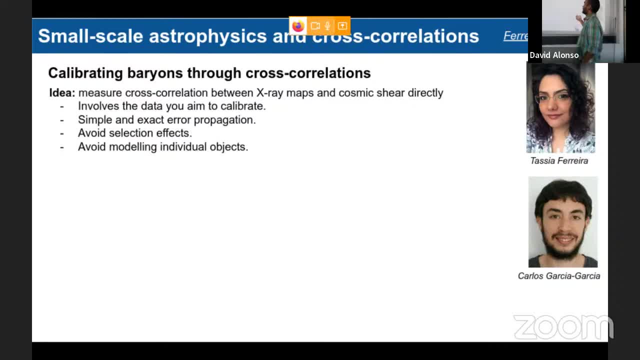 measure the cross-correlation between all the diffuse x-ray emission in a full sky x-ray map and the cosmic shear data and just look at that cross correlation as a probe of of the of the distribution of variance. and so the advantages of doing that is that it directly involves the data that you're. 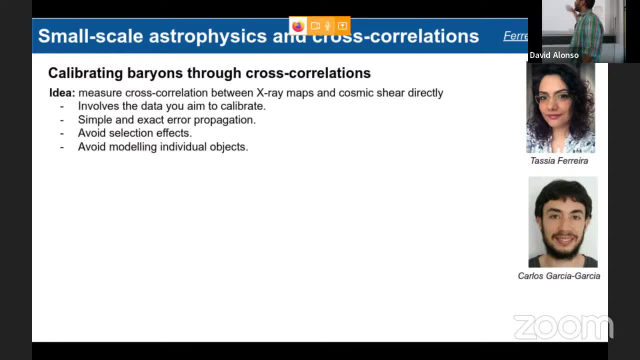 going to calibrate, which is the cosmic shear data. um, it uses exactly the same data analysis methods that we use to do 310 two-point analysis or any any cross-collation based analysis. so so that means that error propagation is is extremely simple and exact. 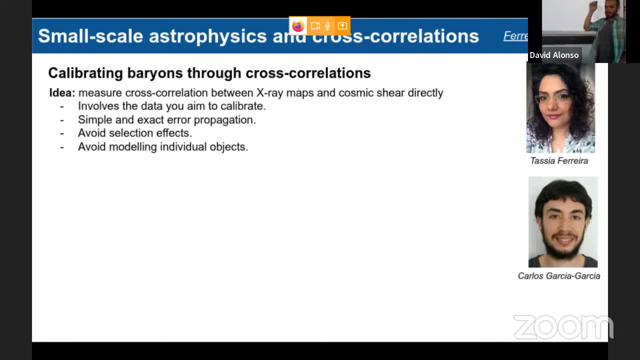 um. you avoid selection effects um because you're not targeting a specific set of of of uh clusters, um of a given mass or anything like that. you just look at all the combined x-ray emission and you don't need to. it doesn't rely on the modeling of specific individual objects. 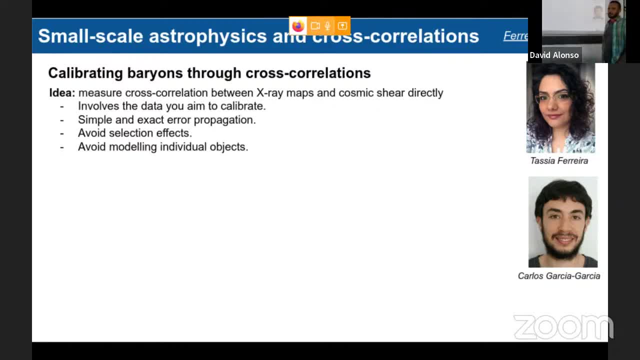 um, which which can be quite tricky, and then averaging results from individual objects. there might be uncertainties that don't really um average out um. one of the advantages that i i didn't mention before of x-ray x-ray data is, if you look at the at the contribution um. 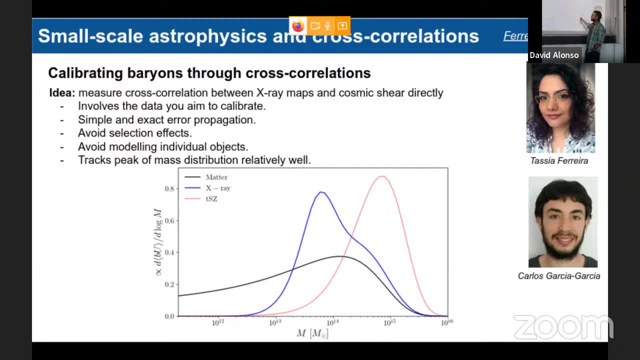 from halos of different masses to cross correlations of different sorts, right? so in black you have the matter, uh, the matter part spectrum, and how a lot of different matters contribute to the amplitude of the matter part spectrum. um, you see that most of the contribution is coming from halos between 10 to the 12th and then 14, maybe a few times. 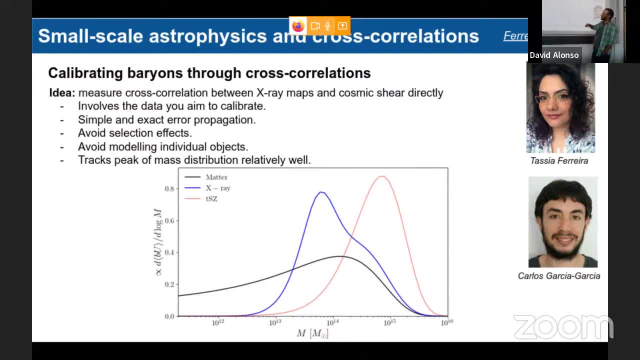 if you are looking at psx, for example, because psx scales, like masters, are five over three, uh, you're actually more sensitive to slightly higher mass scales than maybe you would like to be more sensitive to at least three behavioral factors. um, so if you, if you have UCF, um, but you 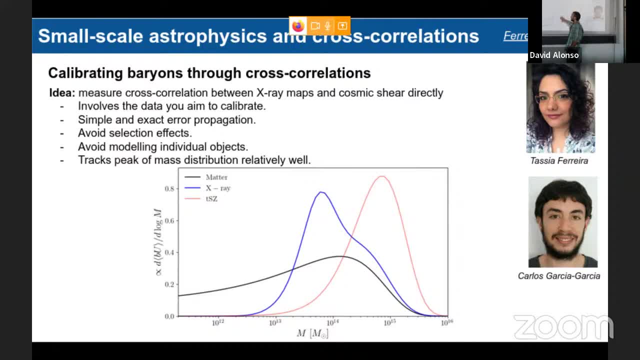 don't want to be sensitive to uh mu and all the macro desires uh, but you're more sensitive to uh the double spread of mu and so on. so, for example, if you have a maximum mass, um, you're you're more sensitive to your mass, uh, maybe x-ray data brings you back down a little bit. 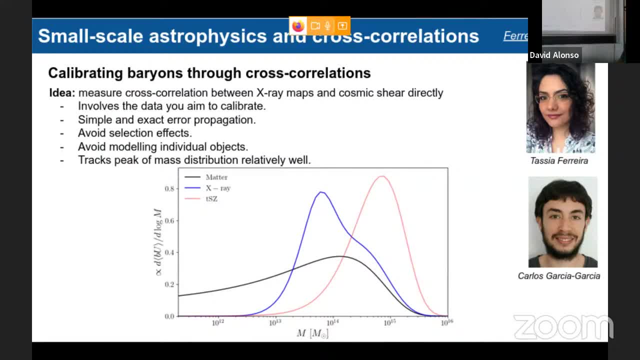 because because of how it depends on temperature, and that's it. so it actually targets halos of the masses that we kind of care about. maybe if we want something else that is able to tell us something else that is able to tell us something about the really low mass halos, but at least that'd be better, um. 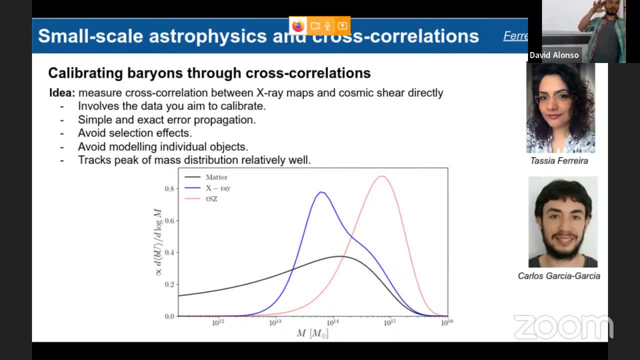 depending on the range of temperatures. that you're looking at is something that roughly goes like temperature to the one half instead of temperature, right. so tfn goes like density times temperature. so when you integrate over volume you're going to get mass from the density integrated over volume and temperature. if you look at how the virial temperature depends on mass, 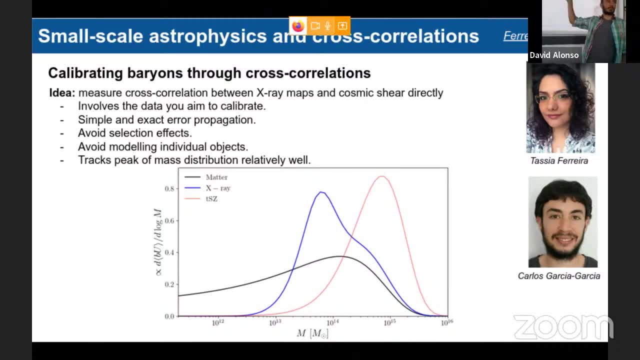 you get another power of two over three. so so you get mass to the to the five over three. here you get mass to the power of one from the density integrated over volume, even though the density squared. but that doesn't affect things. and then the temperature is. there's a weaker. 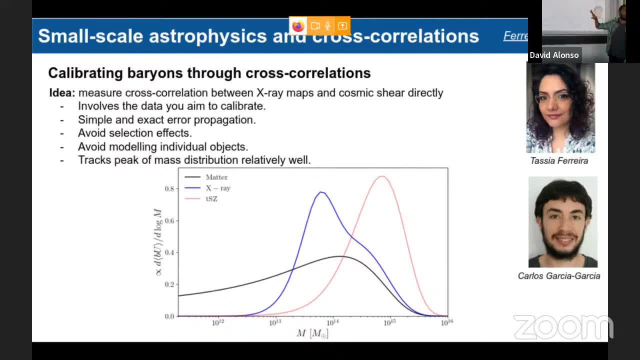 dependence on the temperature. so so it's almost proportional just to the mass. basically it's a bit a bit stronger than just the mass, but but enough that that it doesn't shift the peak massively. but but except if you go to sufficiently low masses, the gas is not hot. 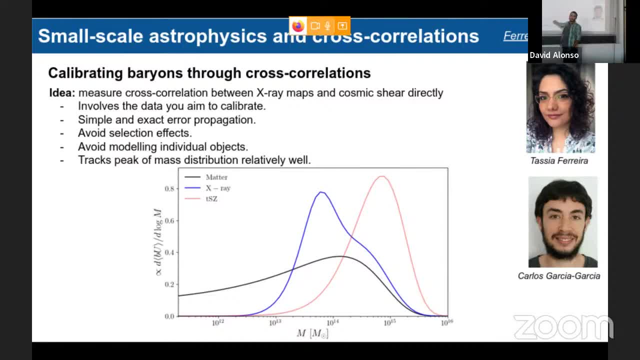 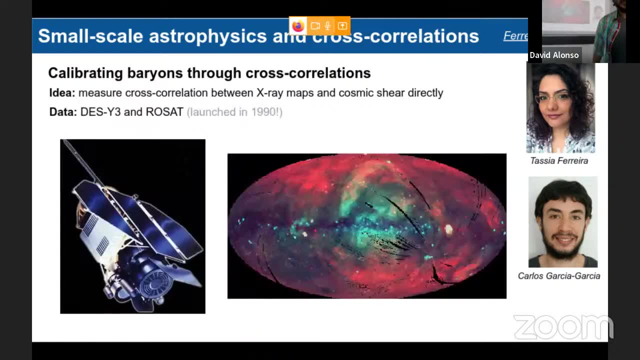 enough to actually emit in x-ray. so that's why there's this cutoff here, where you don't um right. what we did is we, we cross-correlated um, a cosmic shear from um ds and x-ray map, full sky x-ray data- sorry from rosa, which is a satellite, a german satellite that was launched in 1990, so it's almost. 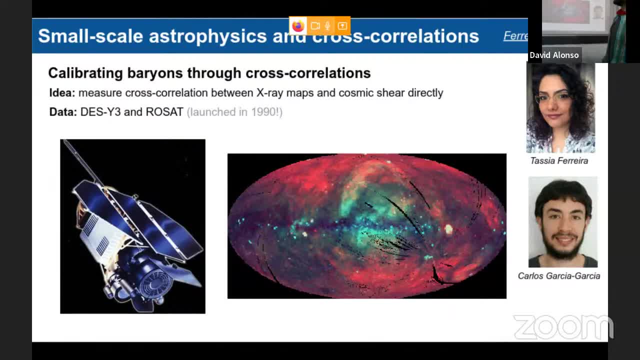 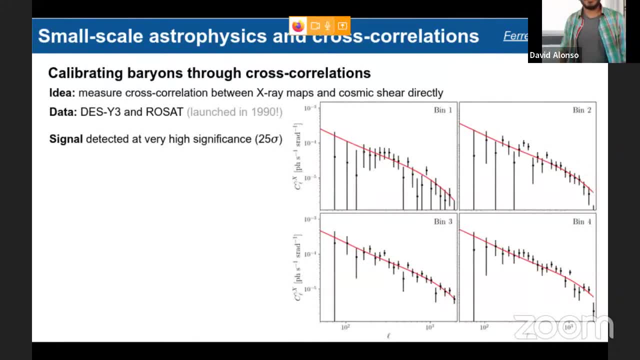 as old as um uh, so it was a lot of fun to actually analyze this data. this was, this was pretty cool, um uh. so here are the results. so so this is the, the cross correlation between rosette and and ds in the, the three in the four ds register. 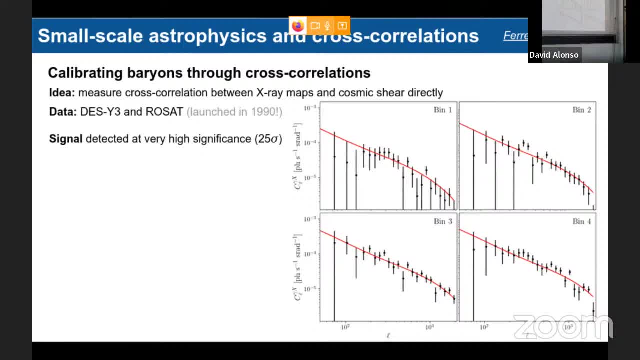 pins. so you, you know we pick up the, the, the cross correlation of really high significance. it's totalized 25 sigma, so it's actually comparable with the significant significance of the cosmic shear alpha correlation itself. um and uh, yeah, so this is the measurement, uh, so it's in principle. you could do really accurate science with these kinds of measurements. 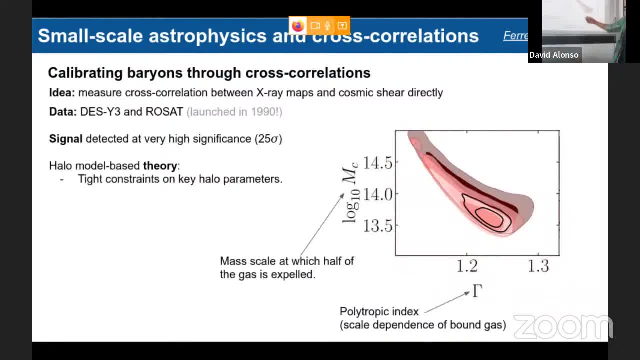 um, what we did is, uh, we used a, a halo halo model based theory, theoretical prediction, which might be not completely accurate, and this is something that we we probably want to work more on in the in the future, but it, um, uh it follows very closely the, the model that was used in in one of the papers that that uh tillman led um. 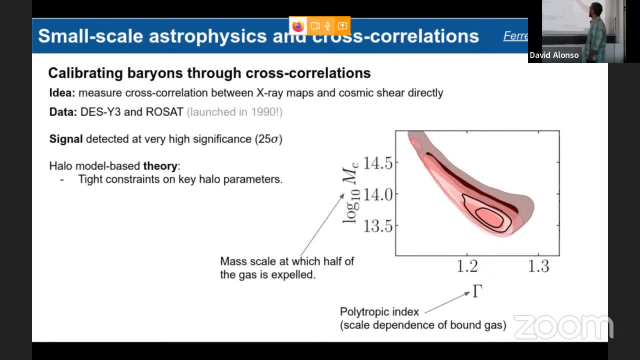 what we saw is that this, this data, is particularly good at constraining these two parameters. so there's four parameters in the model. there's mc, which is the halo mass at which half of the gas has been blown away by. again, the polytropic index of the of that gas, uh, which tells you about the. 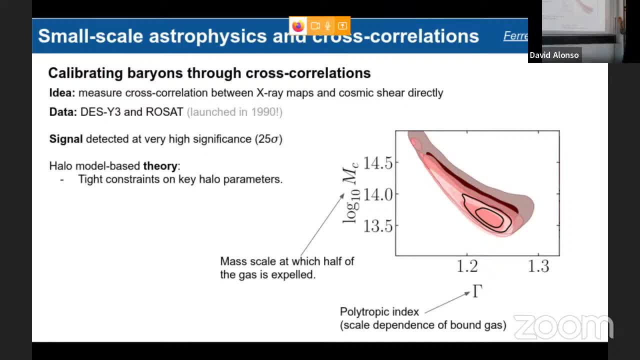 abundance of the bound component of the gas, um, a parameter that uh, that tells you how puffed out the uh, the ejected gas is, and a parameter that gives you information about the departure from the virial temperature in the in the bunker, so something that tells you about temperature and 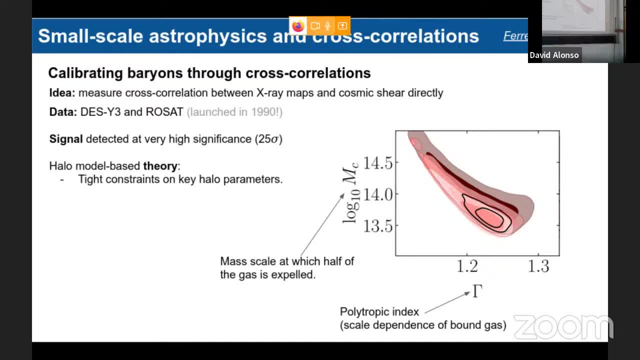 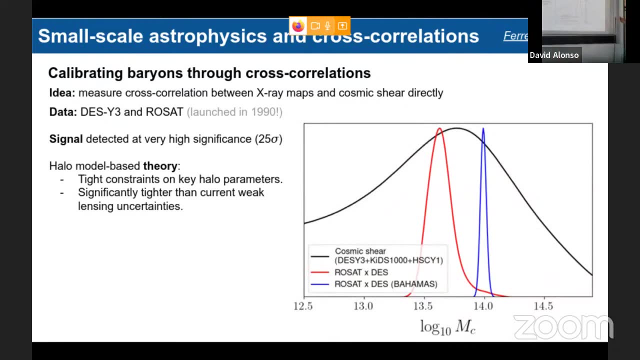 about the popping out of the of the ejected component uh. it turns out that you can get marginalizing overall votes. you can still get very tight constraints on mc and gamma and actually this is rather important because right now the the main kind of parameter that determines how much bionic um uh suppression there is in the matter part spectrum. 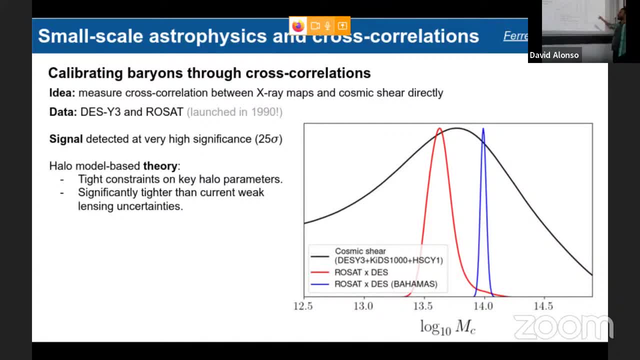 is actually mc. so if you can constrain that, quite well, uh, in principle, you can tell to a good, a good amount, uh, how much um our, our suppression there is on on small scales. um, so these are, for example, the constraints we get from from our data. this is the what i showed before. this is a 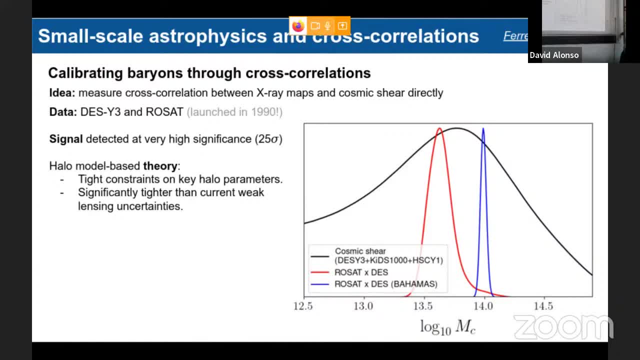 but i can explain what the blue is if you want uh. but just look at the red compared to the constraints you would get if you just had the cosmic shear data to try to self-calibrate the bionic uh, the parameter. so so you know this type of preparation in principle can tell you almost. 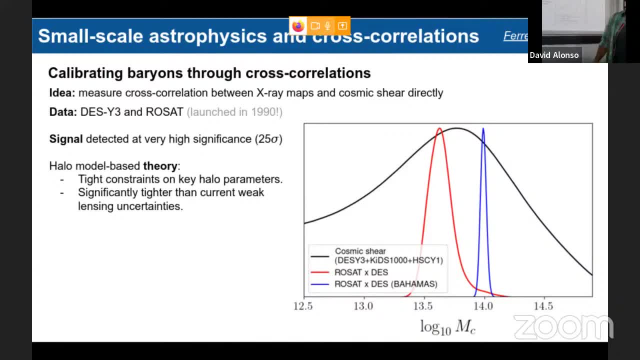 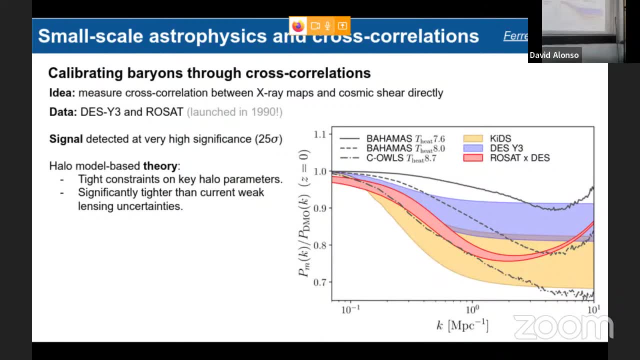 exactly how how much um bionic suppression you should, you should expect um. so if we propagated that to the plot i showed before of the bionic suppression uh factor, this would be the kind of bounce that you would get from from this. um, i would take this with a pinch of salt, mostly as an 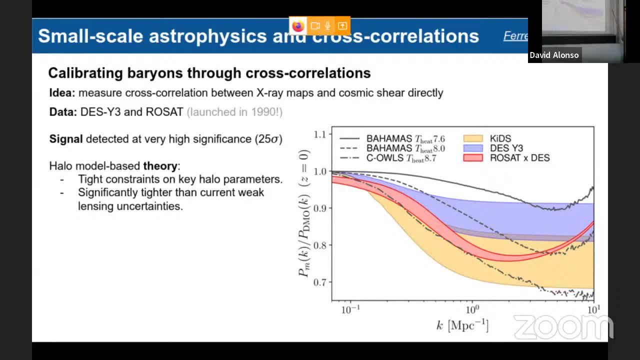 indication of how powerful these type of correlations can be, and the pinch of salt is that this relies completely on a halo model that we, uh, probably want to want to be more careful to, to calibrate with, with hyper simulations, etc. before we can actually fold this into a full cosmological 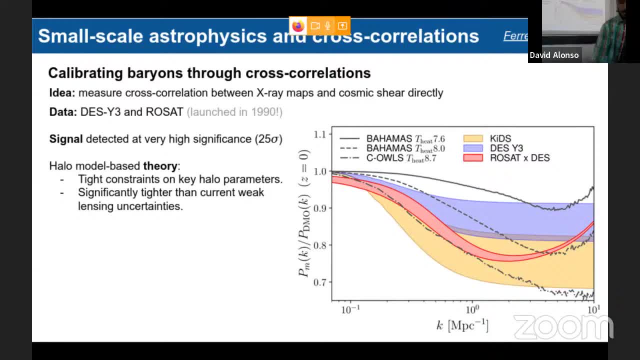 analysis, and that's it. i think yeah, um, uh, so for sorry, uh, no, um, so future, uh, future improvements on this. besides trying to improve the, the model will be combining with with tfz data. so i would be quite excited to do that, because it um would allow you to break the. 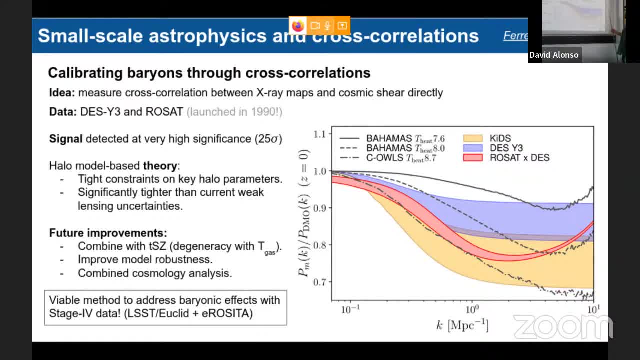 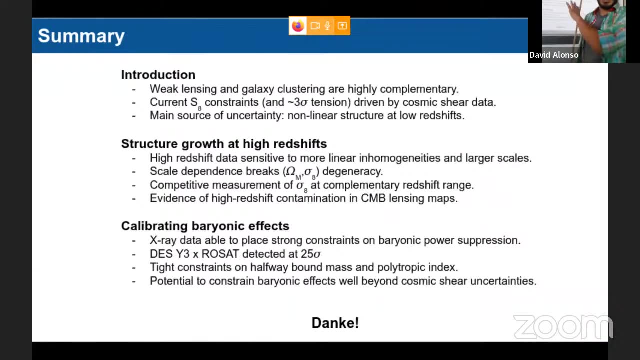 generacies, for example, with the temperature of the gas because of the different weighting, the temperature, uh, and then eventually do a combined cosmological analysis. so what i said before, um, yeah, and yeah, very excited to see if we can actually apply this to to any uh future, future stage four data: um, that's it. i won't go through my summary again, but 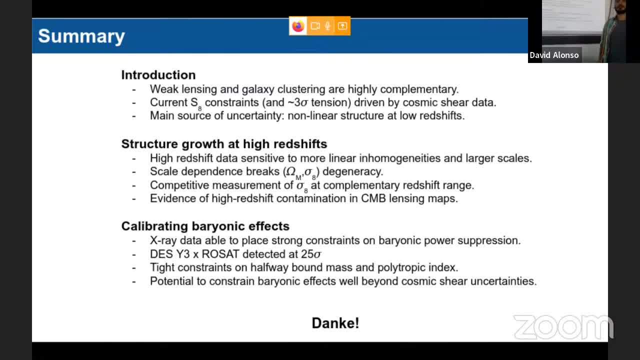 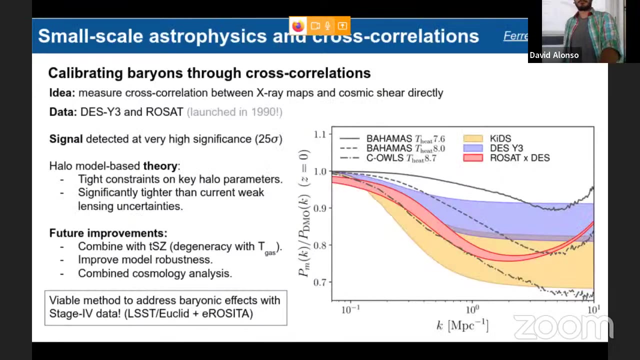 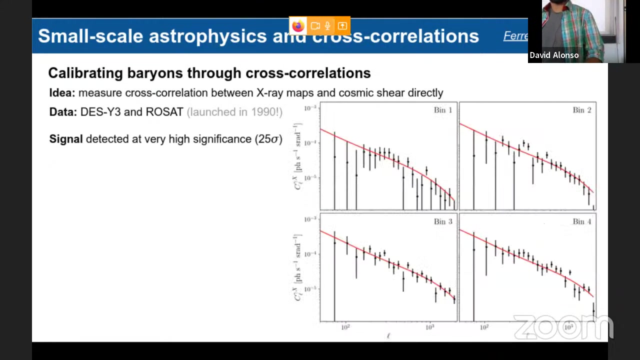 just to reiterate: thank you very much for the invitation and being great. thank you, let's see some questions. we've got some questions. yeah, sorry, we were very busy. going to the last thing you're talking about, did you change the scales? uh, we went a bit uh stupidly- not stupidly, but like boldly, i would say so we, we actually used all the 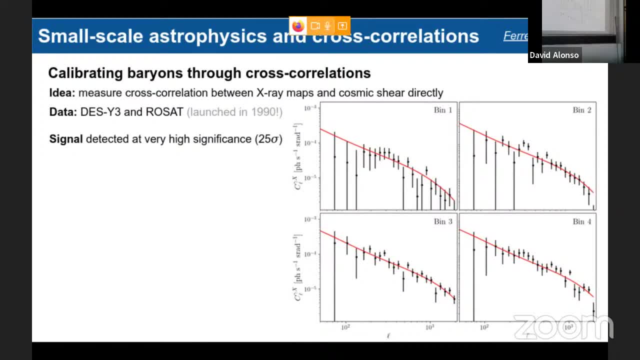 all the, the scales down to l of 2000. right, we're not trying to do cosmology here, but actually try to figure out what's going on on small scale. so we went all the way to where we know bionic effects should be: um, um should be relevant to some extent, right? so so, um, it's not the kind of scales that. 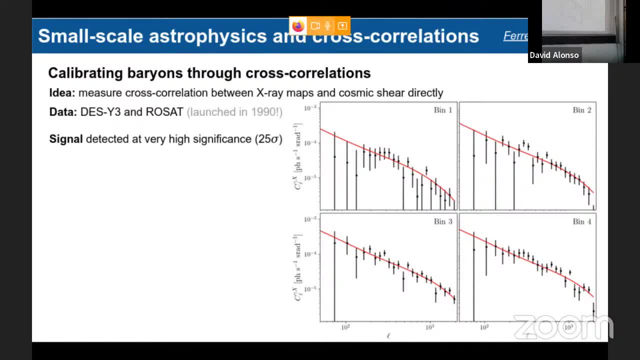 necessarily one would use in a in a sheer, sheer analysis, because you know you would be a bit more sensitive to, but in this case we actually tried trying to pick up the parameter section. so there's a paper led by carlos giovanni is also involved where we're looking. 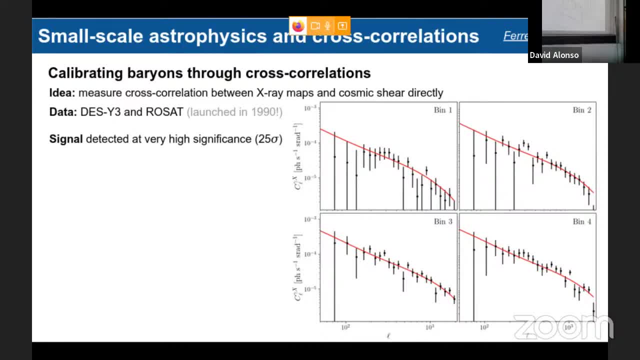 at actually looking on on very small scales, um, uh, whether we, we, we pick up any any relevant uh firing effects using using the, the backhoe emulator that joanna has worked on that hopefully will be out in a few weeks, but uh, but yeah, so in this case we, we went to relatively small. 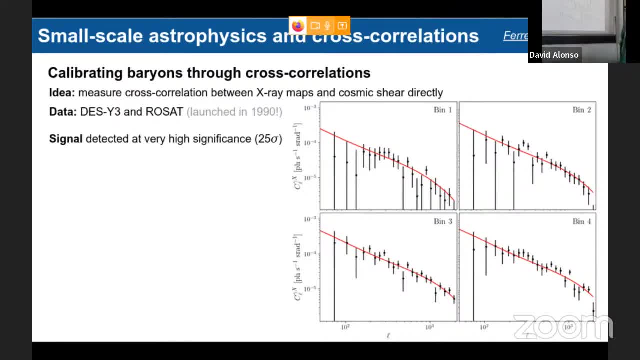 actually holding up. so you're fixing cosmology there, right? yes, yes, we're fixing cosmology to black, that's right? yes, yeah, but and using ds for new shear, which is intentionally, which is in tension with plank. so so this um not not necessarily right in the sense that we're not trying to do cosmology with this. we're. 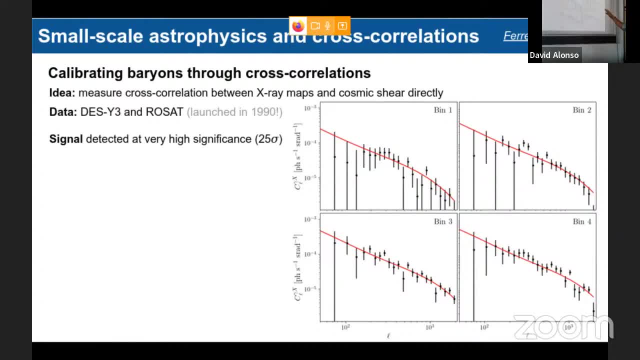 just saying let's assume that something wrong is going on in ds and maybe in the treatment of ironic effects or whatever. let's say we, we trust the most robust and and precise constraints we currently have on cosmology, right? what would this type of correlation tell you about? about? 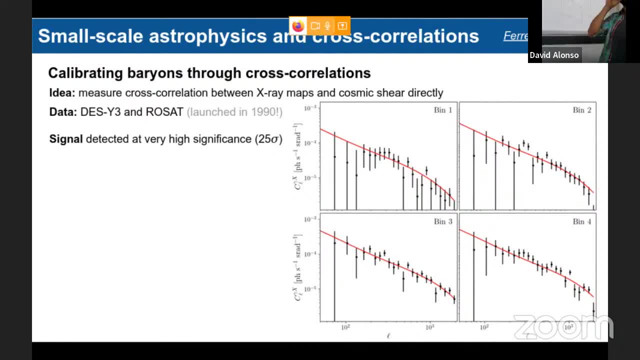 just for the baryonic constraints, i would say i would expect the baryonic constraints, uh, are correlated with cosmology. yeah, like that, but blank value, which is intentionally the same. yeah, if you're using, maybe like, yeah, i think so, i think, yeah, i, i agree, i agree, um, we just i don't think we're at the point where we can fold this into a 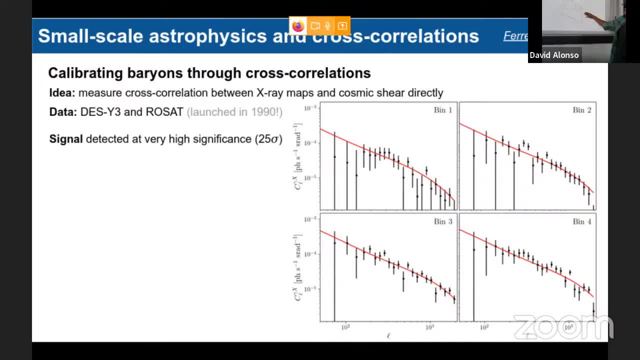 cosmological analysis, because we, the model presides at the kind of 10 to 20 level, but not at the level that we would need it to be for cosmology, right? so yeah, but i, i agree, yeah, yeah, um, you thought about this. let me see at the beginning, and i i forget, what we thought um. 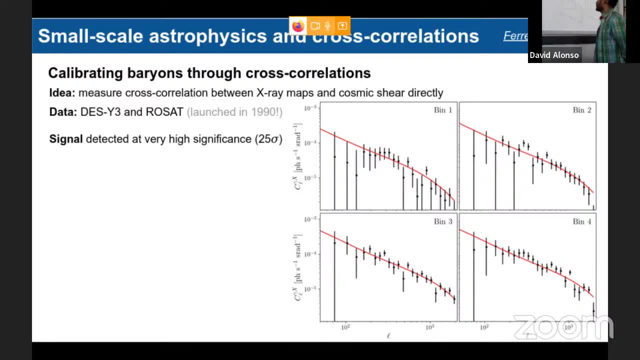 but in principle, yes, uh, in principle yes, and they would affect you in the same way that they affect um cosmological constraints from the x-ray power spectrum, which people have tried to do in the past. um, so yeah, so that that's something to think about as well. i think, um i would imagine that that's gonna affect almost anything that um like tsa. 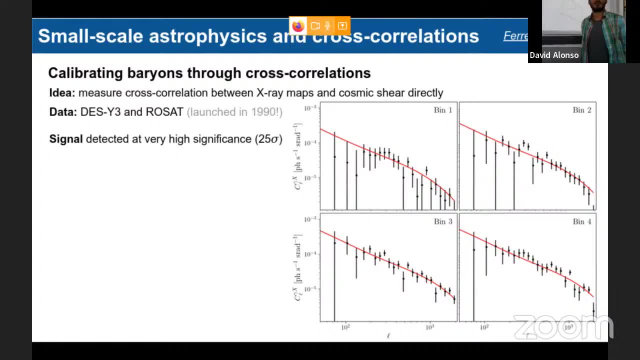 for example, as well, right, um, or maybe not that much, yeah, um. so so yeah, yeah, um, but i would, and i would imagine it would also affect uh, the cluster, like uh, gas fraction measurements, right, and then anything that uses x-ray data. yeah, yeah, um. so no, yes, the answer is. 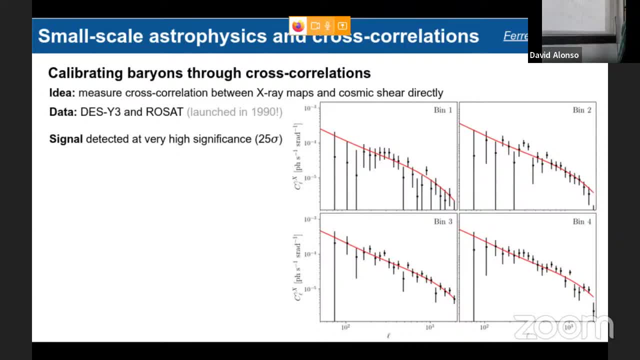 yes, but we didn't. we didn't model that here. yeah, maybe i can ask one: uh, maybe just do about this tension, because we see now, with new real analysis, giovanni and other people- exceptional decreases, this kappa thing, yeah, so where do you? i mean, what do you see? now, if i'm an outsider, should i be worrying about this? is this a real fashion or not? 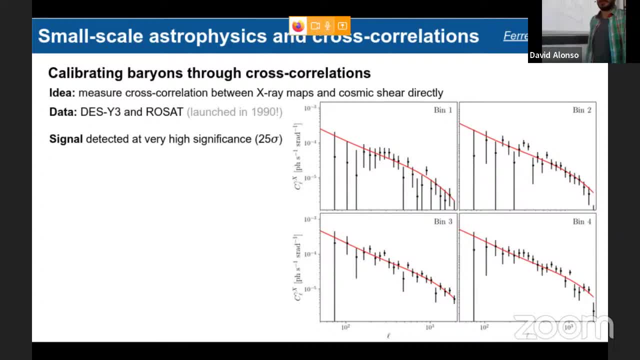 i think we, you know, um, probably you know, we will know better when lsst is around and three sigma becomes seven sigma, or it doesn't. uh, i don't know. i think the fact that you can actually isolate it to a very specific range of red shifts and kind of scales tells me that it's probably something to do with how we're. 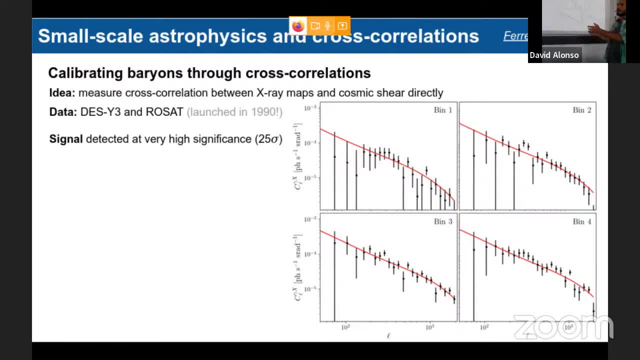 treating those right, um, um, but it's a complicated problem. we we actually need to pull uh as much data as pros uh as we can that actually allows us to um, yeah, to pin down what what's going on on small, particular variant effects and things like that, before we can actually say: because even if 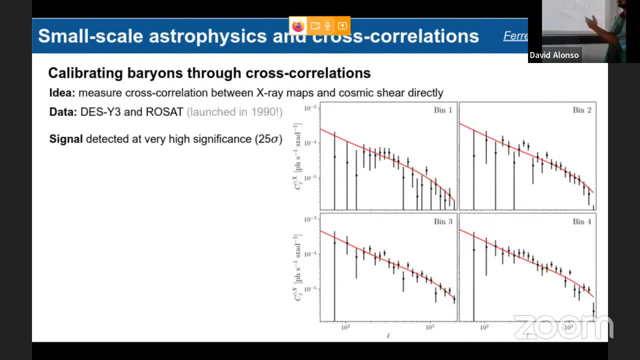 it's on small scales. it could still be new physics right on those small scales, right, so we just need to make sure that we have a good handle on on what, um, what non-new physics things we, we, we need to model better. basically, um, but yeah, i think, yeah, the fact that anything that is higher red chips. 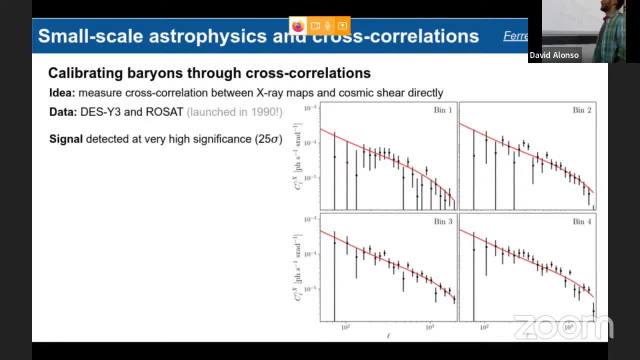 or particularly larger scale, doesn't seem to show up this tension. um tells me, you know that. tells me that whatever it's causing it, it's on the very small scales, which is actually where most of our theoretical uncertainties. so so, then, we need to work on that. 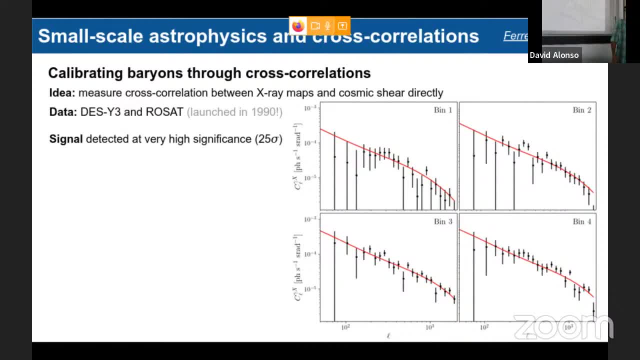 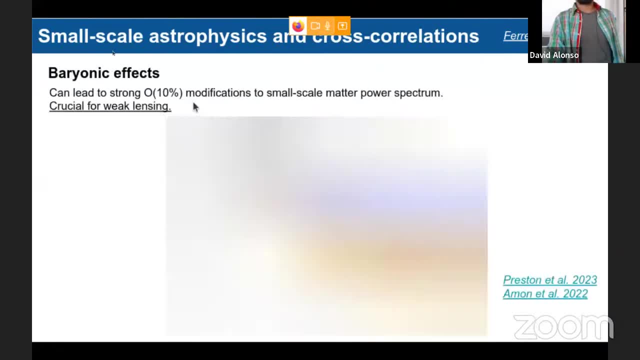 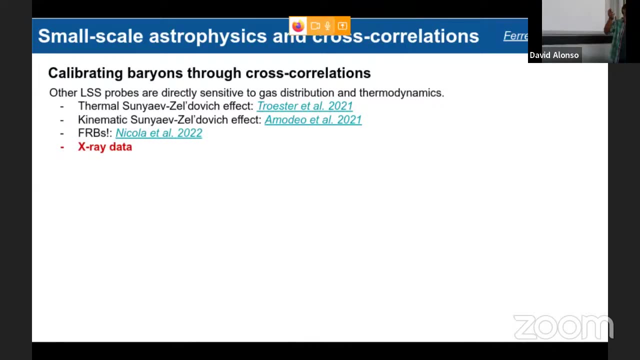 the other. yeah, it's just um, so the ksc has the same. so the um, uh, the thermals and jets of love, each effect has a very um characteristic spectrum as a function of frequency. so it's very easy to separate from the main cmv and any other component in the sky. the ksc has exactly the same spectrum. 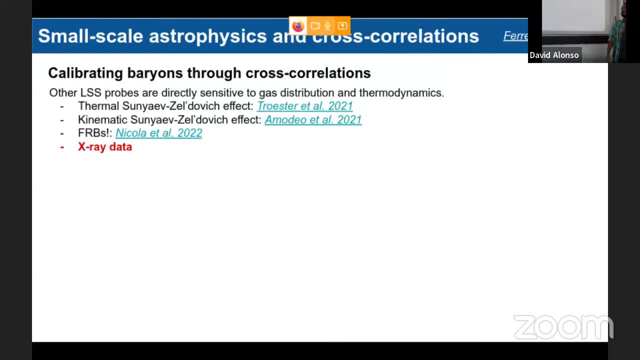 as the cmv. so you can't really use spectral decomposition to pick it up, so you need to rely on its scale dependence to to pick it up. uh, that's the first issue. second issue is that the kinematic sodium knowledge effect is basically the caused by the bulk motion of the of, of um, of the gas. 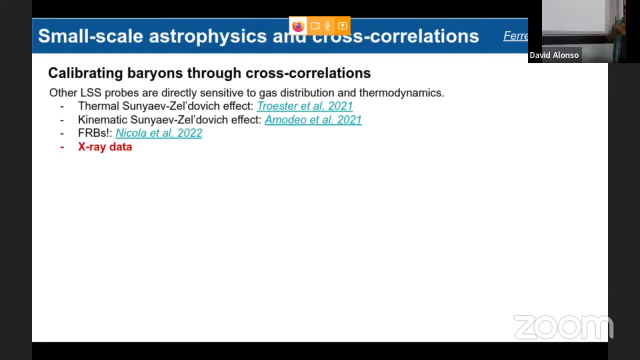 so it's not just sensitive to the density, it's sensitive to the density times, the velocity field, um. which means that if you cross correlate with anything, that cross correlation is always going to be zero, because the velocity can be positive or negative. so that you can show that any cross correlation is is zero, do you need? so you can show that any way. 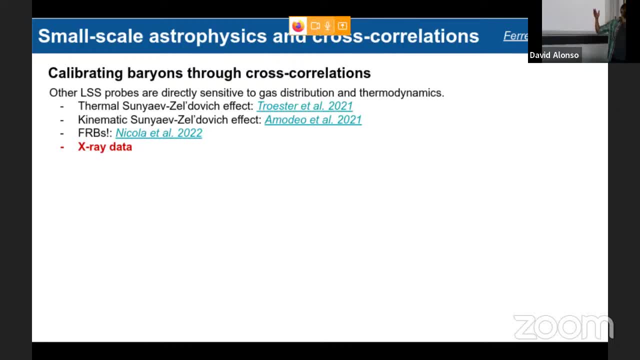 of picking up the. the kse involves higher order correlators one way or another um, so the measurement is very difficult. it's a small effect that is kind of drowned by the cmb noise, so it's only recently that we've been able to detect it to higher than three sigmas um. so the the latest. 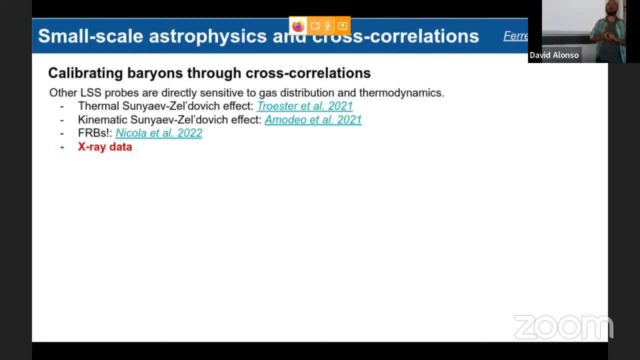 data actually takes it to to a seven sigma right um, and that's where you can actually start doing some some science with it. one potential issue is that, in order to pick up the- because the, the amplitude of the signal is- is quite low- in order to pick up the, 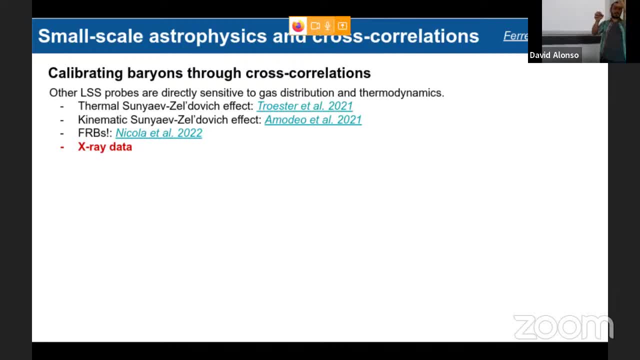 ksc. you need to target, so usually what you do is you would stack maps of the cmb, filtered on specific scales, on the positions of galaxies, um, for example, right with the right weighting. so you correct for the sign of the velocity, for example um, but you will only be able to pick up the effect. 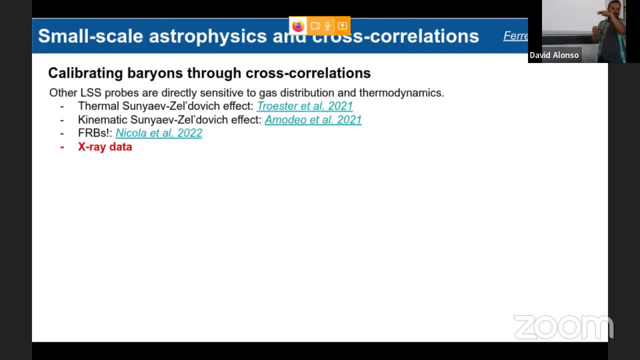 if the, if the ksa itself is sufficiently strong, right? so very often you're kind of limited to masses of 10, to the 13, to 10 to the 14 solar masses, in order to pick it up from the noise. um, so this, this, this problem.